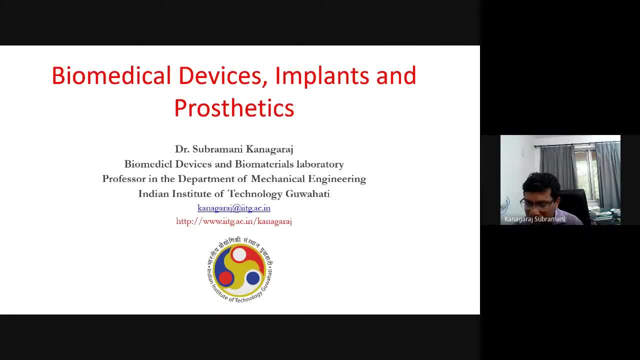 Okay, thank you. Good evening to one and all. Okay, I'm Kanagraj here from the Department of Mechanical Engineering at IIT Guwahati And I'll be briefly giving information or that work, what we have been doing at IIT Guwahati in the domain of biomedical device implants and the prosthetics. 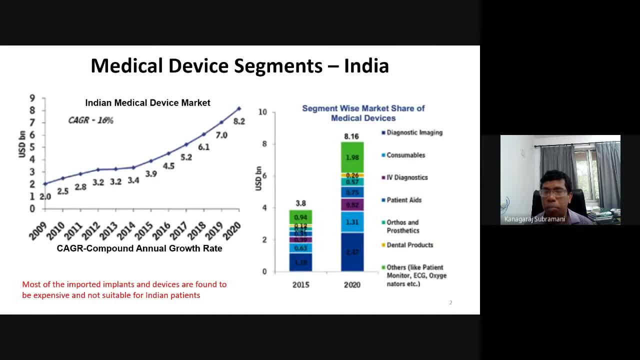 Okay, so this is just one slide, is brief introduction about it. This is what, what is our requirement. So this is what. in 2018, AMTJ, they made one conference and in this one, they have made a summary of summary of our medical device requirement: how much we are importing and how much we are manufacturing- even in a manufacturing domain also- are importing. also, what are the different segments where we need it? Okay, And mostly, if we talk about it, this: for diagnostic imaging, this is out of 8.1% of the 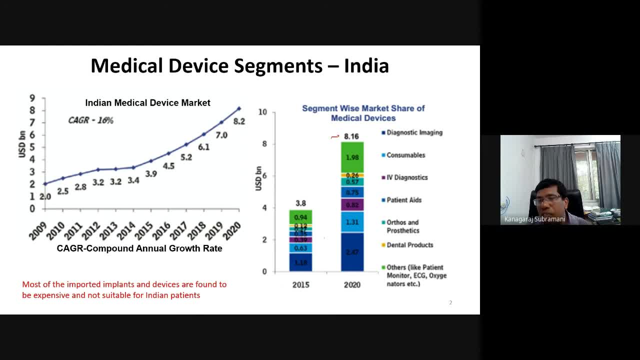 $1.6 million- sorry, a billion dollars. this one we are targeting about a 2.5. diagnostic images consumables- even medical consumables, also part of it- are being imported. Okay, so like that, and our requirement is- you can see here what you can come on: annual growth rate of about a 16% each year. Okay, so that is what the initial growth was. starting in 2009 starts with a $2 billion and at 20, it is 8.2.. And if 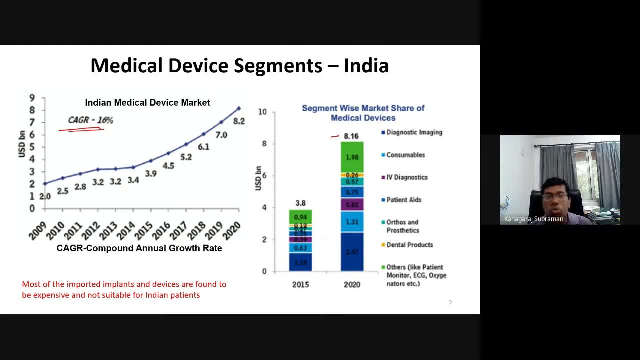 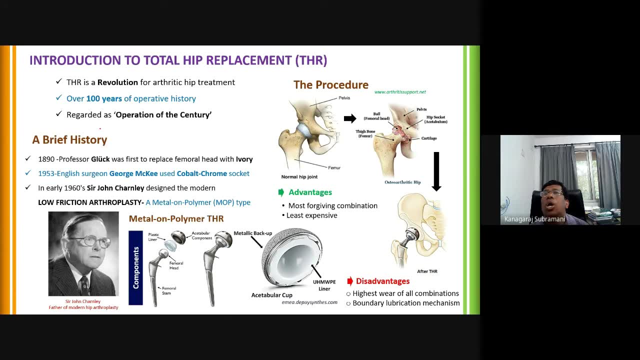 is keep on increasing, and we are. we have been using it also. okay, that first part. what i will be talking about is astabular liner. okay, which is made of medical grade polyethylene. it is ultra high molecule polyethylene, and before that, if you talk about that history, it is start to more than 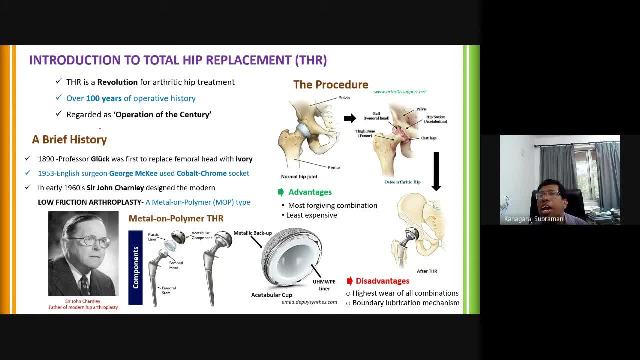 100 years old- more than that. they have been doing a different kind of surgery, starting with ivory ball and different materials they have been started to use and each time, whenever the patient is having some kind of problem, they will come and they will try to modify. so in this. 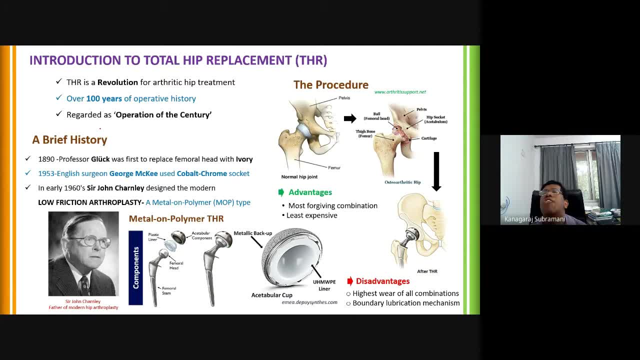 generation they will be talking about. they have been making a different kind of a bearing combinations, starting with the metal and metal, metal and polymer, ceramic on polymer and ceramic on ceramic, like that. so this is what, what you can say in a normal joint, normal hip joints. you will. 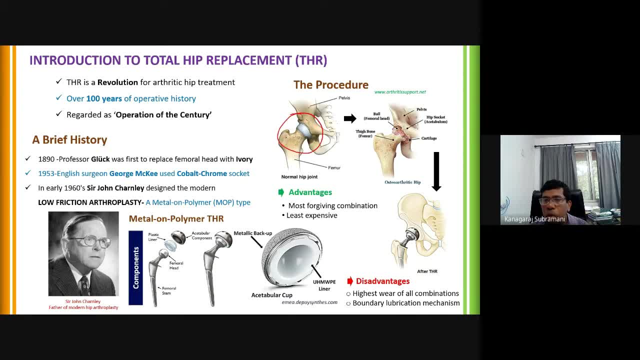 see here. only, this is what an appellate's bone and this is a femur as a femoral stem. here this is a femur and here you will be having a stabler liner, here and this is a femoral head. and this what we are working is: it is a replacement for a stabler liner. what is kept in the pelvis and here, once the person 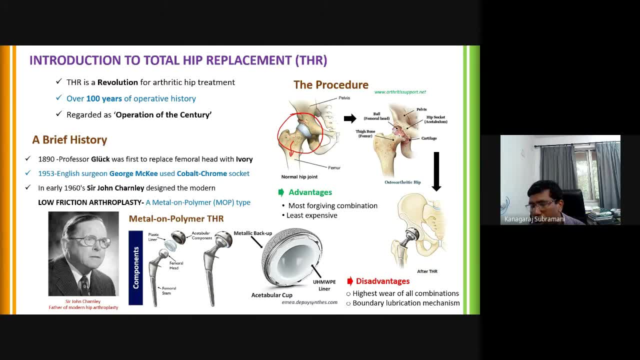 is having a some kind of a problem. anyhow, most of you are from a medical domain, so you will be aware of that. just i am giving a brief information about it. so this is age-old problem, that osteoarthritis. if it is coming, then uh, there will be a, or you can say that cartilage tissue will be damaged and it leading. 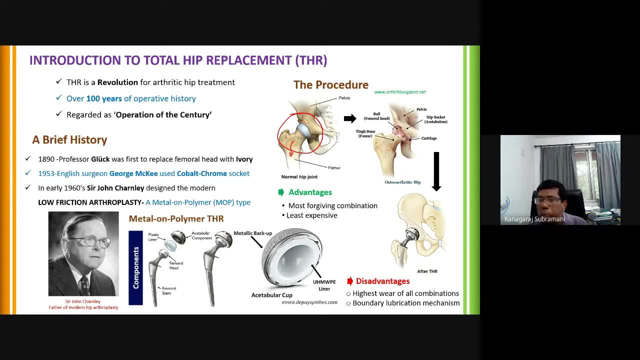 to bone to bone conduct, then there will be a lot of the pain. the patient cannot walk or the person cannot walk. so in order to have a uh, in order to bring back the work lifestyle of the particular person, then this entire part, that established part, will be replaced with this: 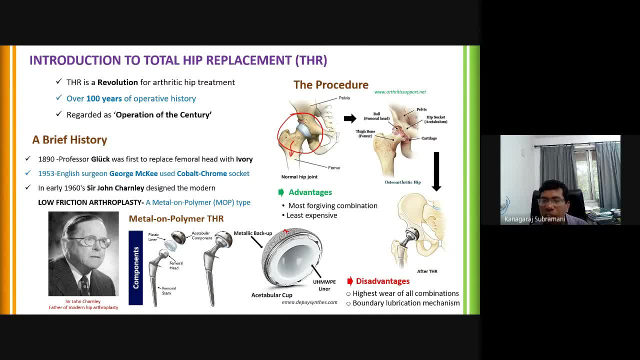 okay, this is what the metallic pack up will be: be fixed in the pelvis and this is what that astabular liner and of ultra high market polyethylene. this is where that femoral head will be moving around. it will be having a three different three. 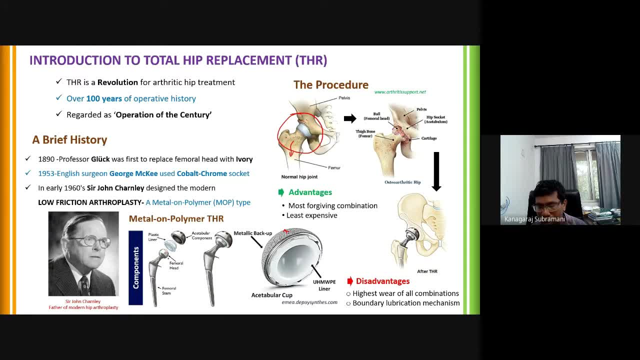 degrees of friction, uh, three degree of freedom, starting with flexion. so flexion extension, then abduction, adduction, as well as the rotation, along with the dynamic loading condition. okay, he was. he is dr john chonley. he started around the 1960s. he started to develop this metal on polymer. 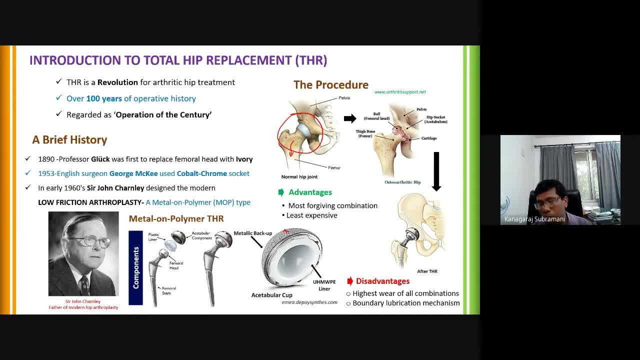 total hip replacement with a bone bone cement. okay, so that is what he started, and after that, in a metal day, different kind of metal, starting with the cobalt, chromium, ultramalloy and other things, are being used, and though it is being used from 1960s onwards, 60 plus, but that number of 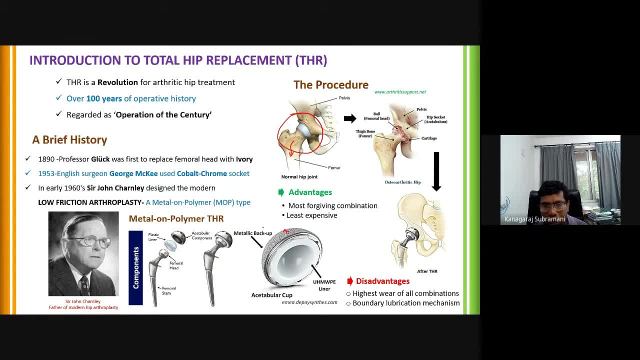 wear. debris generation from the astabular cup is the major issue here. okay, that's what. initially they started with the pure polymer, then after that cross-linking polymer, highly cross-linked polymer, then alpha, overall dispersed to polymer and all. there are different stages of it. okay, still it is being used and that's what it is. okay now, before. 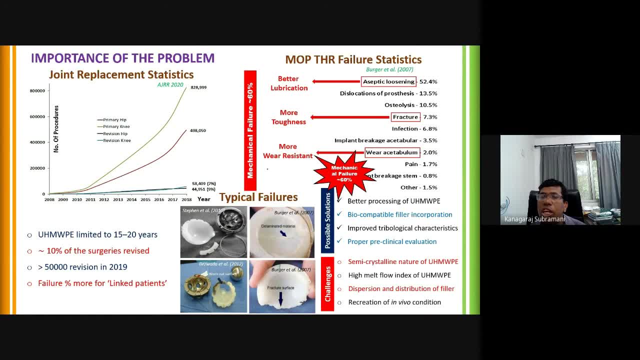 we go into that, that, what we have been working, these are that a major issue. even though this is being used, it has a lot of issues. there are many studies on the retrieved implants you can see here. instead being a polymer, it is getting broken like a brittle failure kind of it here. 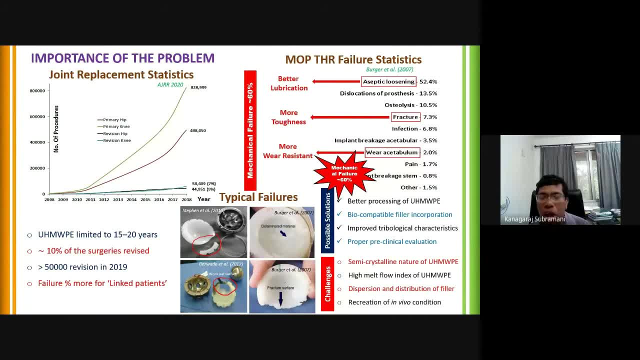 due to the. it is a totally, it is a burning out or it is a fractured in two pieces, or delamination and all like that. and these are the possible failures, what is reported in the literature and if you see the reason for it, that a major part of it near about 52 percentage of the problem. 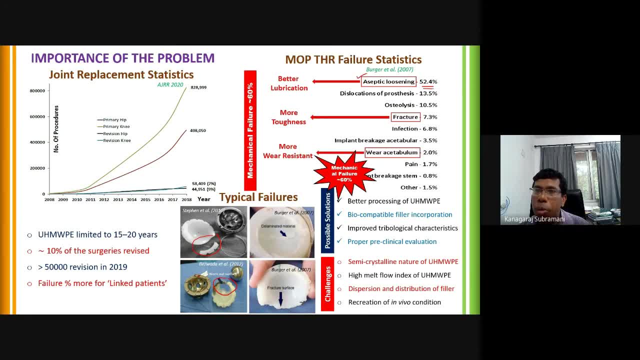 is mainly due to that septic loosening. it could be provided if the implant is having a better lubrication- okay, because in this one, in a normal case, it is having a better lubrication. once that total hip replacement is done, then the lubrication in the bearing condition, bearing media, is lost. 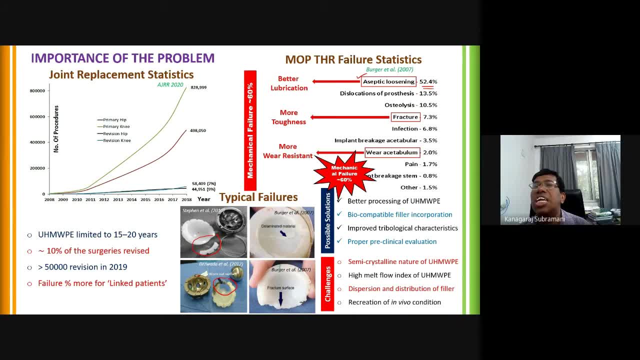 so if you could provide the better lubrication that excess heat generation between the bearing surface will be reduced. then cascading effect could be reduced. that that is the reason for the aseptic loosening. then another one: failure, fracture of the implant, and it is about a 7.3 percentage. it is if you increase that toughness of the material. 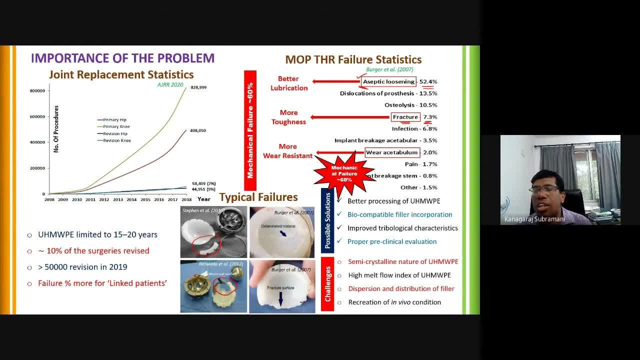 okay, another way, make a simple way. if you want to say that area under the stressor strain curve, if you wanted to area under that stress versus strain curve, if it is getting improved, then we can reduce that wear volume generated. okay, that wear volume is inversely proportional to the 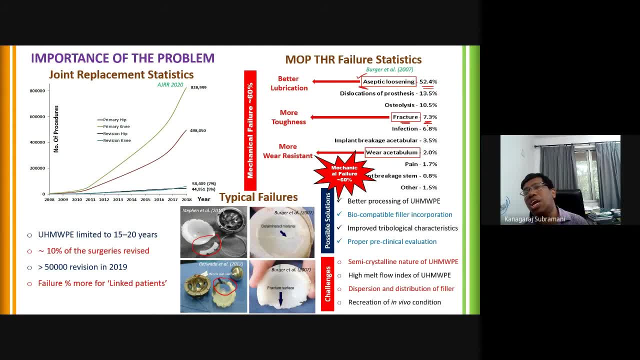 toughness. so if you want to reduce that wear volume, then you can reduce that wear volume. okay, that wear volume is inversely proportional to the toughness. so if you increase the toughness, wear volume could be reduced. in addition, that fracture also will be reduced and after that that we are of the um. it is about a two percentage. so if you add all those, 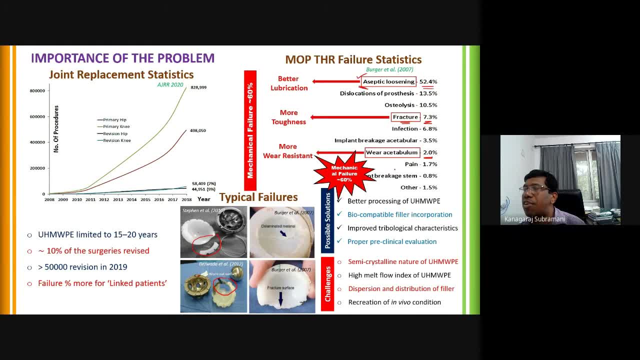 things. this also it is a surface phenomena. if we increase that surface resistance, wear resistance, if we increase it, then we can reduce the problem. so out of at near about 100 percentage if you talk about it, nearly 60 percentage of the revised surgery of the primary implant, because primary 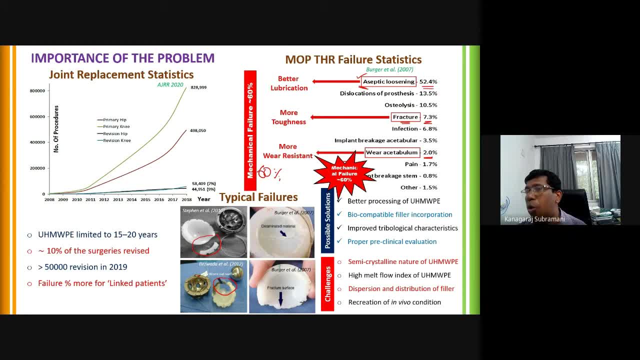 implant primary surgery, we cannot do anything okay. so once it is done, near about a 10 percentage of the surgery in a 10 years back, whatever it is done it will be. i had to keep on adding one percentage here in a year, so at 10 after 10 years it will be 10 percentage of the total surgeries. 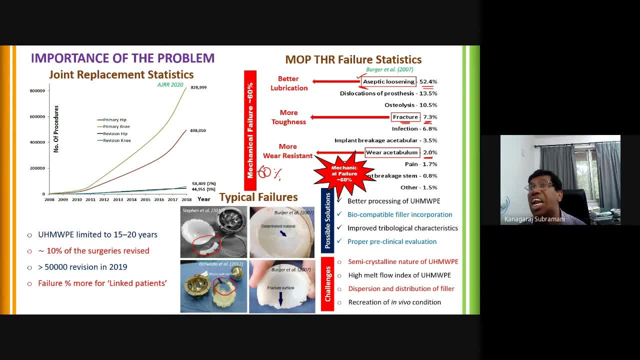 are getting revised because of the mechanical failure or material related issues. if we could work on that material related issues- we can reduce that number of replacement surgeries. okay, so what we have proposed, this is what, uh, what you can say- primary and uh, near about, uh, what you can say. this was the primary hip surgery, near about a, near about 5 lakh and a primary knee. 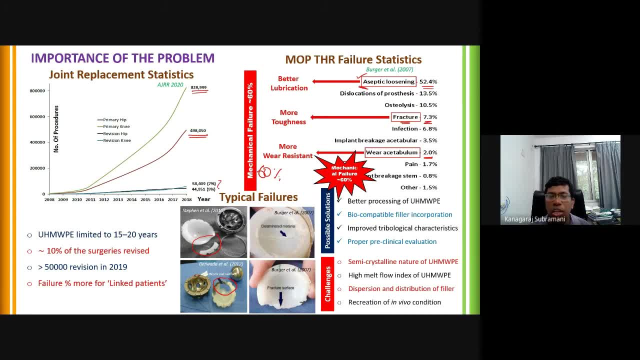 replacement is about 8.3 lakh and this is what that replacement surgery is and out of that, 60 percentage of the surgeries are revised only due to the material related problem. okay, and if you see the possible solutions and if you could able to do that- better processing of ultra high market polyethylene, or we can have a. 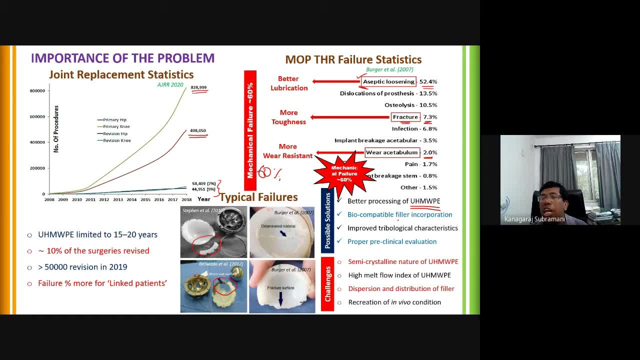 biocompatible filler or the reinforcement if you want to attack, if you are increasing the tribological characteristics of that composite material and in vitro state, a proper in vitro study under simulated condition. if you do, then we can reduce that number of replacements surgery okay. so when you are coming to the challenges, to achieve those possible solutions, because that 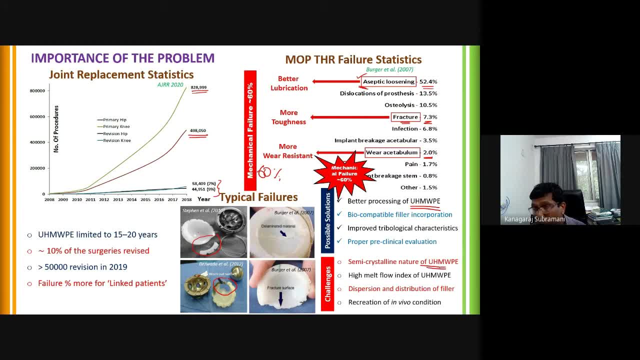 ultra high market polyethylene. because of that, we can reduce the number of replacement surgeries okay. so when you are coming to the challenges to achieve those possible solutions, because that of its high melt flow index, even after reaching the melt point it will behave like a solid- okay, the flowability of the polymer will be totally. it will be less so if you find the 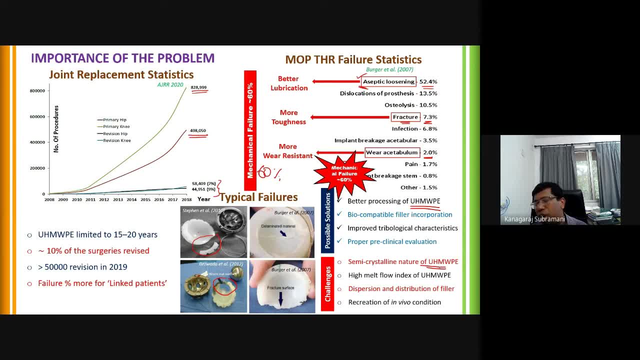 many literature. they will be adding some kind of a plasticizer or somewhat, identity polythene also. they will be adding it, but it is at the cost of the wear resistance of the material. so, without adding any material or without reinforcing it, we need to ensure that how we can improve its. 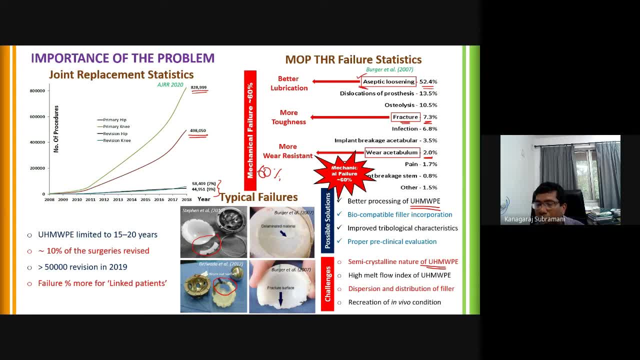 characteristics: okay, only with the processing technique, okay. and if you want to replace, if you wanted to add any reinforcement, then you need to think about how, what could be the optimum concentration and that concentration, how you are going to disperse it in a homogeneously without any. 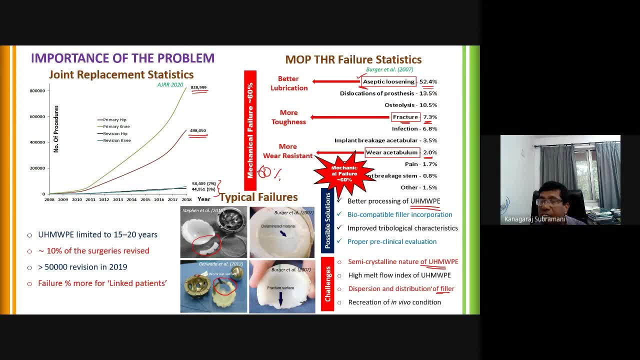 agglomeration. that also we need to see. and after that it is not only the material development, we also need to develop the cup and it needs to be tested as per the iso standard: one four, two, four to one or one four, two, four, two, three. okay, that gives that kinematic profile as well as the kinetic 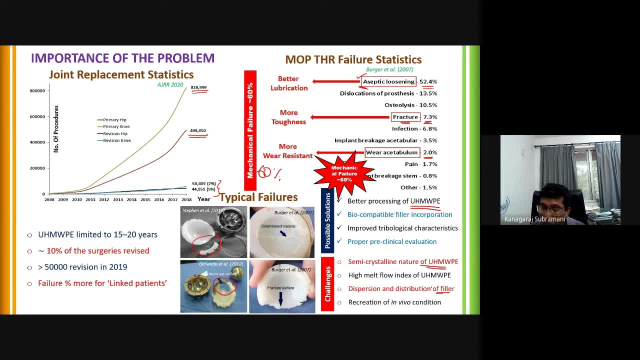 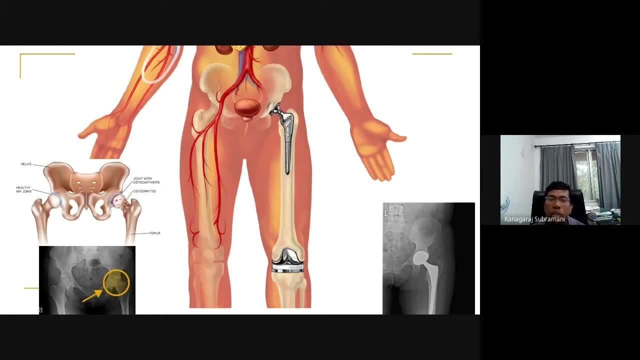 profile of the hip. okay, so we need to do that kind of testing before it could be. uh, it could be thought of testing it in animal and human being. okay, this part: once it is implanted, how it will be looking like. okay, this is in case of a hip replacement. this in case of a knee replacement. 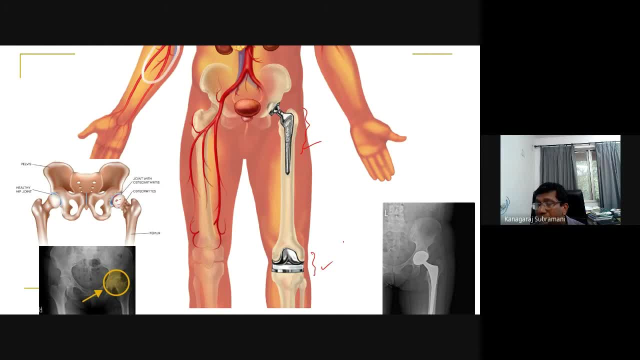 and once this material is developed- and it is a weird- studies are done and the same material can be explored in all kind of a joint replacement: okay, hip joint, knee joint, ankle joint, shoulder joint, all okay. only the geometrically geometrical constraint will be different. rest of the rest of the material, rest the. this material can be used in all kind of. 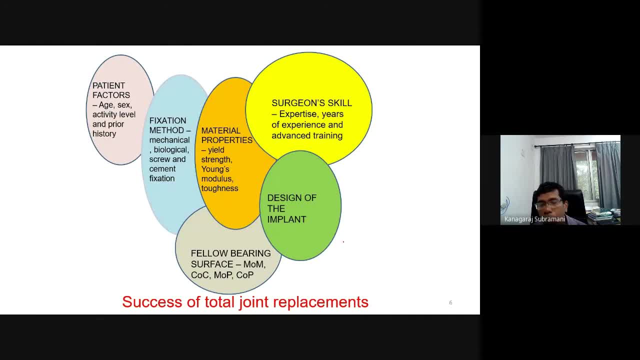 joints. that's what it is okay. so where we are addressing what kind of problem we are addressing it. when you talk about that success of the replacement, success of the total joint replacement, there are many factors and we are mainly focusing on that. i mean engineering aspects only, that is. 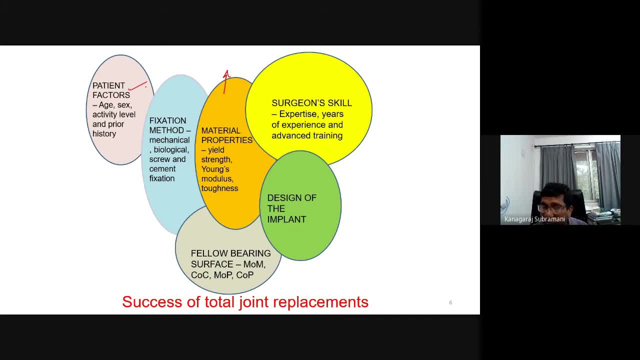 the material properties. okay, so it is a patient related factors. if at all, they are young or elder people about 70 plus or maybe 40 plus. it both are having a lot of significant on the success of the surgery and how it is being fixed, whether it is a cement fixation or cementless. 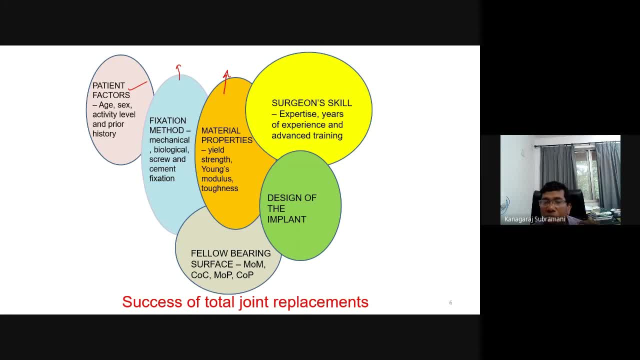 fixation or mechanical fixation, all those things. and when we are talking about a mechanical properties, material properties, what is the yield strength and what is the young smallest? okay, as you know that that modulus of the bone is around the cortical bone is around a 20 gigapascal. 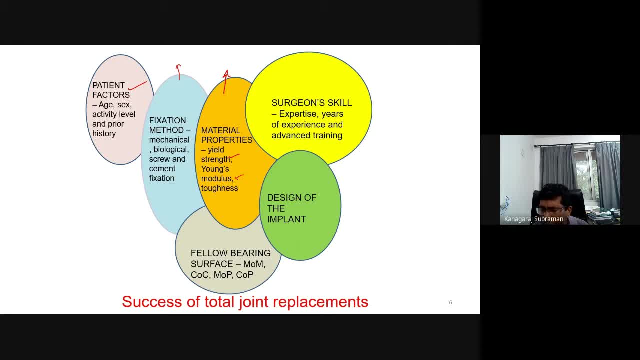 this material will come, we need to bring the material characteristics at par with that. okay then, only there won't be any mismatch in that stress shielding and all it could be avoided. okay then, this fellow bearing, whatever you are using it, whether it is a metal on metal, 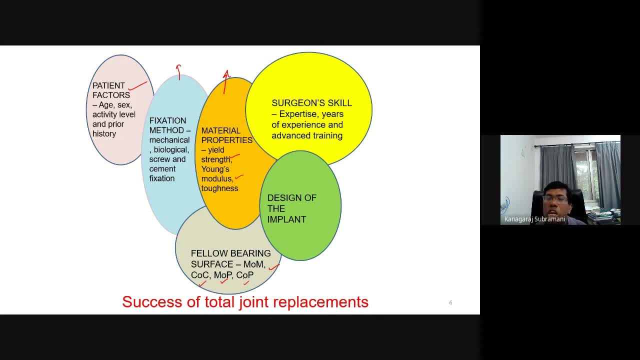 metal and polymer ceramic on ceramic, ceramic on polymer ceramic or any other material, which combination we wanted to use it. so, depending on that, that the debris will be reduced, or debris will have some kind of a cascading effect on the biological tissue, then a design of the implant and finally, the surgeon skills. okay, that is what, how far he got. 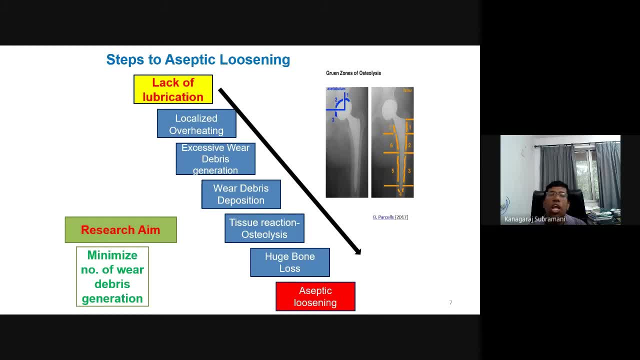 expertise and, uh, you'll find all those things okay. and in case of the replacement surgery, that most of the reason comes in that aseptic loosening- that is, 50 percentage of the replacement surgeries are done and then the replacement surgery will come in that aseptic loosening, that is, 50 percentage of the replacement surgeries are done. 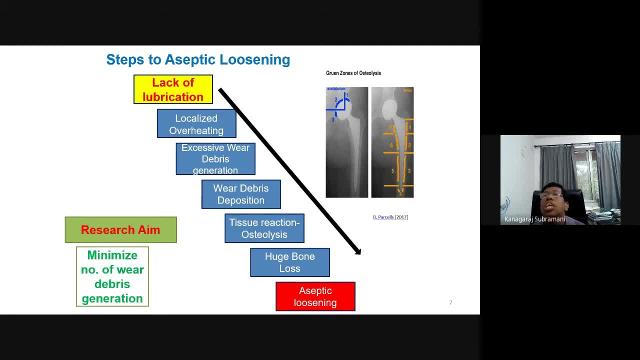 if we could able to provide that proper lubrication in that bearing surface, we can reduce that. okay, this is what lack of lubrication it will be due to that, leading to that localized overheating. then excessive wear, debris if the temperature is more than the softening point. the shape of the cup. 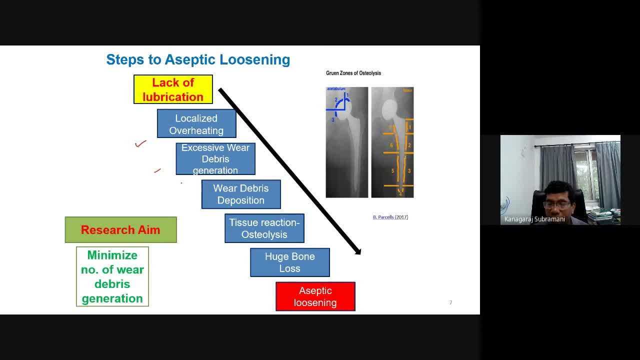 also will be changed, then that will be leading to softening, then wear debris generation and it will be deposited everywhere. then osteolysis will be happening, then bone loss, then it will be leading to that septic loosening of it. so if we could reduce that localized heating and a number of wear debris, 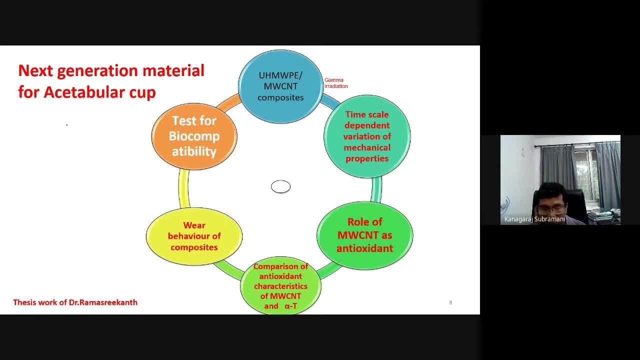 generation, then we can reduce that, we can increase the lifespan of the implant. so in this case, what we are working on it is is that we are working on a uh processing of ultra high market polyethylene and ultra high market polyethylene and it's the cmt composites. okay, so in this one first, we 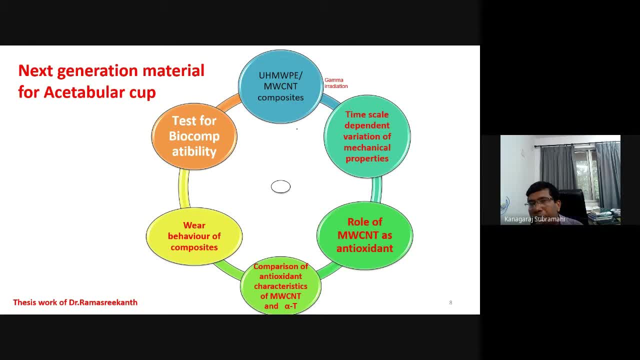 started with a material development and after that, a product, a cup, a stubbler cup development and it's a characterization. okay, that's what we'll be discussing. this is a composite when you are making it, so we need to do all the mechanical characteristics before and after the irradiation once you do that irradiation. 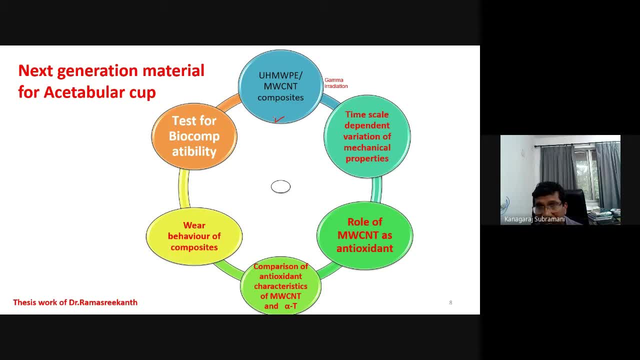 then how long? uh, what you can say. there will be a cross linking and there, in addition, there will be three radicals also. so we need to ensure that the three radicals are to be scavenged in order to reduce that degradation of the material properties. so we need to ensure that the reinforcement 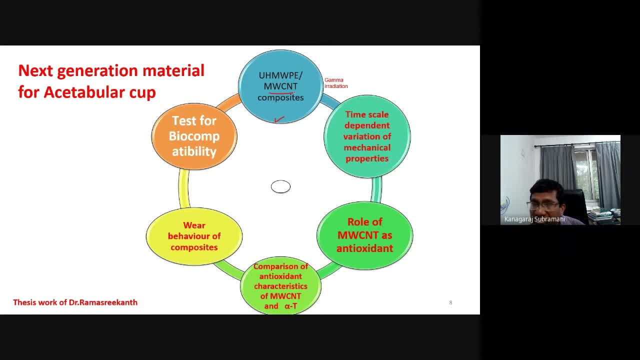 whatever it is being used, it could act as a reinforcing element. in addition, they also scavenge those three radicals, whatever it is getting generated due to the radiation process. okay, that's what initially, if the properties will be good in due course of time, within a three months. 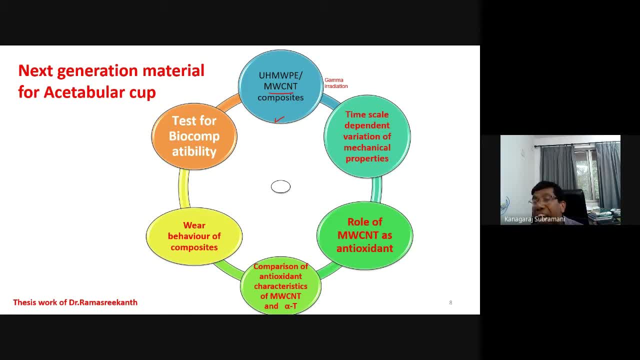 and all like that, the properties will be getting deteriorated due to the radicals generation. okay then, we have confirmed that a cnt with as an antioxidant and we have compared with the antioxidant at par with alpha copper. so, in order to absorb have, in order to absorb those radicals, whatever it is generated. 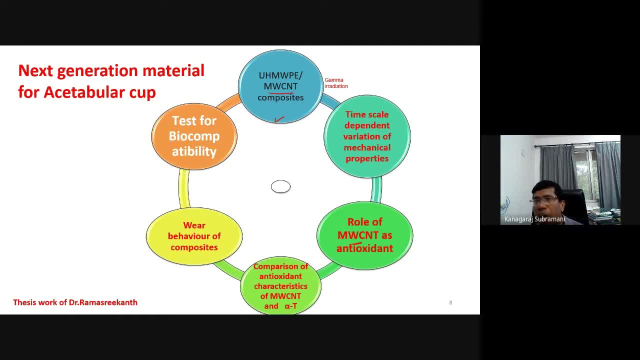 people that fda has approved to use, that alpha temporal and these characteristics are at par with cmt composite as well. then we have characteristics, we are behavior of the material and that test for biocompatibility, as we are adding the reinforcement and in addition, after that we need to go for that in vitro testing as per the iso. 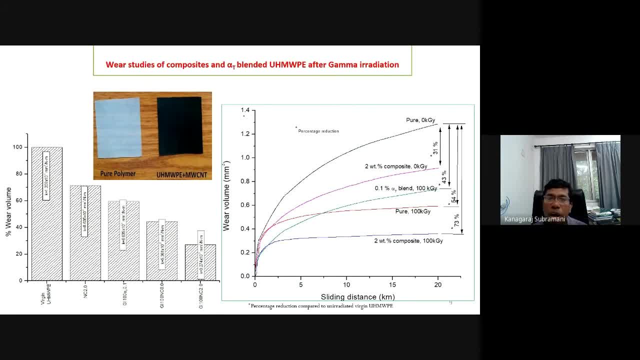 standard. okay, and this is what, uh, what we have developed as cmt composites, and this is a pure polymer cmt composites and alpha t blended composite as well. okay here, alpha to copper oil: we have used about a 0.1 weight percentage, though we have done a parametric study. i am 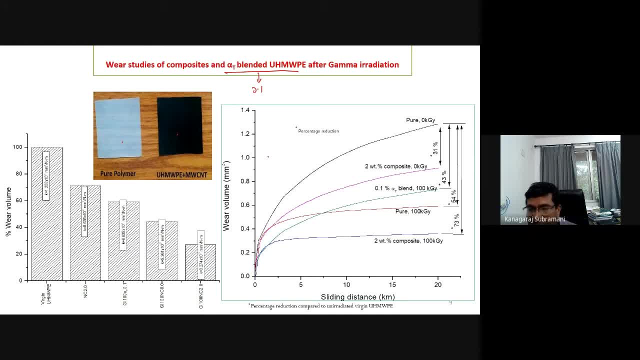 giving just a summary of it. okay, and this study, we did it in a pinon, this machine, okay, and about 20 kilometers sliding distance of 20 kilometers and with this, also with this is with the a stem standard, if i'm writing to 199, okay, and this is what we are volume. when you increasing this is for the 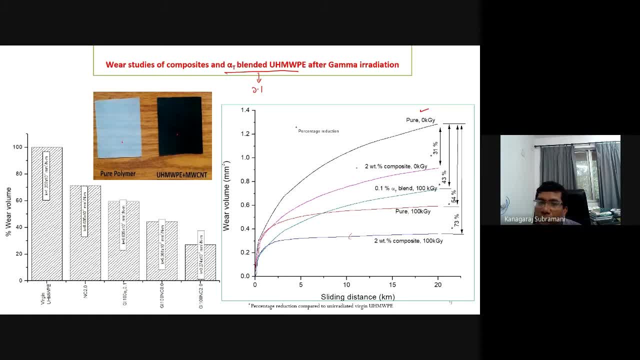 pure polymer, irradiated pure polymer and if you do that, two weight percentage of reinforcement, it is about 40, 60, 40 to 60 nanometer diameter cmt that we have used it and this was chemically treated in order to have a carboxylic functional groups on the polymer. 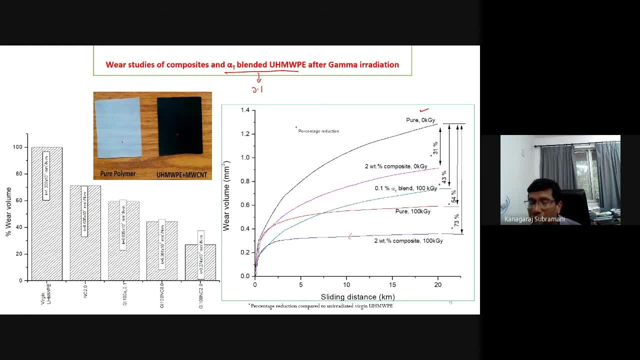 sorry on the cmt. and when you mix it, uh, during that melting process, that carboxylic acid group will be having chemical bonding with the ultra high market polyethylene so that there will be a perfect low transfer between a polymer to the reinforcement. okay, that's what that wear volume. 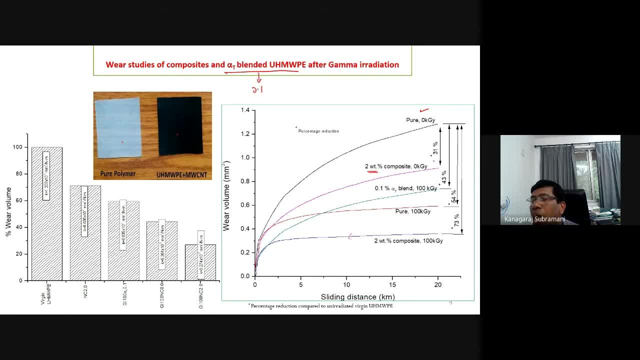 got reduced once you have reinforced it with the two percentage, it is about a 31 percentage- and uh and a, a and this one with alpha t, alpha top overall, with the 0.1 percentage, this one, if you do with the normal uh polymer with only with an alpha top overall blend, there is not much. 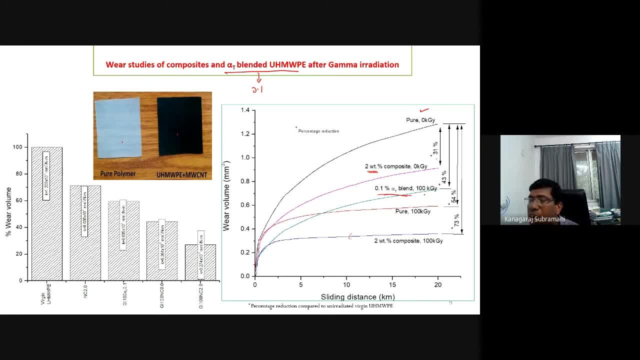 significant difference in any properties. once you do that irradiation, then we could able to ensure that the mechanical properties are getting increased because of the cross linking. okay, and that is the reason. due to that, you have about 43 percentage reduction in a wear volume and pure polymer with. only with the reinforcement, only with uh irradiation: 100, 100 kilo gamma, is it? 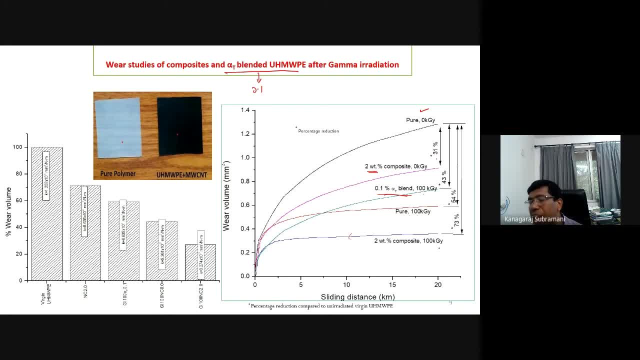 is about 54 and if you do the reinforcement with irradiation we could reduce that rate total wear volume by 73. okay, so by this way we can ensure that the number of wear debris generation in the composites could be reduced drastically. okay, this, what is the pure virgin polymer and composites and 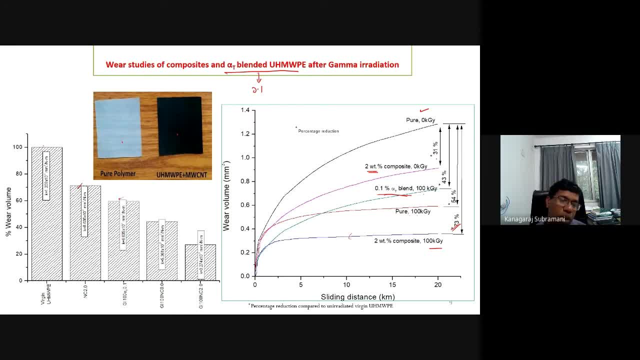 alpha tocopherol 100 kilo gamma rays and with 100 kilo gamma rays simple pure polymer. then after the decomposing we could reduce it. this is for normal test sample in mechanical properties. we did with a dark bone shape and this is what we did. we pin on this, so we'll 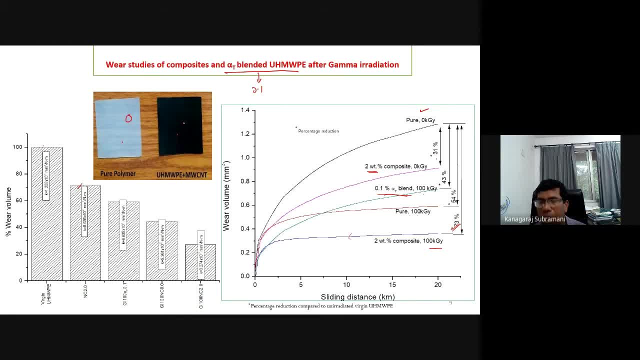 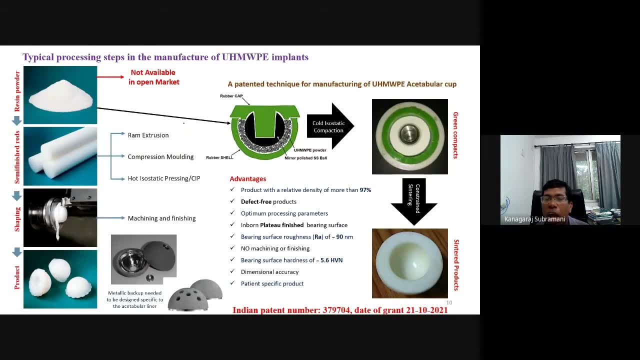 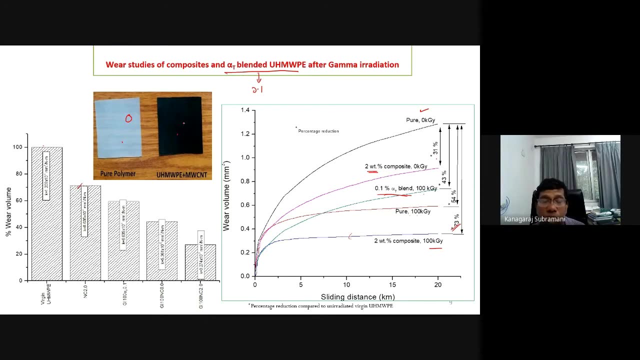 cut a small specimen and we do that testing and all like that. okay, and after getting these properties, we started to make a cup, a stabler cup product. okay, and this also we made. we have started to make this composites from the medical grade polymer with the sample was, the powder was. 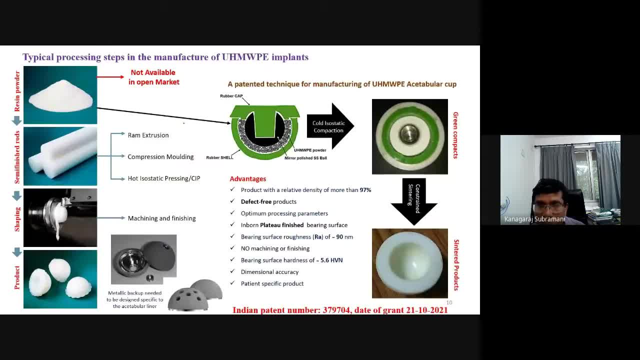 given by the decona. it is a medical grade polymer and with this powder we started to make a stabler cup. okay, and what is being used commercially? right now that they are in gujarat and all like that, they will be having a lot of product and this powder particles- sorry, extruded rod. 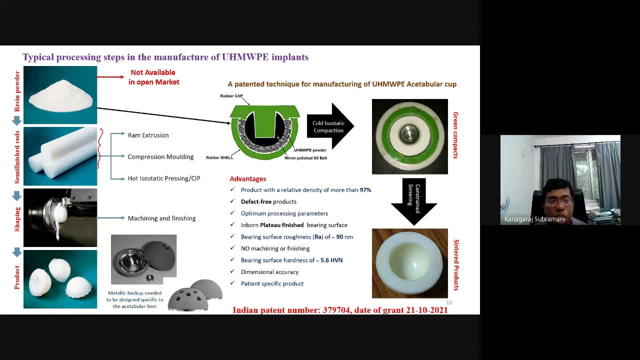 okay, and we are making a cup of this and we are making a cup of this and we are making a cup of that- are getting imported from this rod. they do that machining process with the desired dimension and they will be getting that cup and all like that. okay, and they will be making it will be. 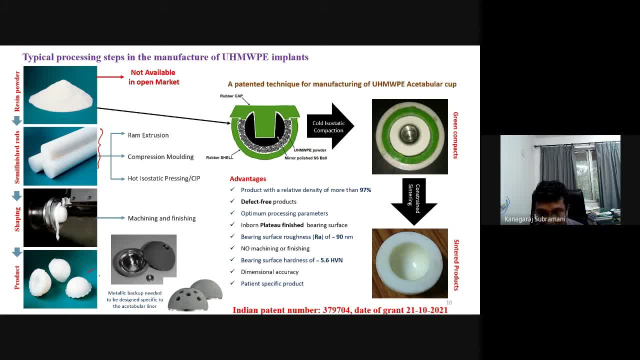 mechanically clamped within the metallic metallic pickup and it will be used in a total hip replacement. what we are proposing is that from the powder we can directly get the product. okay, so whatever the surface finish, you are going to get it in the testabular liner. okay, so that. 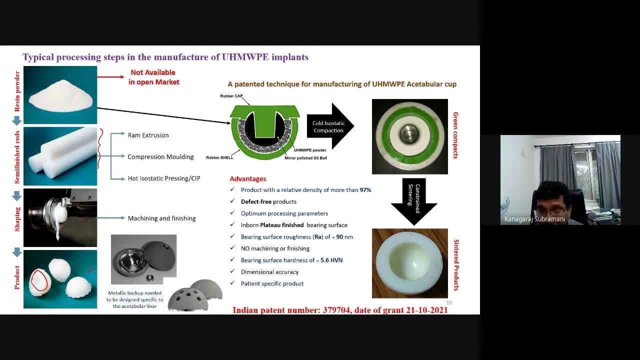 we. we were expected expecting to get without doing any machining process. that is what our novelty in our product when we got our patent. also, it is granted okay. so this from this powder we will have over this is a silicon mold. we will be getting the desired shape and dimension. okay, whatever. 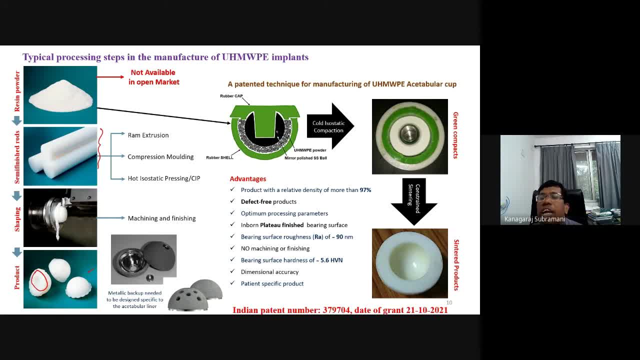 the shape you wanted, we will be having it, and this is what the femoral head. what is commercially medical grade or whatever commercially available surface finish? sorry, whatever the keep, whatever the shape, is going to be okay. and what are the mold? yes, okay, this is what the femoral head. 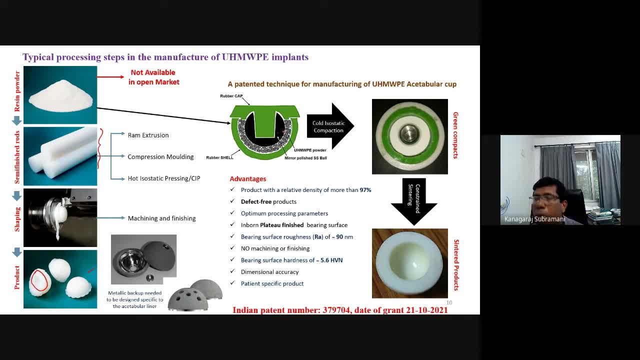 whatever commercially medically, whatever commercially available surface finish: sorry, whatever, whatever. this material will not be used after filling. it is an unisex polymer, so this functional. sorry that that femoral head is available in the market. the same thing has been used. okay, so the same thing. and this assembly was used in a cold isostatic press and you can see that you will be having a 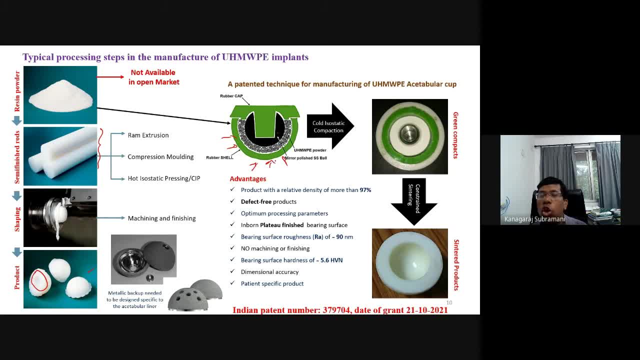 gold compaction and all like that. okay, so you will be having that exact shape and the desired thickness. okay, then, outer periphery: it is, it is anyhow. it is not a bearing surface, we will not bother about it. and that inner surface, only the bearing surface. so here as the ball ceramic, this. 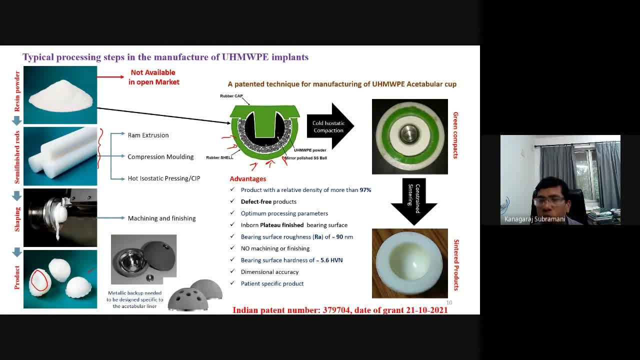 is a cobalt chromium multinolite. this ball is being used generally. what will happen? the ball will be having a surface roughness like that and after cold isostatic press compaction, we did it in a conventional sintering at the same and the ball, what you can say- pressed conditionally. so 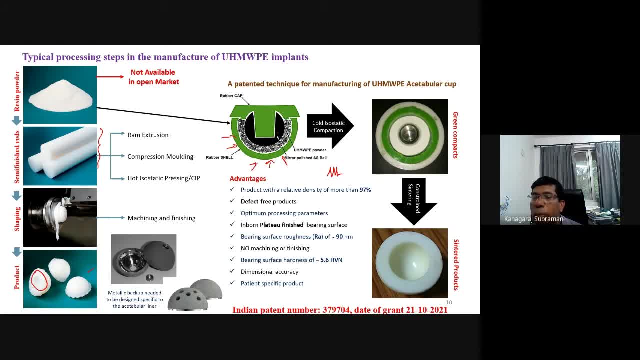 what will happen, as it is a non-pressurized sintering, what will happen wherever that peaks are there? this is what metallic surface finish you can say as to block up, sorry, in the femoral head. okay, so these peaks are getting. if you see that, the peaks are whatever. 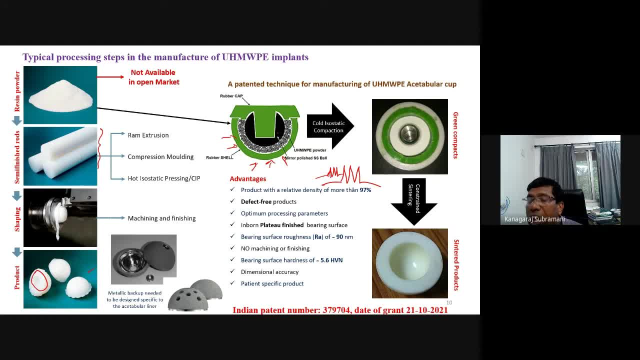 it is there in a femoral head. they are all getting penetrated into the polymer. okay. however, that, as it is a non-pressurized sintering, so this is a. as the polymer is also having my high melt flow index, it is not going to fill into the cavity. okay, so peaks in the polymer surface is restricted. 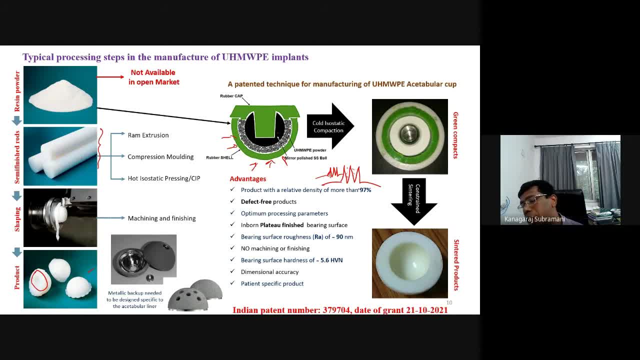 only you will be having the value. so that will be leading to the plateau finish surface just up by the manufacturing process. so by this way we could. the density of the material is about more than 97 percentage and the bearing is about it is a defectory product. okay then, we have optimized. 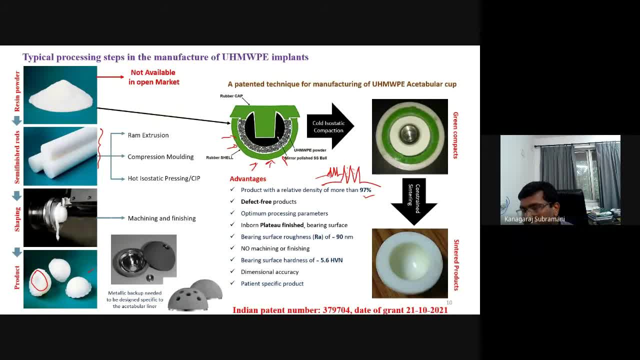 we have optimized the process condition. what is the convection temperature? and what is the convection temperature and the sorry, it is a room temperature, only sintering temperature and the sintering duration. okay, that we have optimized. okay, so we could optimize the properties, optimize that, optimize the processing parameter in order to get 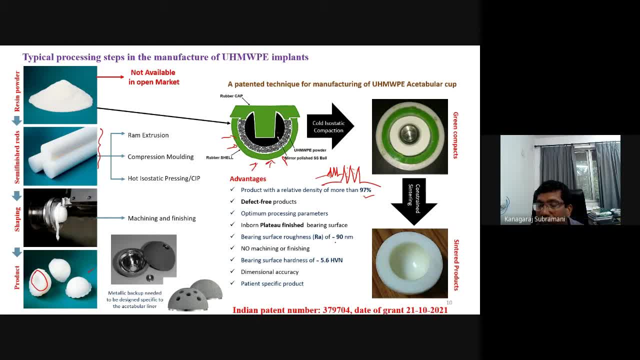 the desired surface finish and all like that. so we could get that surface finish of about 19- 19 nanometer without any misting process, directly. we could get that surface finish okay and that finishing surface surface having the hardness of 5.6, because hardness okay and it dimensional accuracy and all. 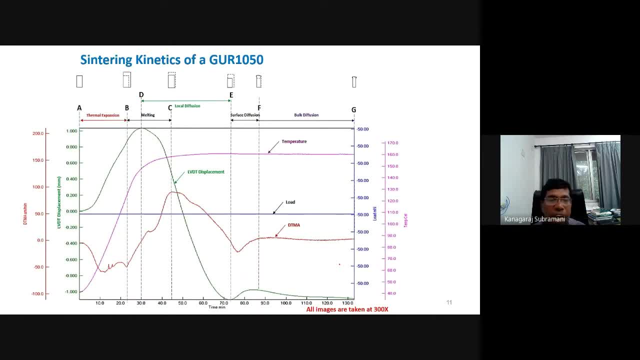 everything we could retain it and this is what the sintering kinetics. we have studied it, okay, and each time you can see here this is at a starting stage. these are the, that polymer powder, and once you start to heat it, you can see they started to. 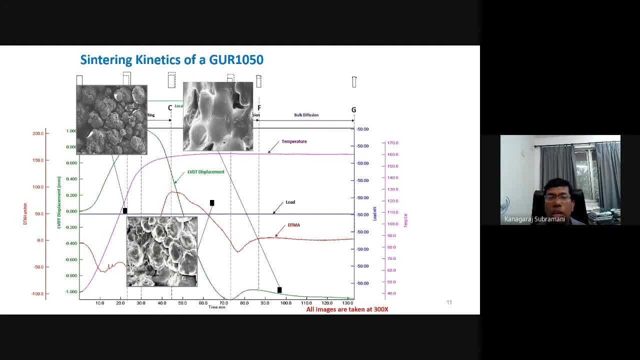 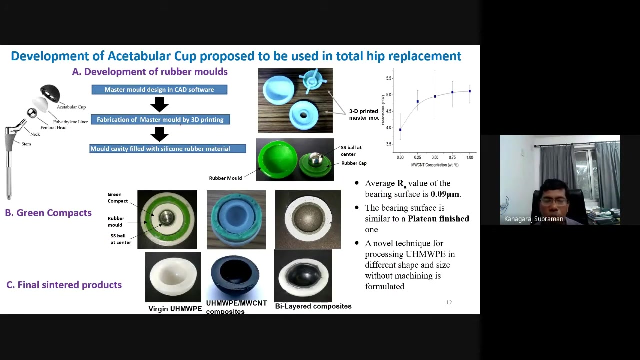 diffuse one by one, okay, and you can see here that there is grain boundaries, that bond is, particle bond is are getting diffused, okay, and after that there are deficient and there will be no boundary at all. okay, this is what you will be having, that semi-strength volume, and this is what, how we could. 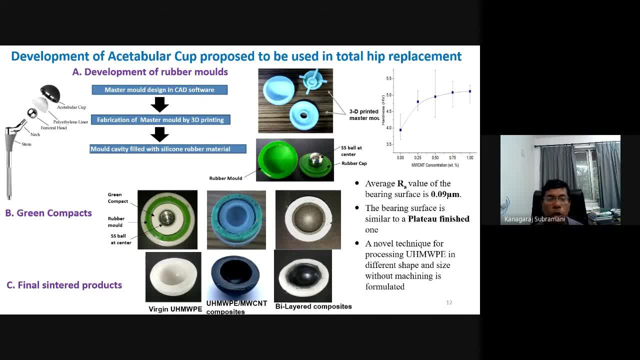 we could get that product okay and this is for virgin polymer and with the reinforcement it is a. we have used a different type of cmt and in this case the properties we have optimized and it found to be 0.25 weight percentage. earlier case it is 4060. it is about two weight percentage. 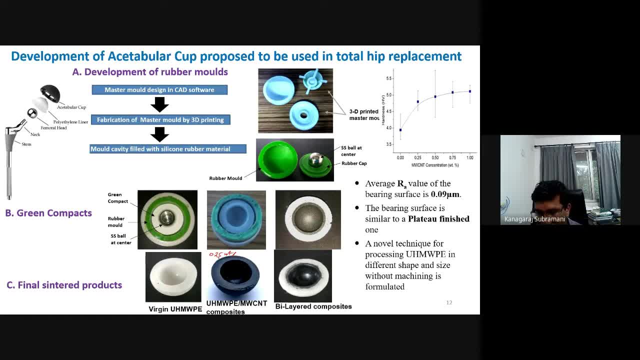 we are where we found optimum and in this case a different type of nanotube, it is about 2040 type- and where we could read: they obtain the best properties at a point two, five, eight percent percentage itself. this is what cmt composite, okay, and this is what the bilayer- bilayer in the sense. 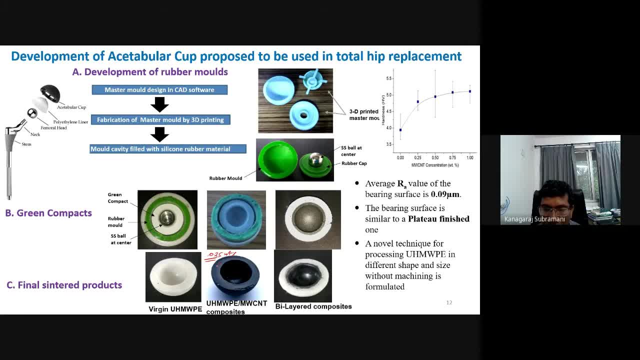 even 0.25. also, this is what that bearing surface may be, up to 2 mm thickness. if you have that reinforcement, then still we can reduce the requirement of the carbon additive. that's what we have made it. still, we are working on that processing parameter so that we can get 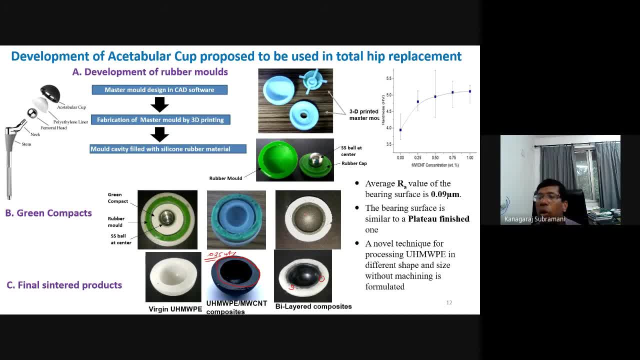 a defectory products and all like that. okay, this is what a Post, a 0.25. you are finding more or less that: the same hardness. that is what we have designed it. okay. so the flat advantage is that a flatter finish and 19 nanometers. that is what okay this. 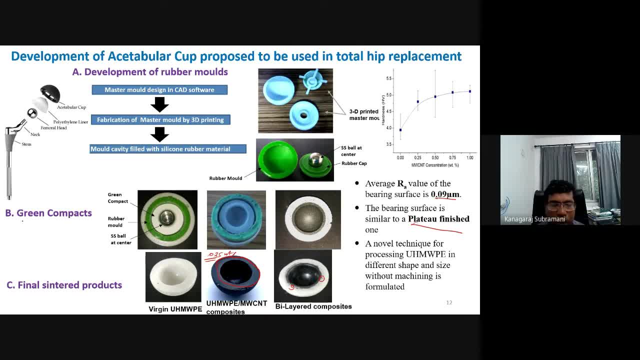 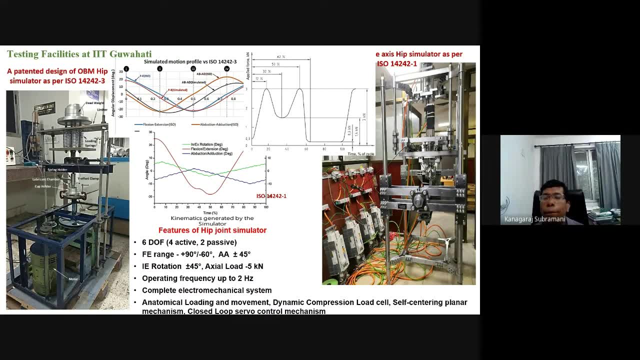 is a final product and this, what we have, this is a product, what we have made it and we will be testing it. we have been testing it also and in order to do the testing, okay, we have developed a two different simulators, and one is with the iso one, four, two, fourробl. okay, we have developed two different simulators, and one is with the iso, one out of four types, so this is the first one and after that the other types. okay, so using 거죠 mit az iSo one, four to four, 3 of them. i's good when you consume too much, right to. 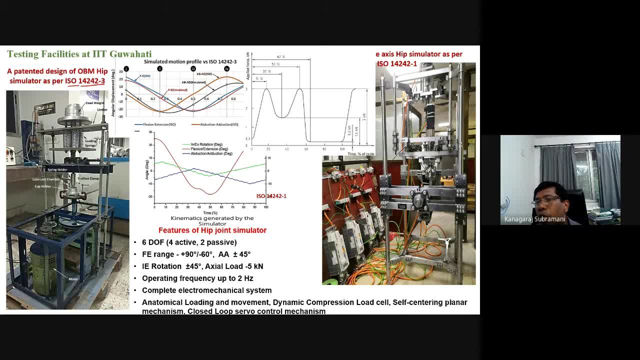 so into that in order to do all four. so we are that advantage: we have used the contribution method to four to three. another one is four to four to one. okay, in this one, what you can see here, uh, you have a three. as i said, this is aspect that: four to four to one. you have a three degrees of. 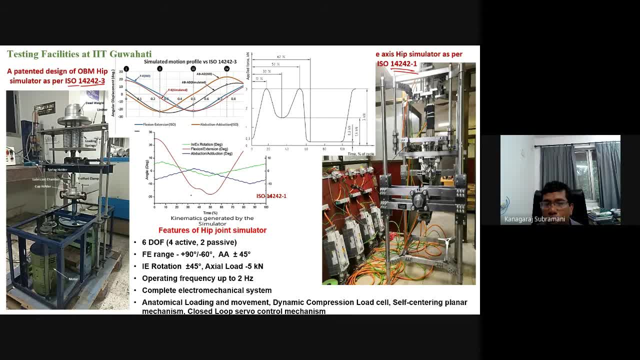 freedom. you can see that this is a flexion extension about a plus minus 23 to minus 23 and after that this abduction adduction and there will be internal, external rotation. here you will find that three servo motors. one is one will be here. okay, so servo motor, one motor will give a. 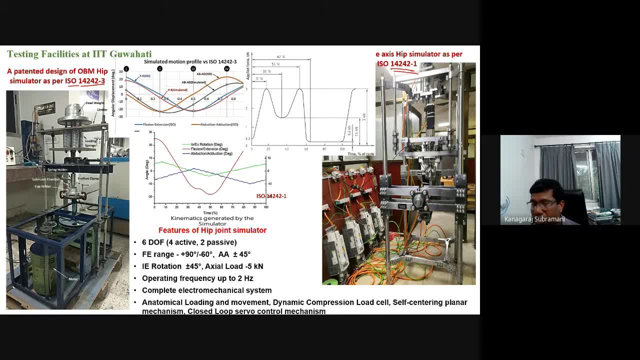 flexion extension. another motor will give abduction and action. another servo motor will give an internal, external rotation. another servo motor which is connected with the screw rod, will give that a dynamic loading pattern, as per this one you can see here, this is what you know- within 100, one cycle, it's about 100, okay, thousand microseconds. you can say after that, within 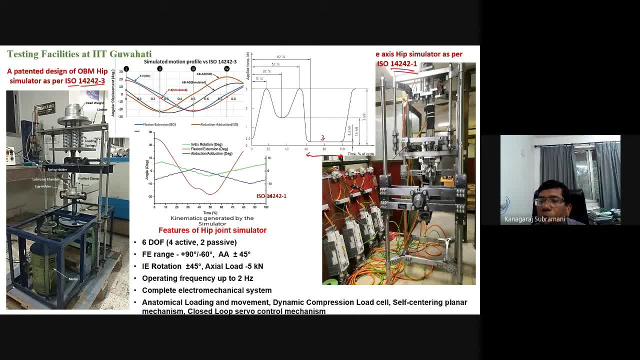 near about 400 microseconds. load will be only 300 newton and within a 60 percent of it. at a two point of time it is reaching a three kilo newton. at one point it is reaching at 1500. so this is what the dynamic. 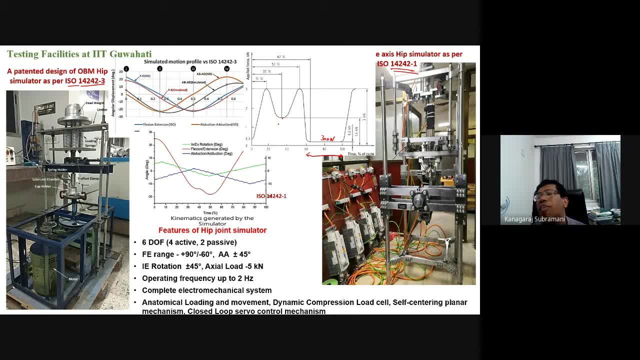 profile within a second. we need to have this kind of dynamic profile. uh loading profile. we need to go at the hip zone, okay, and this one we and we need to see that, uh, for up to five million cycle, how that weird bridge generation or the surface profile and 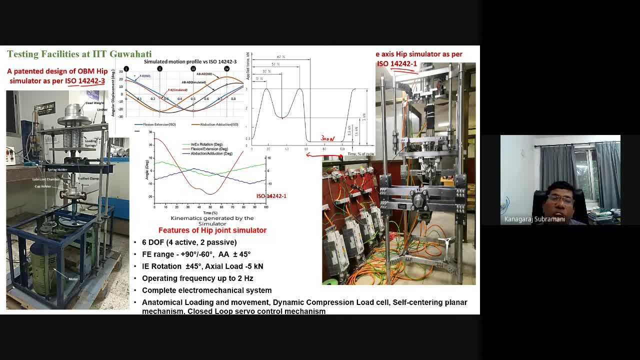 all we need to do that testing. okay, another one we have made with iso one, four, two, four, two, three in this one. what is that? it has two degrees of freedom. one is a flexion extension, another one is abduction reduction. here only we don't have, uh, internal, external rotation in addition, whatever, 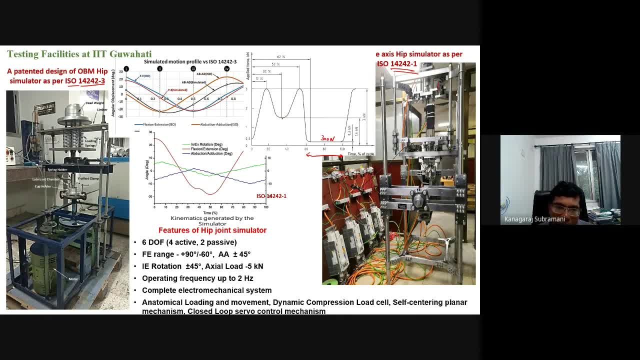 that the dynamic profile we could get it here. the same dynamic profile, we could get approximately the same, not that exactly the same. in this case, uh, we will have a near about a three thousand and a. after that it will come to that near about uh 300 and it will be 150 then after that. this is what. 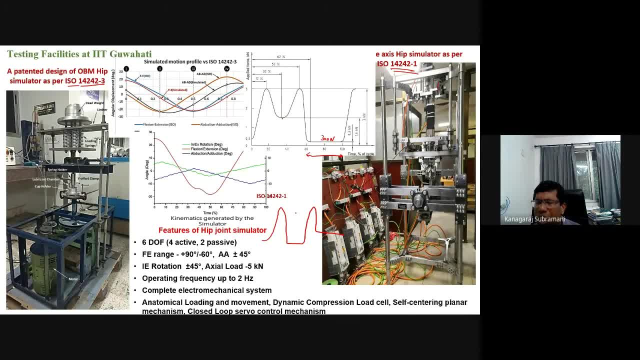 more or less we could get it okay. however, it is approximately 75 percentage of the dynamic loading profile. this is about uh 3000 newton, okay, and at some point of time, uh, this is about 300 newton. only the time the scale will got a little bit different. however, that's what i'm saying here about. 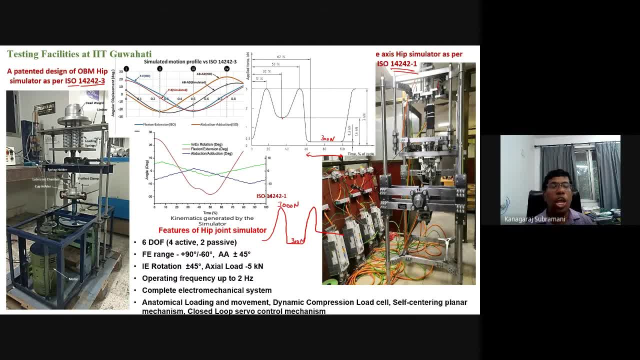 load profile we could get in the mechanical system itself. here only one dc motor was used. okay, to have two degrees of freedom along with uh dynamic load profile. okay, and here you can see, in this one you have a cup holder and uh cup holder along with a dynamic. 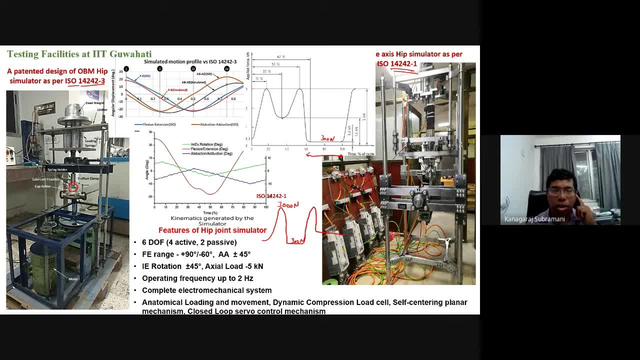 profile. okay, so this, what, what? we have tested it. uh, as per that iso one, four, two, four, two, three, and we are just working. oh so, when you look at how modern has converted the dynamic profile, this is kind of a owej one whole system. is you know about more or less we could? yeah, we have tested it for. 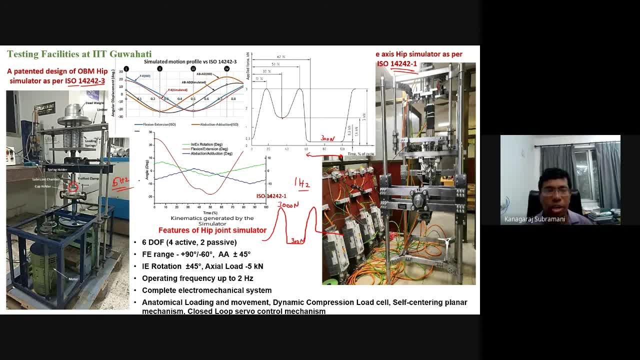 five million cycle, okay, five million cycle. and here this will run at one his and and this. we are running at only five kilo, five heads kept, five hertz. uh, frequency only: okay, just in order to reduce the time span of it. however, even we have a lot of options, even if you. 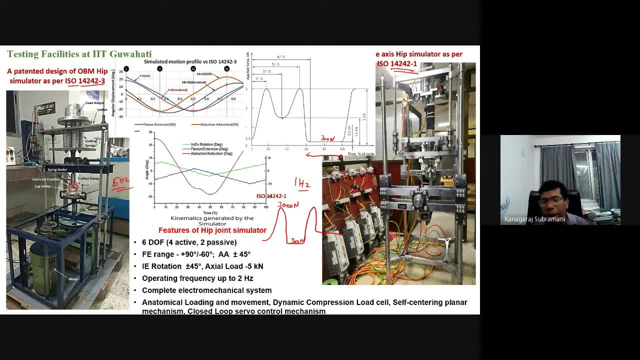 three degrees of freedom also okay, and we have a wide range. that flexion extension, though it will be plus 23 to minus 23, we have a different option. within that, we can have that, all the modulations and all like that, okay. so this is what, the development part, and we have tested it, and 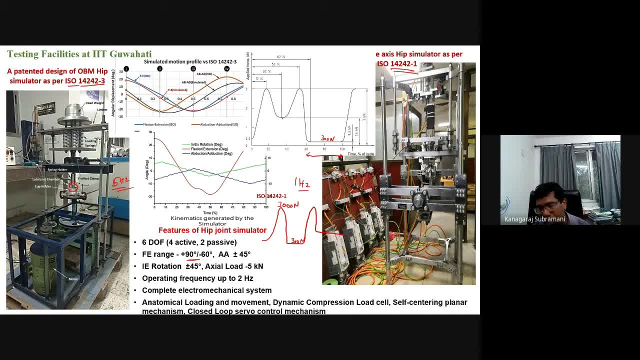 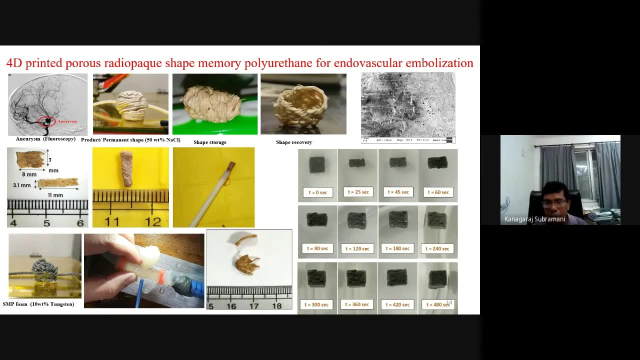 the debris generation also, we have controlled compared with pure polymer and it is also found to be less compared with what is what is reported in that literature. okay, and that is what a stub lurker. what is being used in a hip joint replacement, and hope it is understood if you. 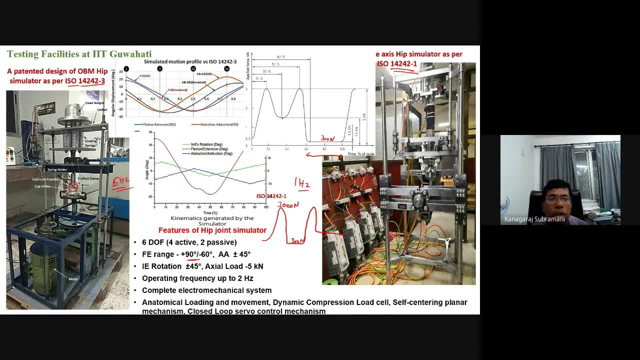 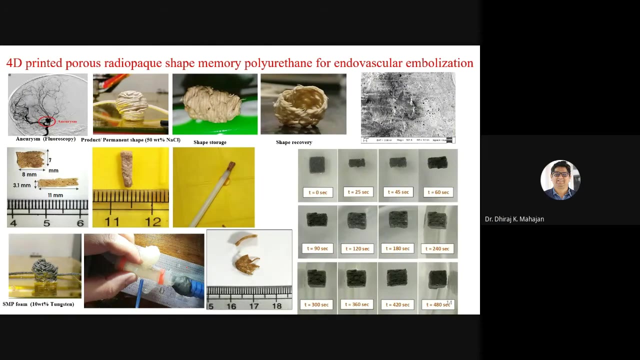 have any query, you can ask me also, otherwise i will move forward and finally you can come back. we can come back to the question answer session. hello, uh, yeah, yeah, professor, we can continue. i think, okay, it is okay right. another implant category is: uh, shape memory polyurethane endovascular embolization. okay, so right, this is. 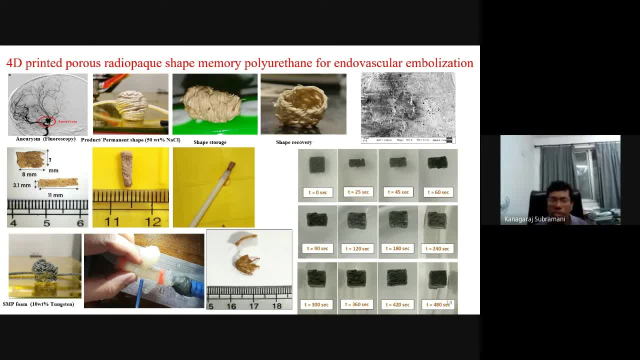 you can see that aneurysm in the blood vessels. suppose in the blood vessels at some portion of it it lost its stiffness. then it become a balloon kind of it due to the blood pressure. then that whatever it is, a balloon form of it is, it is going to burst at some point of time. then that mortality rate is very high. so once if 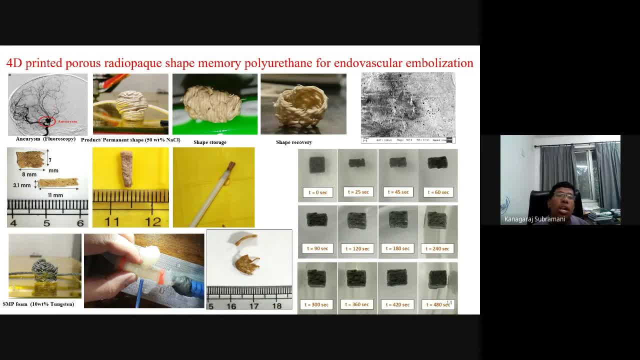 it is identified that the doctors are using a platinum coil. they are filling it in that aneurysm just to ensure that the packing factor is sufficient enough so that the blood flow will be restricted. okay, so what we are planning to do is that, once we get the shape of that aneurysm, 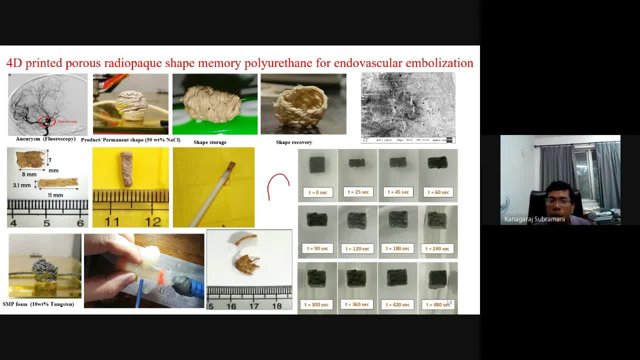 we will be getting that 3d printed shape of it. okay, this is what that ballooning. okay, this is. however, it is enlarge version, by the way. okay, we will get this and after that, uh, we will get the shape of that aneurysm and that same thing. 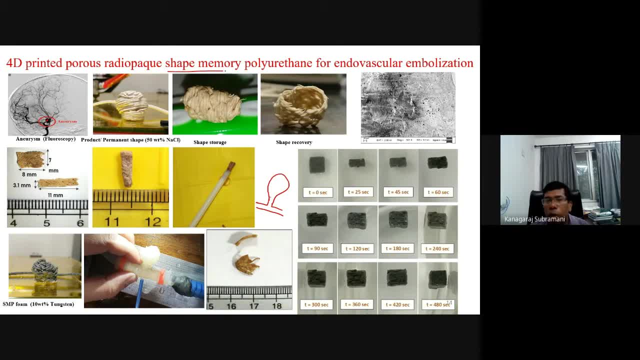 will be getting a 3d printed using the shape memory polyurethane along with a radiopack material. here we have used nanobaryon sulfate. you know barium sulfate is being used as a milpre presents radiopak material in a bone cement applications. 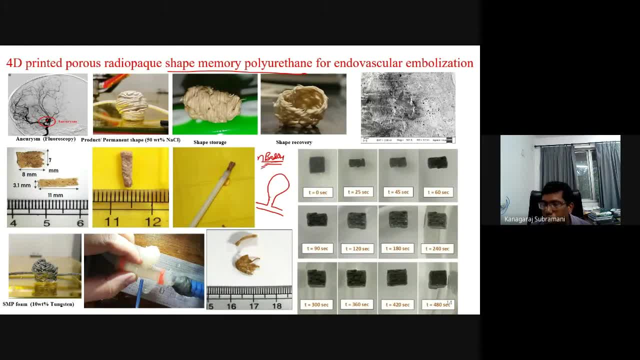 uh. however, in order to reduce the concentration, we have used a nanobarium sulfate, which will be having a higher radio pack or equivalent radio pack with a lower concentration in a conventional case. here, what a 10 by 8 percent is being used? here we have used about one or two percentages. 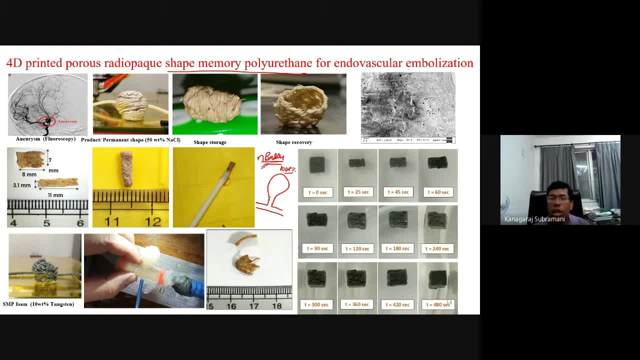 okay, in order to have a desired radio pack. okay, and after once you make that shape of the aneurysm, as it is having that shape, uh, shape, memory characteristics we brought, we converted in the form of wire. okay, converted in the form of what the future plan is, that that wire will. 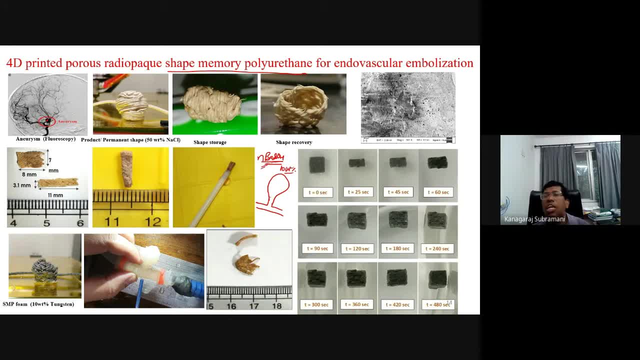 be attached with the catheter and it will be deposited in the aneurysm zone. okay, this area, and here the temperature is the external stimuli. okay, so as soon as it reaches that body temperature then it will get back to original shape of that aneurysm, so that packing factor will be good. blood flow could be restricted. 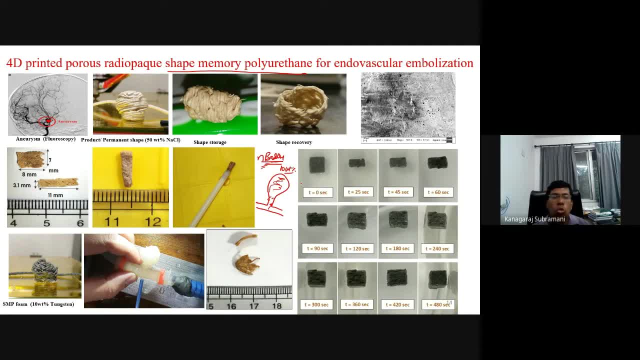 to the maximum possible extent. okay, so this is what that, what our plan and we have done: a shape, memory, polyurethane and that here. initially we started with the tungsten. okay, uh, and tungsten and tantalum. sorry, not tungsten tantalum. we have used it because you know you. 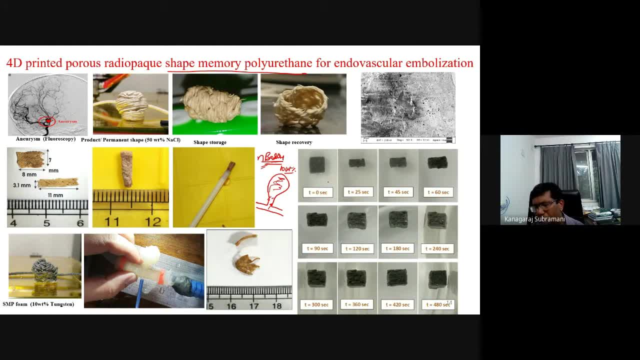 may be knowing that one, x and all being used and eoh also being used along with the tantalum. okay, so this is that shape memory characteristic, what we did. okay, so initially we have made with a one centimeter cube, okay, then one of one of its sides got compressed by 50 percentage. 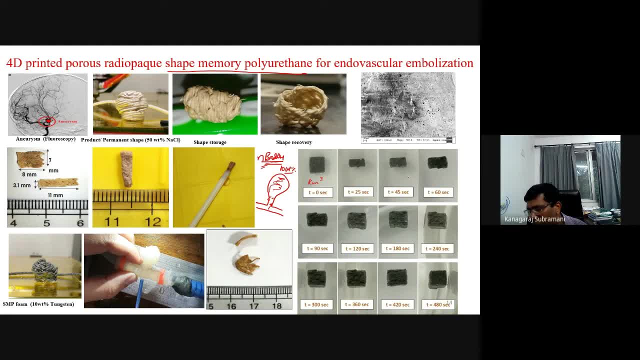 and it was kept it in that near about 38 or 40 degrees centigrade. okay, this is external study. okay, so at a different interval we could, we watched it and we ensured that it is coming back to the original shape of one centimeter cube. it means, though, it takes about a near, about. 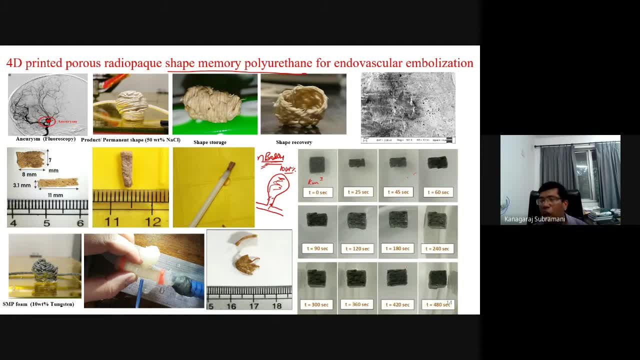 what you can say. eight minutes time so we can manipulate or we can play with that timing and getting that exact recovery rate of recovery. we can manipulate depending on the record. so in that way you can say, once you are inserting through the femoral artery till it reaches the desired, 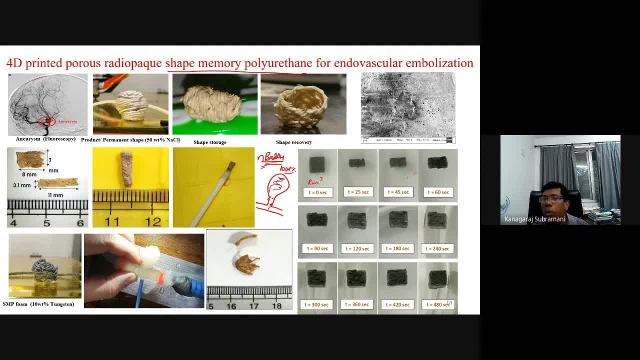 destination. if it is taking five minutes time, so till five minutes time. we need to ensure that it is not gaining its original shape. we need to retain it like that. that is what this study we did and for in vitro study what we did. we get that sample- 8 mm, 7 mm- and these are two samples. okay, and this: 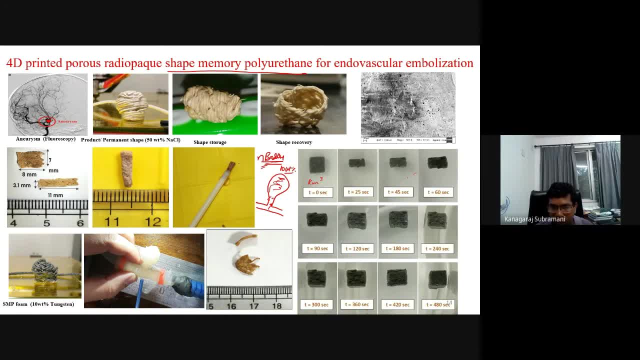 after converting into the secondary shape, it got inserted. it was inserted, okay, in that catheter form and we have made a silicon rubber and this aneurysm also, though it is an enlarged scale- okay, if the lab scale- we did it okay, and here we have ensured that the pulsatile flow is being carried up. 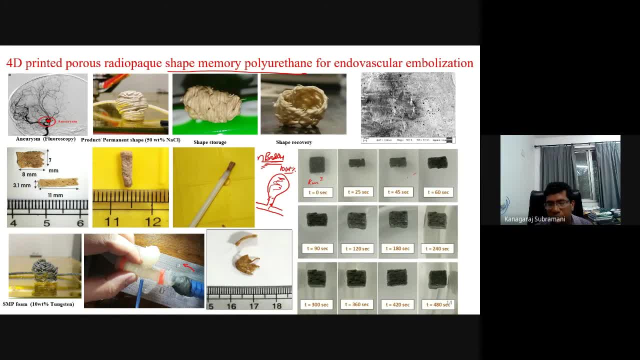 okay, the water will flow in a pulsatile medium, like pulsatile flow, like a blade which is pumped from the heart. water the way it goes, the same flow rate with the pulsatile flow. and here we have this inserted: that shape, every polymer within that. then after 10 minutes and all like that, we have. 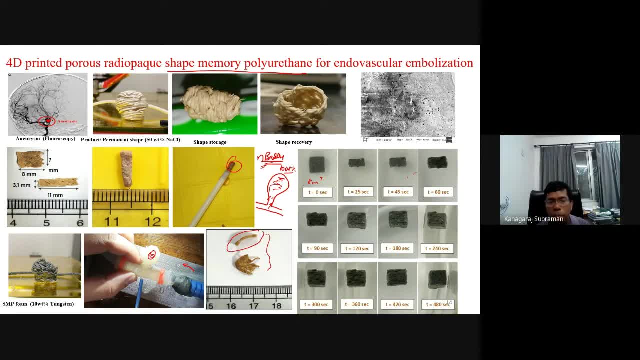 removed it. you can see here. this is what the shape here, what we got it here. also, it is more or less that the same shape. we could okay after once it reaches the desired destination, after 5-10 minutes, we could ensure that the raw material shape whatever we have desired. we could able to. 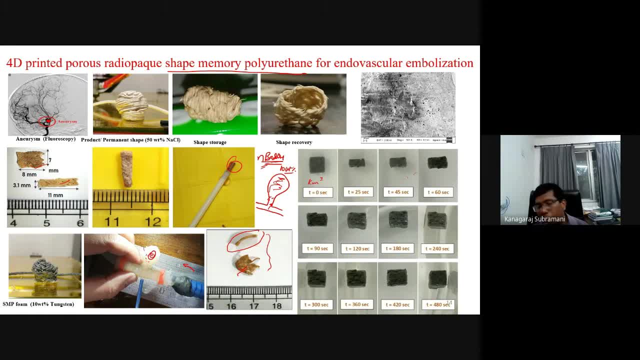 achieve that, that's what fine. so this, what we need to take it forward to, that maybe animal study. then after that we can think about a further study and all like that. this is a proof of concept, uh, which could be explored for that treatment of that aneurysm here. the purpose is just uh. 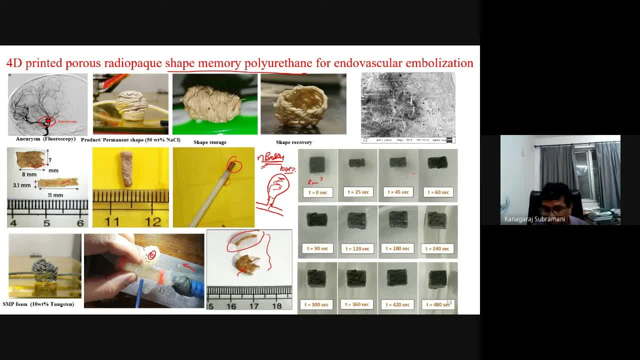 to replace that platinum coil. that's what? okay, so in not only the platinum coil replacement, increase the packing density also. so in this case the entire aneurysm volume will be blocked. so there won't be no further blood flow. it will be like a solid liquid embolic material, like a onyx and all. 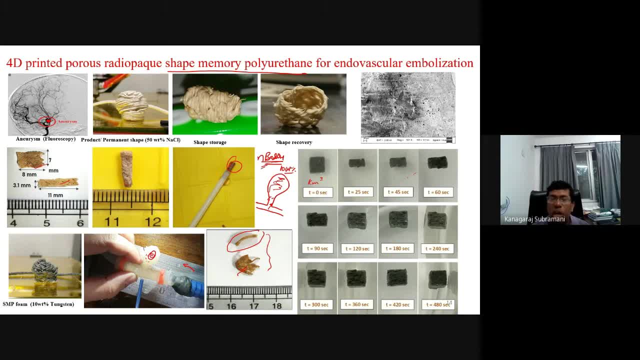 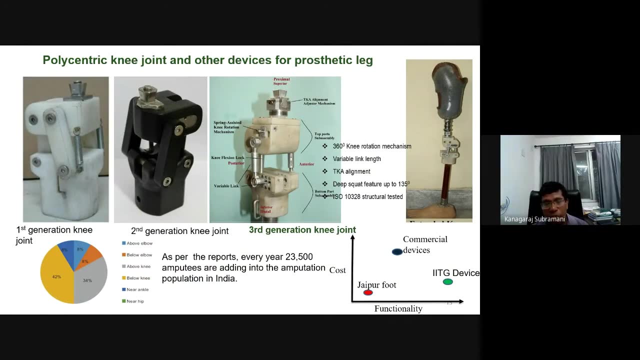 how it is. restrict the blood flow like that we can with a solid metal itself. we can restrict the blood flow, okay, with a small volume of it, that's all okay. this is what the shape of polyurethane for endovascular embolization okay. next will be that, our prosthetic device. we are working. 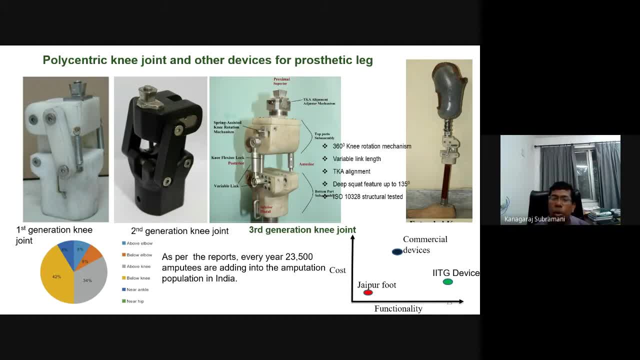 on a prosthetic knee joint. okay, and right now what we are working is a third generation. this is what the first generation knee joint- okay, so it could go that flexion extension of around 90 degree and 2 to 95. okay, and this can go up to 135 degree knee flexion. and this is second version and this 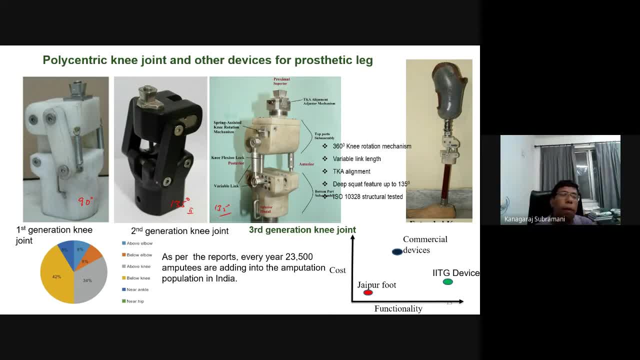 is third version: 135 knee flexion- okay, and here that extension spring is kept outside. this is the first generation and after that, patient feedback, this: we have tested it for around 12 to 15 subjects and this also 12 to 15 subject- okay, and this is now right now we have fixed it. 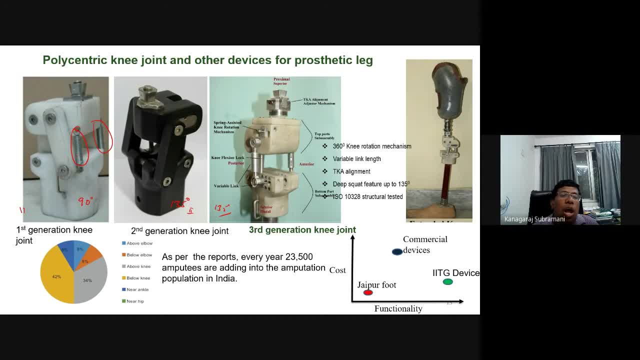 for three subjects. and still it is going on okay and this spring is outside. so they were talking about: uh, if it is inside, it will be good. so we have kept this extension spring inside. this is a torsion spring. we have kept it and, in addition, this in the second model, we could have a deep squatting also. 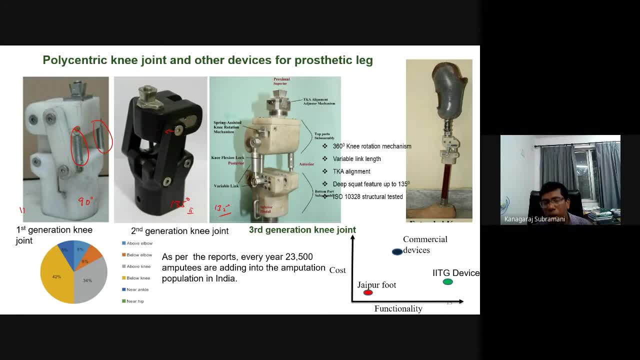 in a conventional four bar mechanism, whatever it is commercially available. you have a deep squatting, however, that a patient needs to put a lot of energy to bring back other what you can say. once the person is a deep squatting, it will be in that stagnated position. 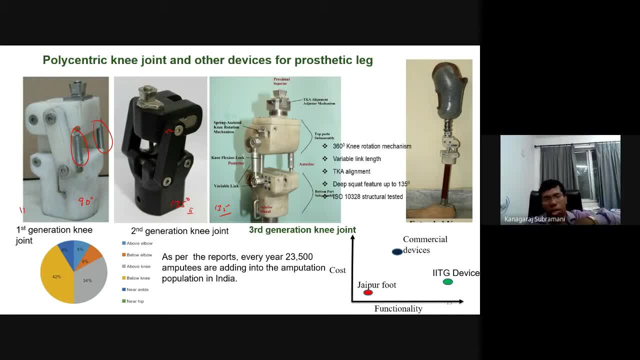 he has to pull it back to the original position. the leg needs to be brought to the normal position by the patient himself, but here, as soon as he gets up, it will be that that torsion hinge mechanism will help him to uh bring back the leg at the original condition. normal flexion will do okay. 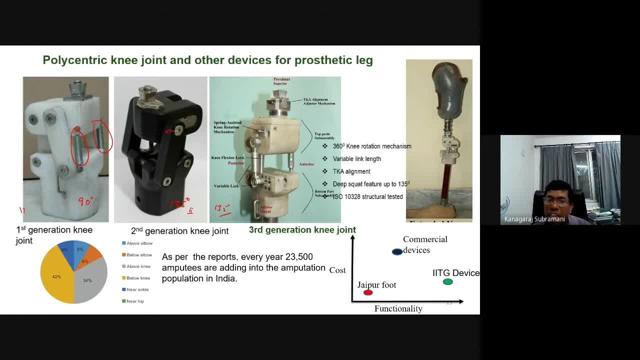 uh, this torsion, as well as the deep squatting we have incorporated here, and in addition, this uh device is also having the locking mechanism. suppose the person is uh. locking mechanism means it is a simple four bar mechanism, so you will be having a knee flexion extension. suppose the patient. 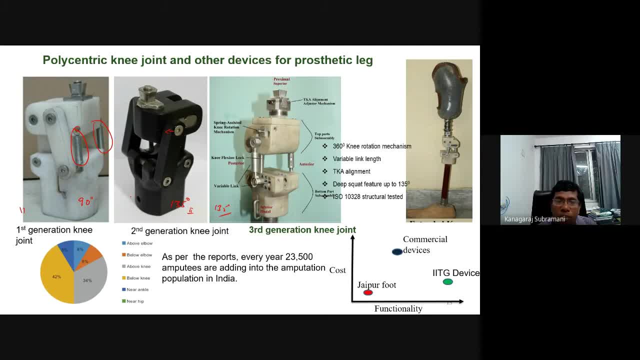 is not capable to do the flexion extension. we need to have a locking mechanism. so here, at this case- here you can see some- yeah, in this case you'll the top part and the bottom part will be locked. okay, so there won't be any flexion. the same thing will be here. here you can see that. 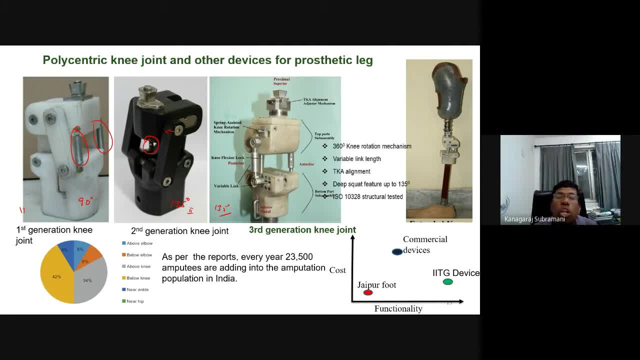 locking provision here. it is not that much visible. okay, so the locking provisions. by that way, we can lock that knee flexion extension. okay, this is the second version. this is coming to the third version. we have made three different options apart from deep squatting and knee lock provision. 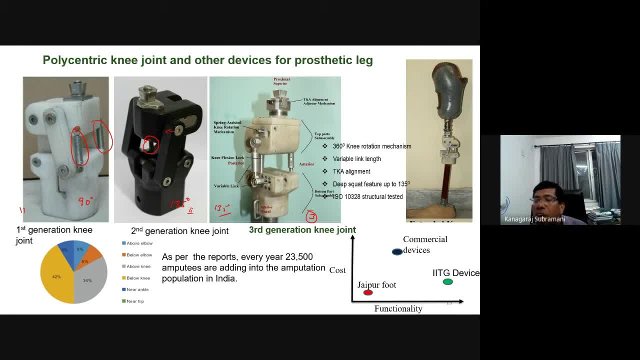 and torsion hinge. we have added three more options. one is 360 degree knee rotation mechanism. okay, this is what spring is: steady, just to pull it. so you hear it that both upper part and the proximal part and distal part will be disengaged. the socket and the tibia will be disengaged. 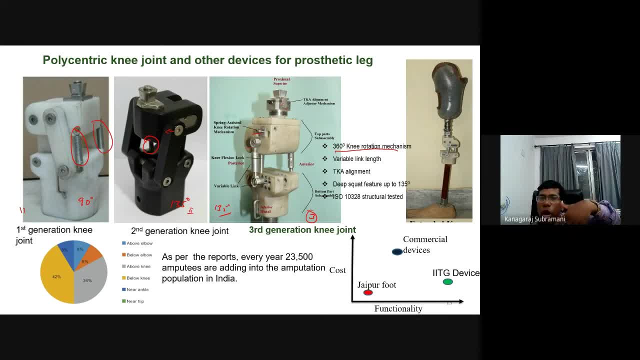 so what will happen? he can do. he is a regular kneeling down or sitting on the chair or holding the chair. uh, his leg, that is everything is possible using this mechanism. okay, there's a first one and second one is a variable link length mechanism means here. these are all, if you see that. 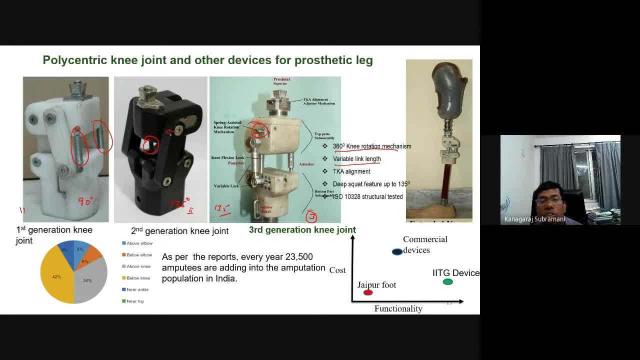 this one and the existing prosthetic knee joint. if you see, these are all fixed. four bar mechanism: okay, it is a normal four bar mechanism. okay, these are all linked. link lengths are fixed. however, here we have may given the provision for increasing or decreasing it. also, here it is a vertical variable length and this is what the horizontal variable is. 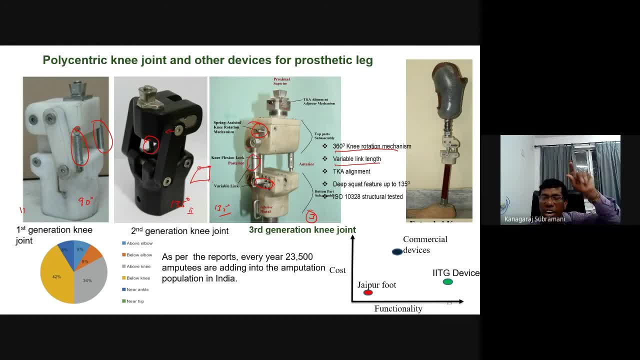 so what is that? if you have it, you can place that instantaneous center of rotation. we can place it at the desired location. if you keep on moving that position of the horizontal link as well as the vertical link, what does it mean? you can increase the stability of a knee joint, suppose for elder people, older. 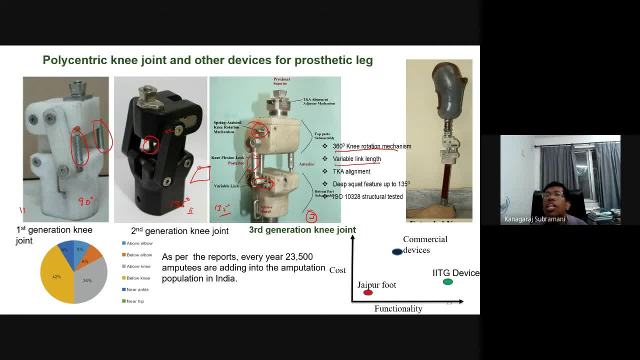 people. if you want they need more stability, okay, for that you can bring that str far away from that knee center, so that will give more stability. or if you wanted to use it for younger people, so they can, uh, but by themselves they can have that more stability. in this case, what can be done? then you can bring. 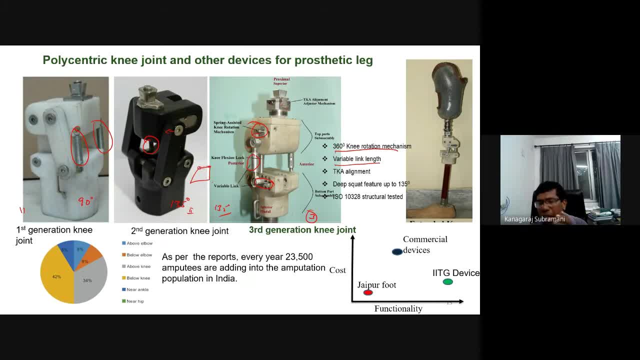 that knee center nearer to that so that, as they can stabilize by themselves in this case, that knee flexion extension will be very easy. if you have a more stable, that flexion extension will be. little means that they need to put a little more energy to have it easy. flexion will not be there. 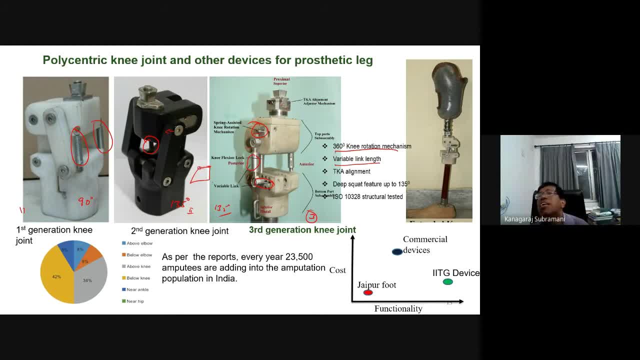 more stability will be there. if you sacrifice a little stability, then only flexion extension will be easy. easy flexion will be there. okay, that is what you can have. in addition, if the height of the person, if it is varying it, so, depending on them, for the same stability or the same. 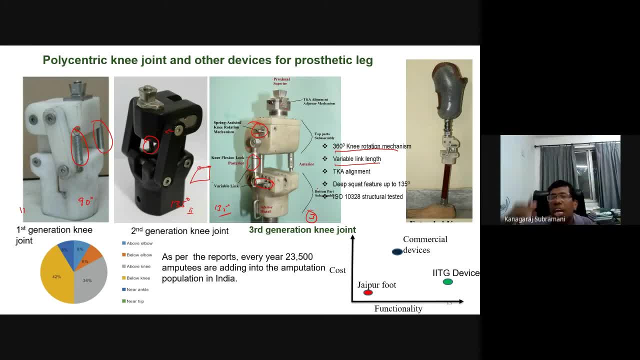 easy flexion. you can increase the link length so that it will be at par with the knee, hip center and all that. okay. then third option is a tk alignment. you can see here here about a 10 mm. you can have a posterior, anterior, posterior movement. okay, the load line and the knee are. 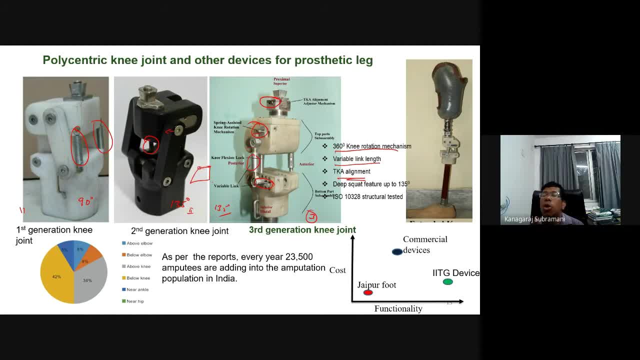 axis, if you wanted to adjust it. this is more mainly it is required for a prosthetist during that alignment fixation. so depending on the patient walking capability or that his condition, he can adjust. it's the link, adjust that. it uh. tk alignment- truncated knee alignment- that he can do. 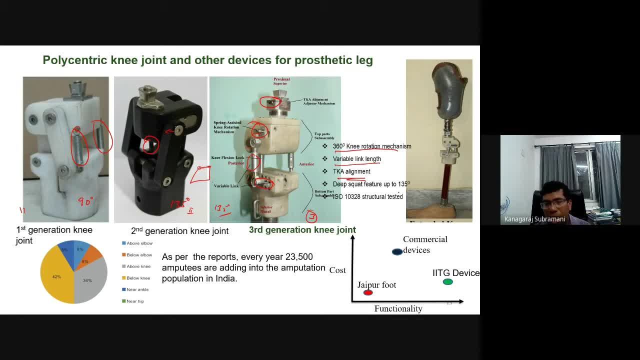 that okay, and we have the deep squatting up to 135 and we have tested as per the iso: one three, one zero, three three eight, okay. and our objective is- you can see that we wanted to increase the functionality at the same time, at that low, at the affordable price. okay, that's what it is and this is what the first generation 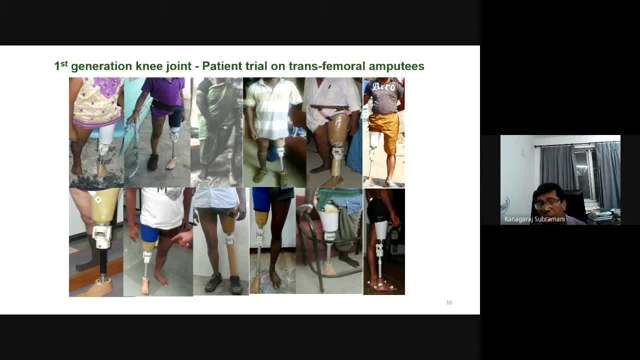 knee joint. what we have used it, you know, some time we did it in a negrim shillam and some of the patients who are from a prosthetic clinic center at kanyakumari. okay, this is what some of the people whom we have tested it. okay, you can see this is. 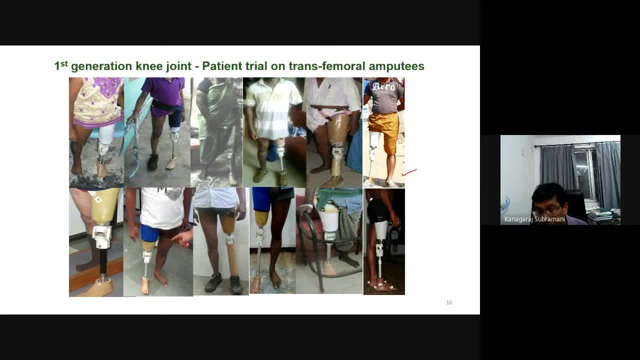 yeah, he is from uh, I can say from uh, with the batik group. we have collaborated, they have used it and this is for gate in a mgm hospital, Mumbai, where we did that gate analysis of it. okay, that's what this is. the different knee joints, uh, different subjects with the first generation knee joint. 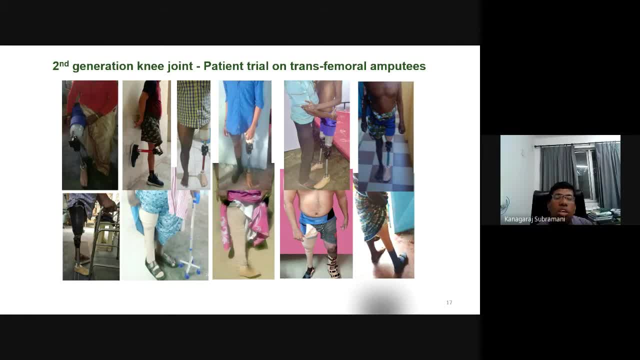 and this is with the second generation knee joints and you can see here this is the one army person, how he is. it was very good and it was and more. most of the things have taken on the day one only after fixing it, and we have fixed it for a bilateral amputee also. 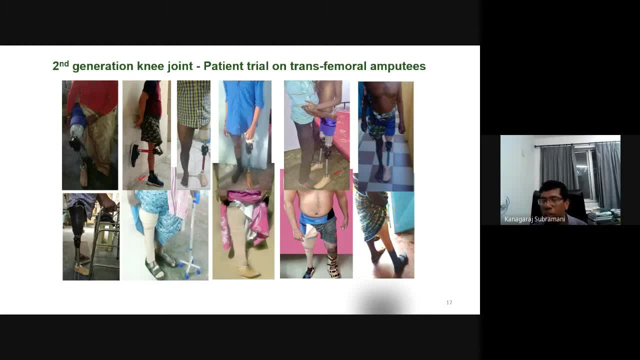 okay, maybe initially it will be in a locked condition, where that the patient needs to, in a bilateral condition. most of the time the prosthetist used to suggest the person need to stand at least, uh, till he get a confident. until about one month period they will be simply sitting. 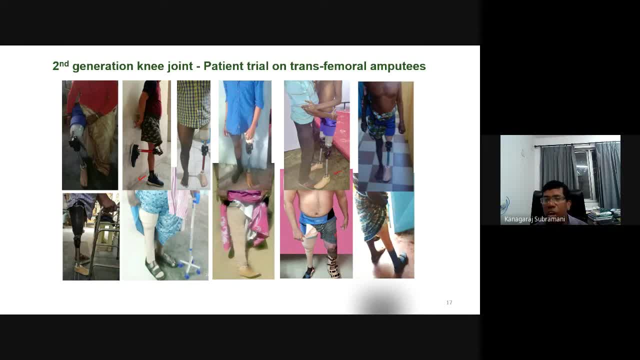 and standing only. they will not have any walking. then, once they get a confident, then after that they slowly, slowly. they can go forever. initially it will be in a locked condition, they will be walking and after that they will be having any flexion extension and all like that. 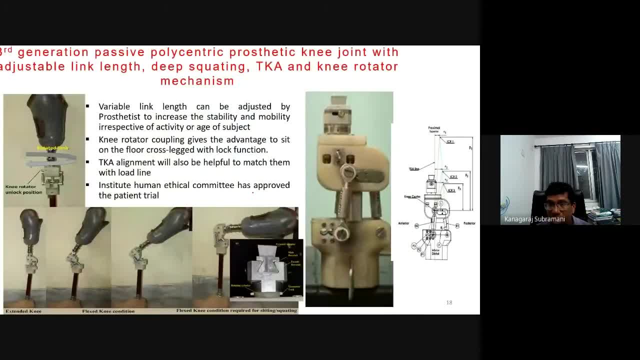 okay, that is what and this is what the third generation, what i was telling them. so you can adjust it. you can have a different alpha stability as well as the beta stability. you can adjust that any center and all. or is that what you can say? instant instantaneous interpretation. 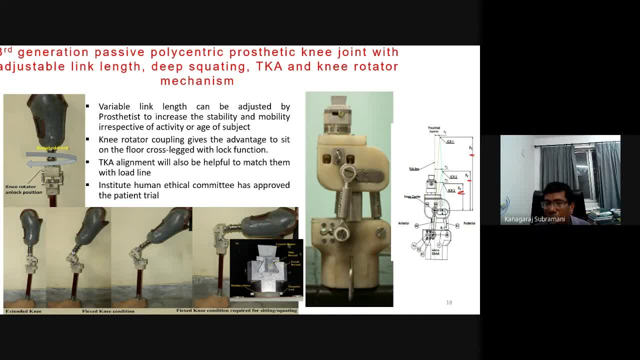 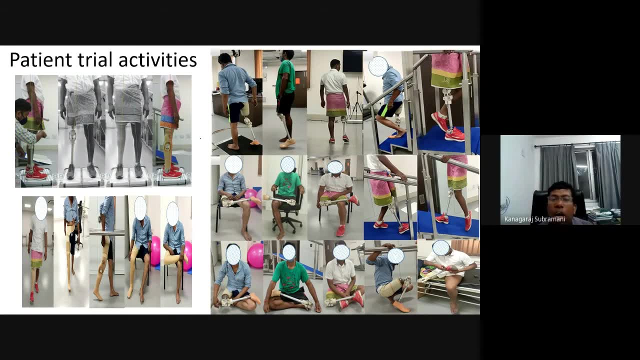 but and this, what, as they said, we have done for three different patients, okay, and this is in our gate lab what we have tested it and this is during a normal walking. you can see here how they are working in and all and even they on the day after that they have been given training in using the. 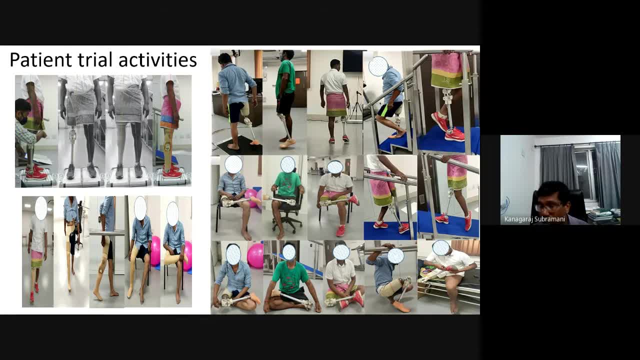 staircase without locking initially, whatever, we tried it with locked condition. in the day one onwards they started to practice without locking condition: reflection, extension and all like that. staircase ascent design and the ramp also. you can see here ramp walking, ascend and the descent also they are doing, and after that, as a knee rotating mechanism is there, they are sitting on the chair. 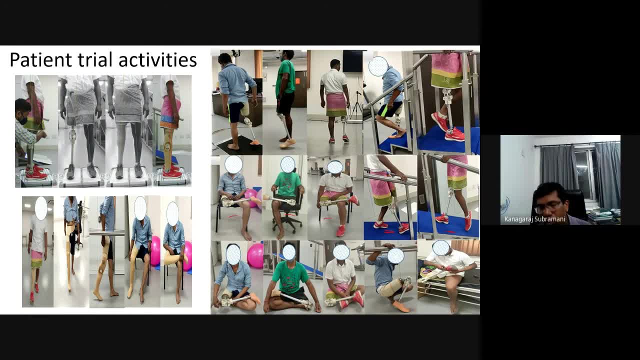 comfortably and they are sitting on the ground, okay, and this is what the deep squatting okay, you can see here and in addition, after that, the knee rotating option is that they can do that, where the shoe and lace and all everything they can do by themselves, the stool is tightening and all they. 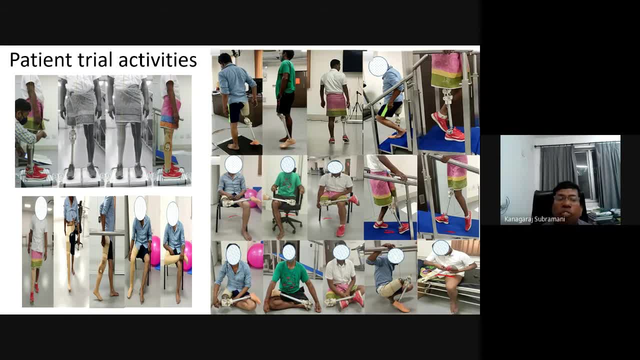 do by themselves. and this is what that alignment situation okay, not only that: joint making and fitting and all we need to make that alignment also okay. that, because it has a lot of assembly, mechanical assembly- okay, so we need to adjust the screw position and all in order to ensure that. 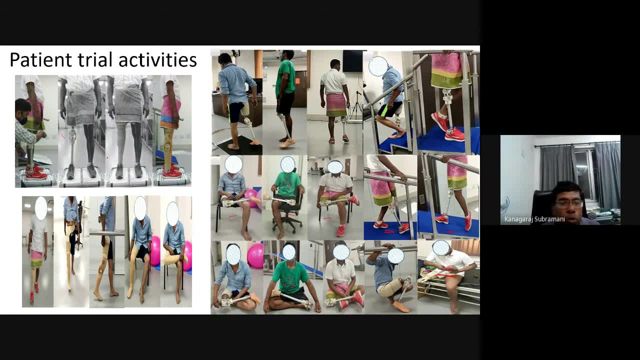 that load line is passing through it. okay, that's what we used to make it in our gate lab and this- this is after situation, how it will be looking like here. we have given provision for adjusting. this is what that till we are. we have given it for three subjects and a few more are waiting. maybe. 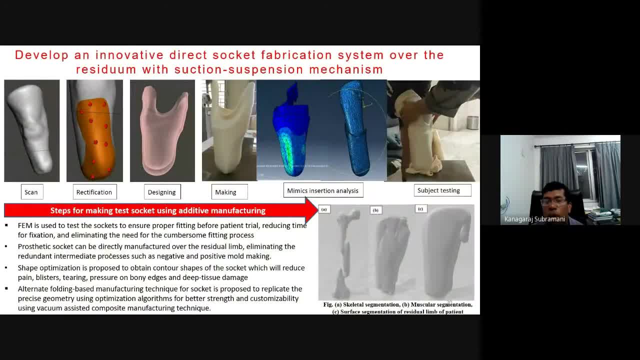 within we it is going okay. that's why, and coming to that socket fabrication system, and sometimes when we get, uh, this is, you can say for ebony amputees, this is what one army person- we got his mri data so okay, and this is what he is from mri- we could able to gather this information. 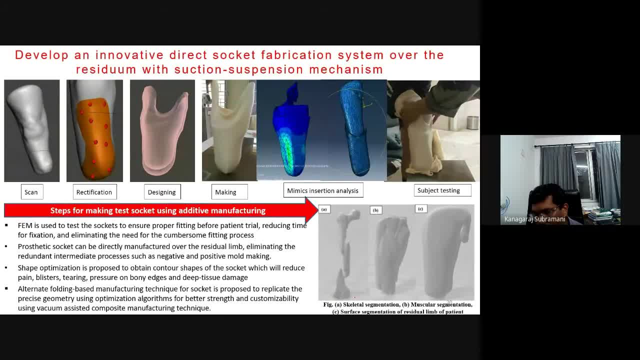 okay, you can see here it is exactly knee articulation and in addition, there are two fractures they have not diffused properly. okay, and the doctor said no more surgery is possible within that. only we need to do that. okay, so we have. we have been working on that socket design. 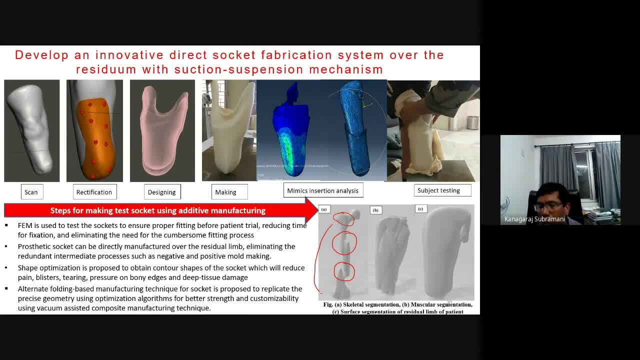 okay, so entire load will be bearing in this place. only it will be doing like that only. okay, so that there we have made a lot of trial. okay, so, even when, uh, before- we use the software or the stress analysis part, when they are using, even in order, but some other company, whatever, 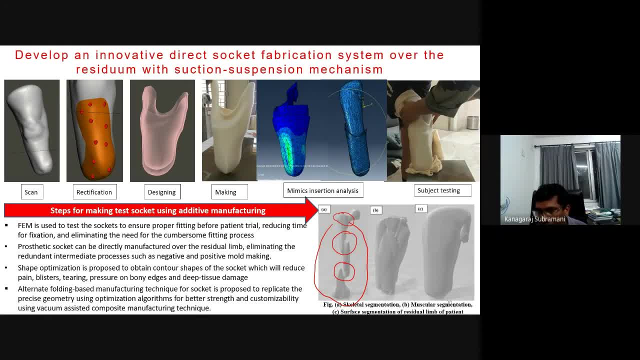 they are using it even three, four times. also, they have revised that socket. still the patient is not comfortable because of these bony prominence, because the stress pattern is even little bit. stress is more than when during that compression stage. if it is more, then that will be a point at which that failure is getting started. okay, during that analysis, that is what we 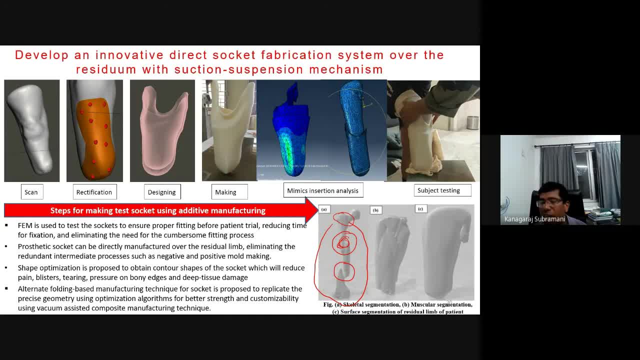 have made a different socket before, five different type of socket design we made, and during a damning as well as the during a heel strike, how it is the load is getting transferred and wherever the stress distribution is there. uh, no, no stress distribution is there, then we will remove, we will. 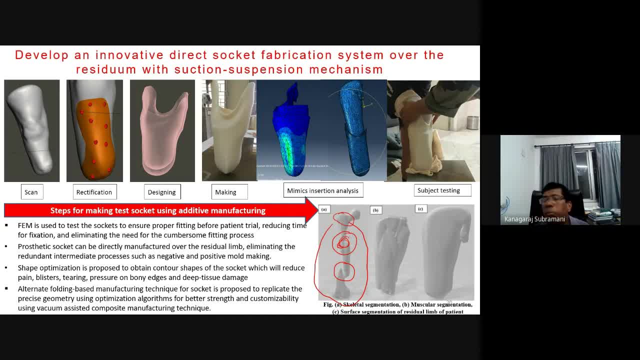 make a window kind of it, so that there will be breathing of the stem. the same thing we are having not tested with a subject- this is for ebony and this is for a bologna- we take that, a scan of that residual stone, 3d scan, and we do all the modifications or stress distribution and all. 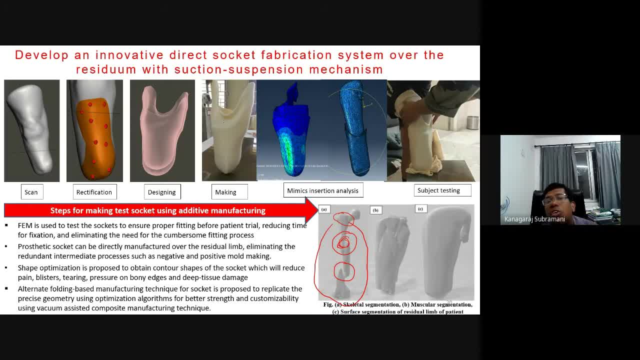 like that. then after that we make a 3d printed socket. okay, then, this for bologna as it is. it is depending on that. when a orthopedic surgeon used to say that the angel, angel fracture and complicated fracture, this could be useful only for the angel fracture kind of it. okay, we have. 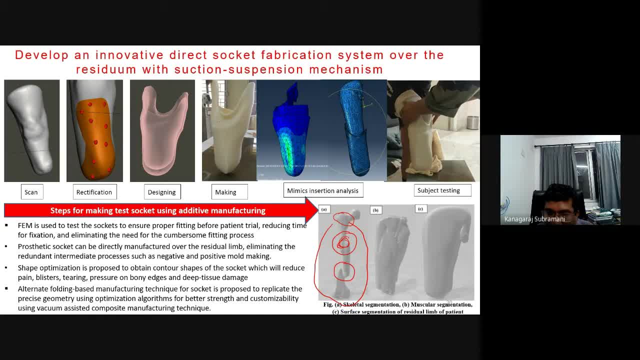 this, what that after making it. once you make this one, then we need, we are. we have been discussing with the prosthetist and all like that. okay, then he will be giving a lot of modification where it should be pressure point, and all like that. this, what after that? it will be a you cannot make with. 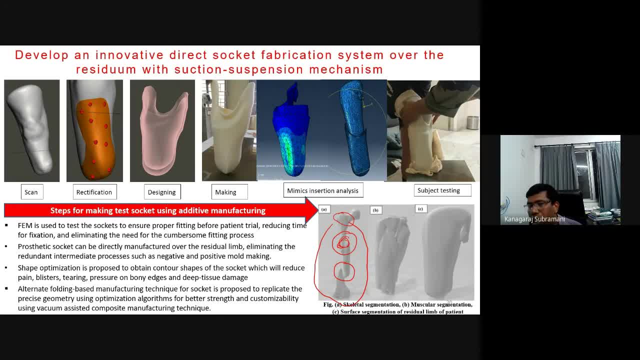 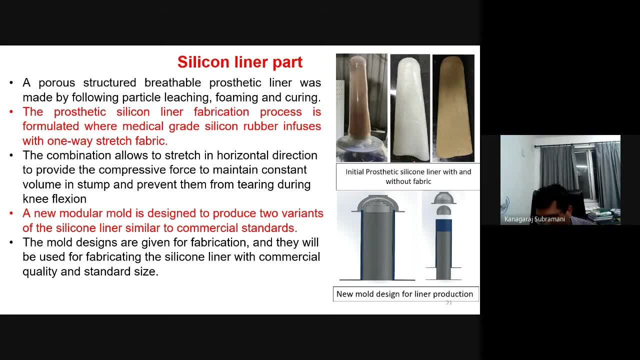 conventional. so that's what a 3d printed we did and after that we have tested it also okay, and we are working on the liner as well. you, because if you use that conventional one, the liner itself, in a conventional case it's costing about eight thousand, and all like that with a breathable liner, silicone liner, which could be. 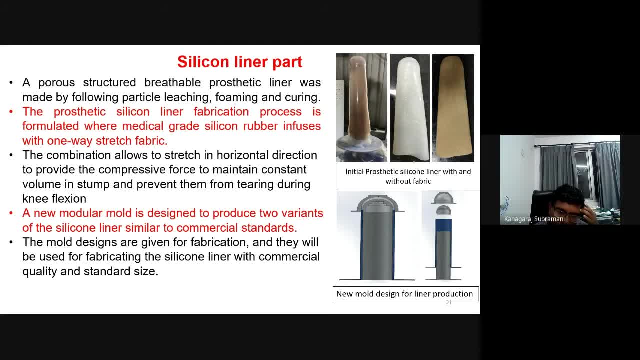 different, variable shape for a different people. that's what it is. okay, we just started. okay, we have not. then we have not made anything right now, we are just conventional. whatever that commercially. if they are using a socket liner fixation, sorry, what is the stocking layer? and after the socket? 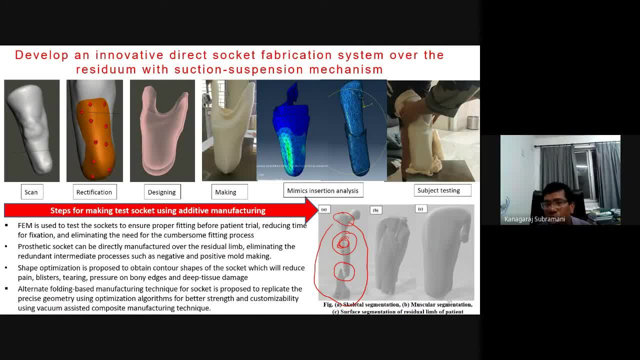 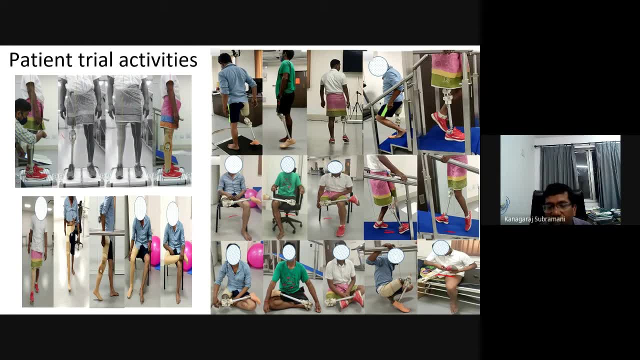 so in other case we use to keep suppose in this: if you assume this one, maybe you can go here. okay, so in this socket, whatever he is wearing, we inside there will be easy, it will be nail alcohol, so that it will give some kind of a cushion, even wherever, in some cases, uh, where that there are some bony prominence, so that also with 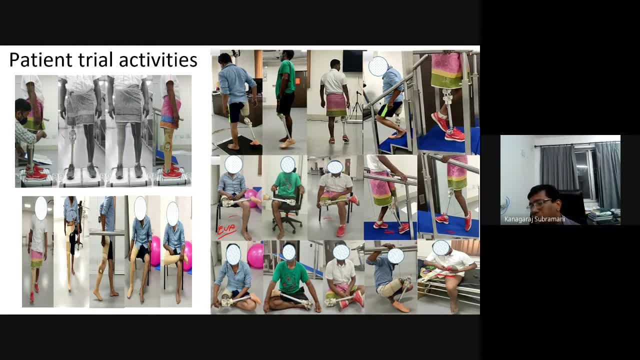 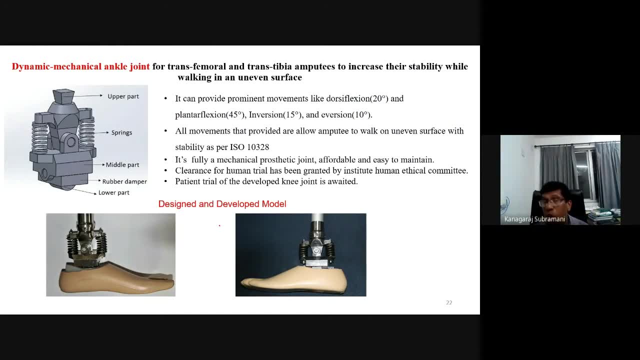 eva will not allow to have a addiction over the socket, so the pain will not be there for the particular subject. okay then, apart from a knee joint, then we are also working on um ankle joint, also the dynamic ankle joint. okay, so this is what that ankle joint viewer, this also we have made with that iso 10328, whatever that kinematic. 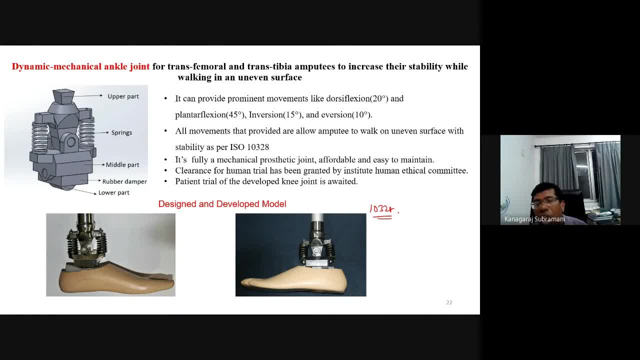 the dorsiflexion, plantar flexion, as well as that inversion, aversion, or it can be for pronation, supination and all like that. okay, this we have provided. on that ankle joint and this was fixed on a different kind of foot, even this foot itself. it is about a two thousand rupees, okay, otherwise. 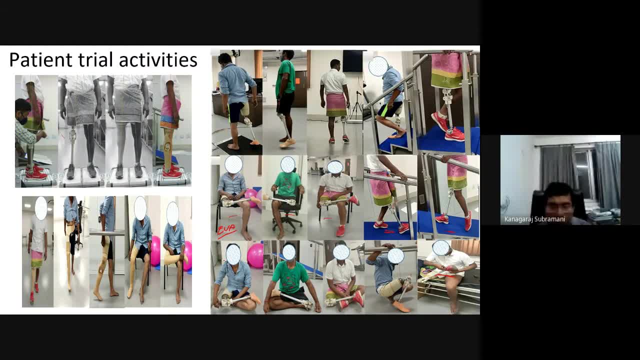 the rigid foot. what you are seeing here in this case- in this case, you see, this is sac foot- is around 700 rupees. okay, because we cannot give it two variables for that subject. that is what for when you are using a prosthetic, this polycentric knee joint, we use it only for a bone amputees. 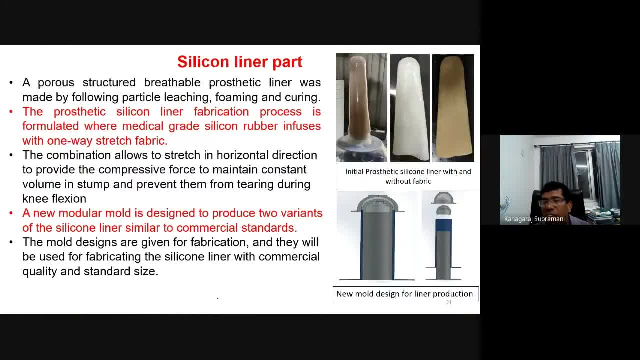 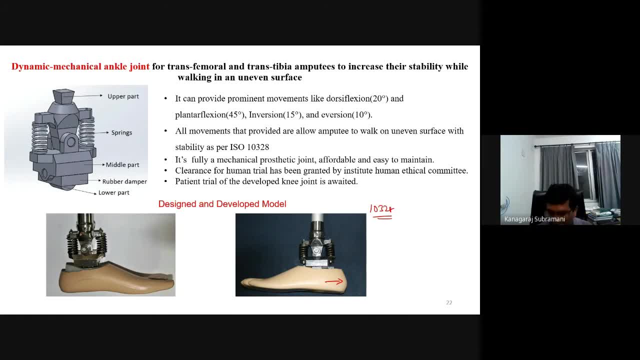 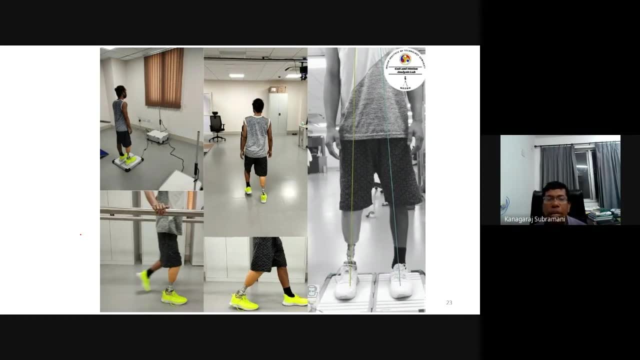 without uh or a rigid ankle joint. this is the ankle joint we are giving, only for the bologna amputees. okay, this is what you can see. we have fixed it and uh, we have tested it, for we gave it for two patients till now. another patient is waiting. okay, after the 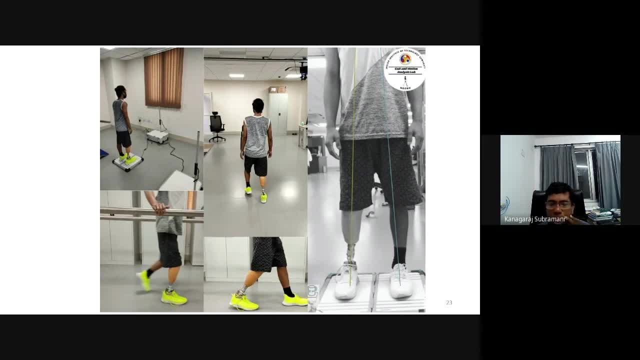 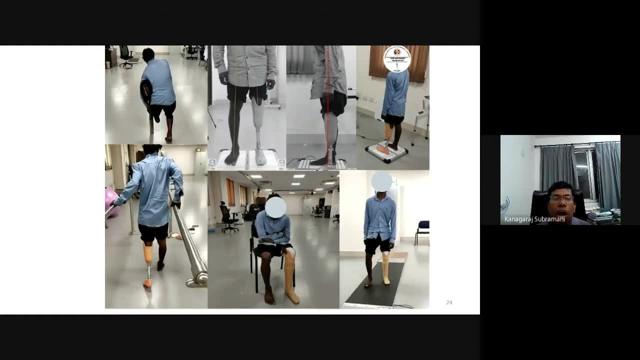 alignment and walking. you can see here that knee flexion extension, plantar flexion, dorsiflexion is very much helpful for the subject okay, and- and this is for our gator facility where we can use it, and all okay for this person, as he has been using it for a long time. so that's what we have. 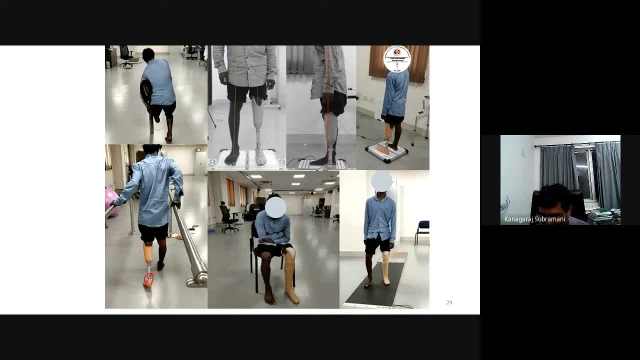 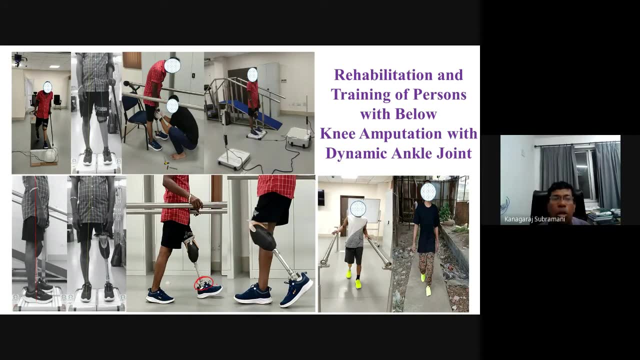 used only the fixed one, okay, so at least he could walk comfortably. gate analysis and this is for the dynamic ankle joint you can see here. okay, in this for walking and alignment and fixing and in walking training and all in that gateway and he it is in that normal his workplace okay, and he was feeling. 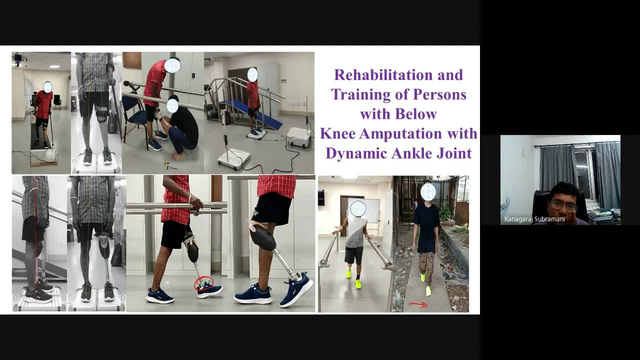 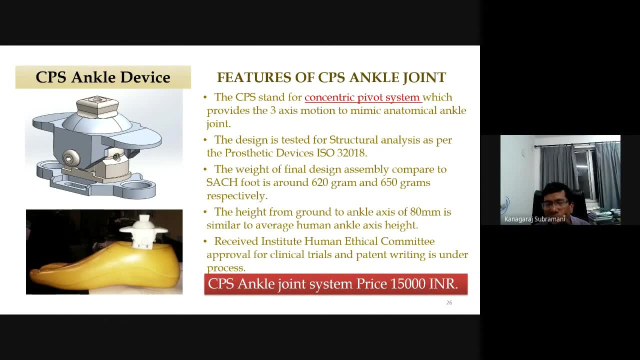 more comfortable with that, required dorsiflexion, plantar flexion and all like that. okay, this is another type of ankle joint. we are also. we are working on it. it is a different type. okay, in order to reduce its weight and all like that. this is second state. 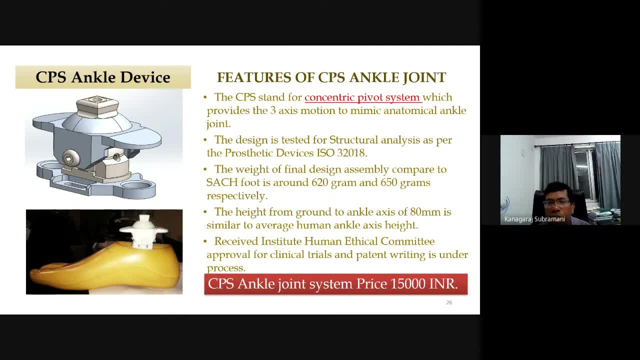 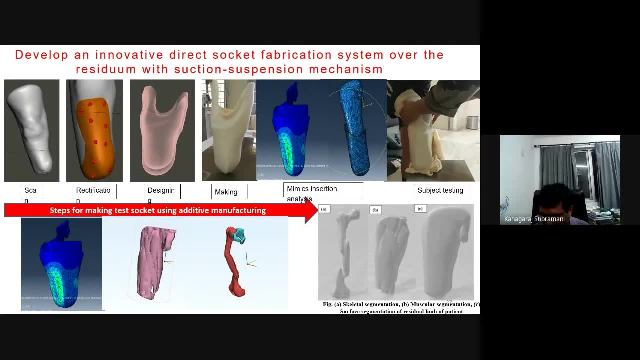 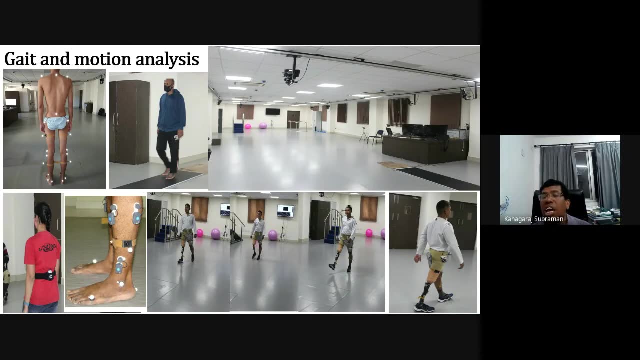 okay, so we will be working. that's what it is: a polycentric concentric pivot system. it can. we are working on it. this prototype is only being made. oh, sorry, okay, and this is what that gate lab where we are testing that, testing our subjects. okay, here we have a eight IR cameras. you can see here eight. 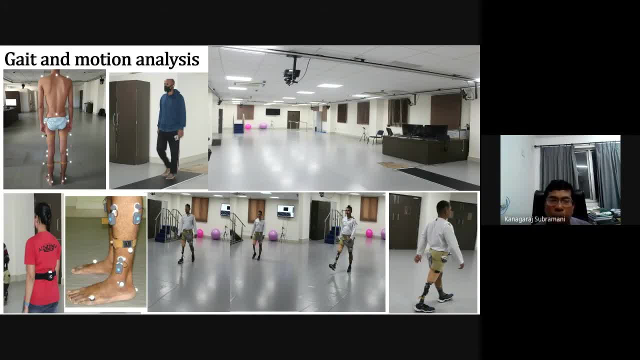 IR cameras and all that. biomarkers will keep it and all kind of a range of motion of a different joints can be studied in this. okay, so different kind of musculoskeletal disorder can be identified and this is a pressure mapping unit so we can have a different kind of a food disorder that 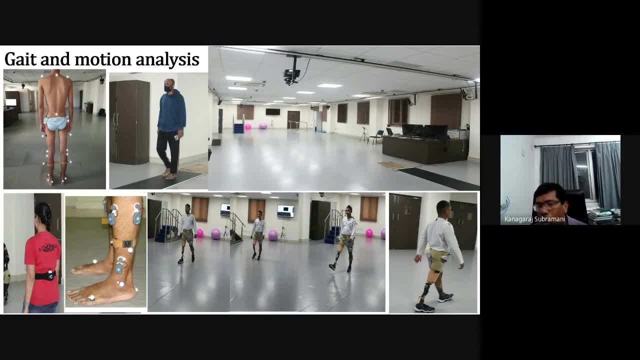 could be identified. so we, once we identify the problem, then we start to work on those assistive devices so that they can have a good quality of life. and after fixing it, that's what we do right: the rehabilitation and all like that: alignment, rehabilitation and all and this muscle. 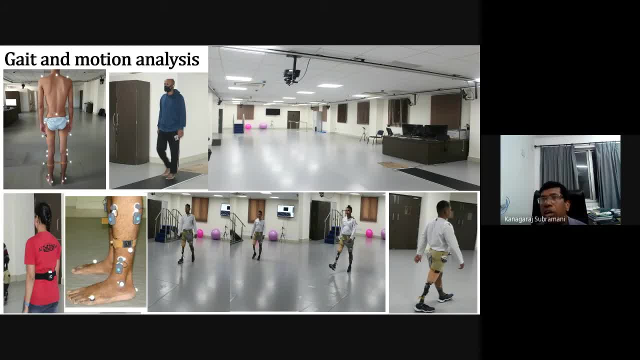 activity also we can measure it. suppose the person is coming with uh, uh, what you can say, uh, back pain and all like that. which muscle is exactly need to be addressed in order to give a muscle strengthening exercise so that his back pain could be reduced? and here, the calf muscles. 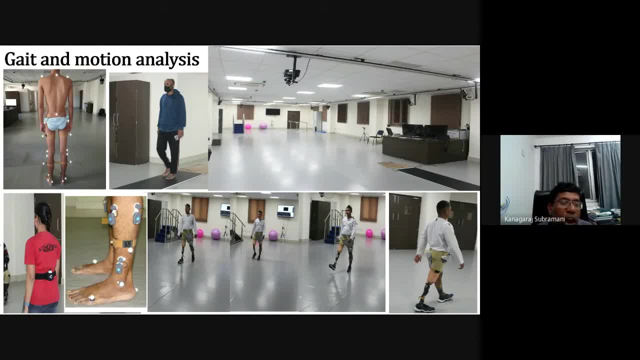 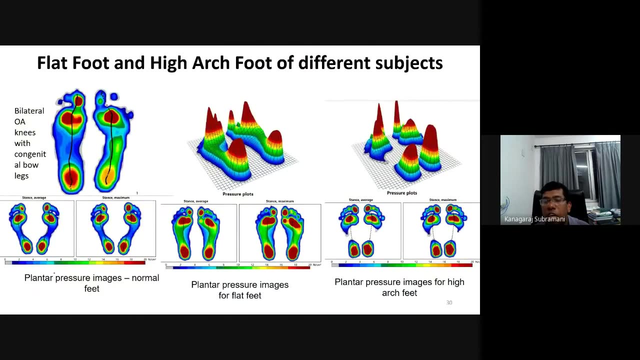 and all that's what. so, muscle activity, okay, EMG sensor and this is that. uh, this is an instrument. this one is the accelerometer and the gyroscope, so you can have a special temporal parameters and all like that. okay, this is what it is in a variety: Gohati, which is being used for our rehabilitation purpose, and all. 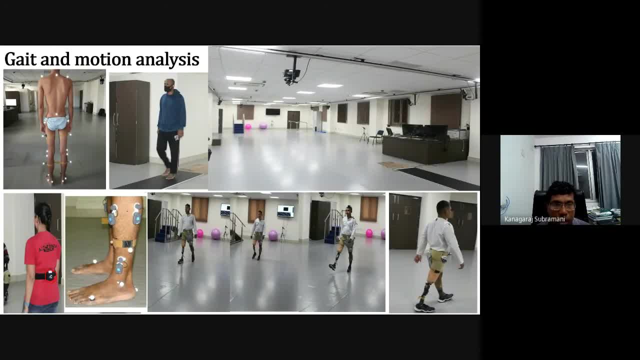 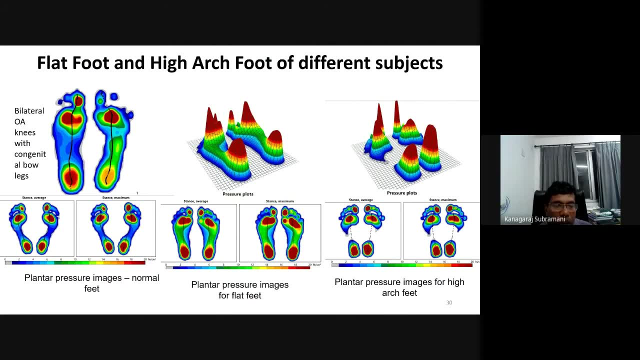 like that, and this is one of the applications of the pressure mapping unit. you can, as said, you can, have all kind of food disorder. you can see here, this is for normal food. okay, this is in a heel position, this is a metatarsal and the toe: okay, it will be like that and, if at all, the flat foot is. 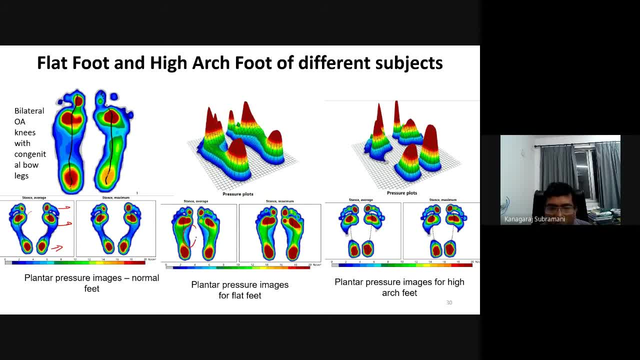 there, you can see, in the middle portion, it is also in contact with the ground. okay, and it means that this the person who is having a flat foot. he cannot walk more than, if at all, he is walking more than one or two kilometer. he will be having a pain. 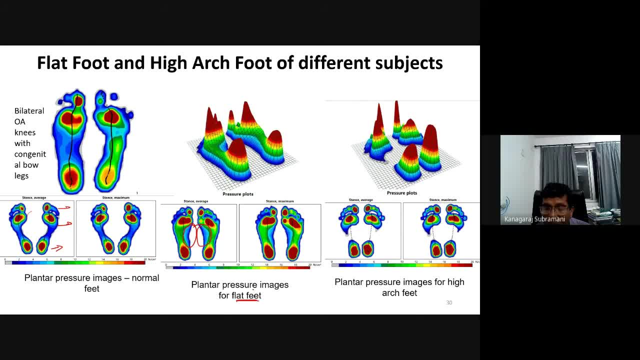 okay. so, and not only that, that, as the loading pattern is a different in a heel and metatarsal and the greater toe, it will be having some kind of effect on ankle joint, knee joint joint in a due course of time. this is one kind of flat foot and another kind of foot is cavity. 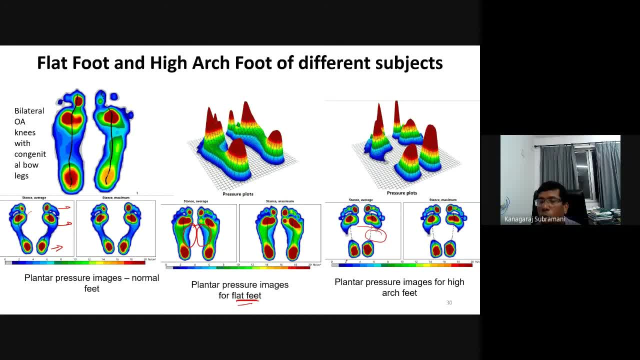 what you can say, higher foot or hollow kind of it. okay, so here, in this case it is: additional support is coming here. there is no support in the middle lateral side of the foot. okay, so just you can insert a paper in this direction. it will go and come back on another side, okay. so this kind of 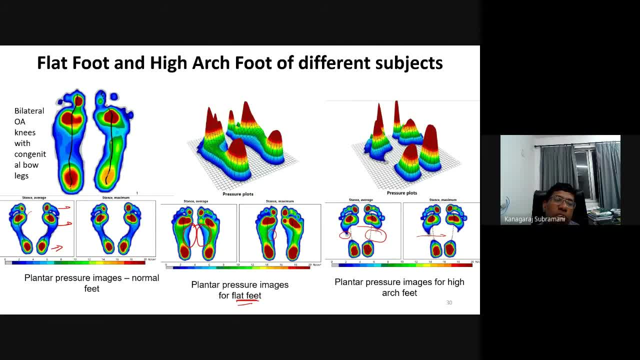 problem also can be addressed. and another one: suppose the person is having a knee osteoarthritis. okay, so in this case I can see here they will ask the knee having a problem, or the? uh, just tell me foreign, foreign, okay, so that, uh, wherever osteo pain is there, then they will not put a much load on it and they will. 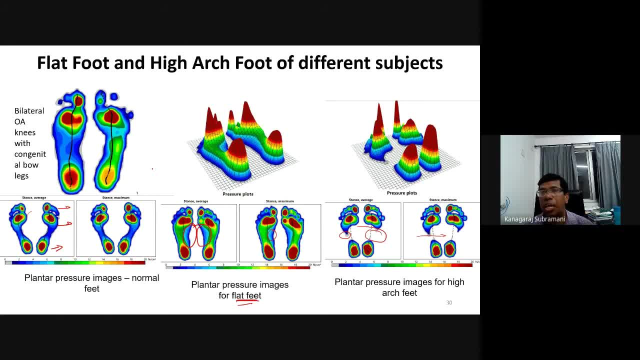 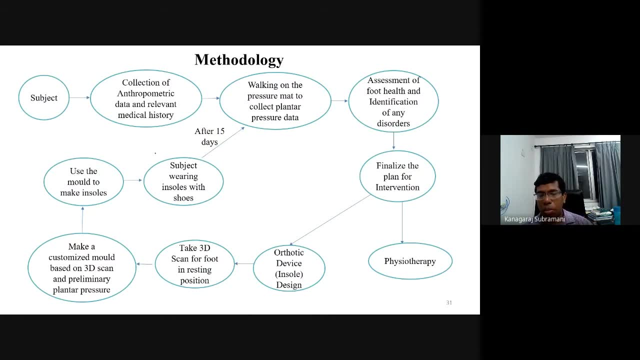 be adjusting and taking additional load on the other knee. okay, that's what. the pressure pattern will get deeper. by identifying it, we could correlate with the x-ray or MRI. we can identify. this is what what we are working on. it okay that when the some subject is coming. okay, so what kind? 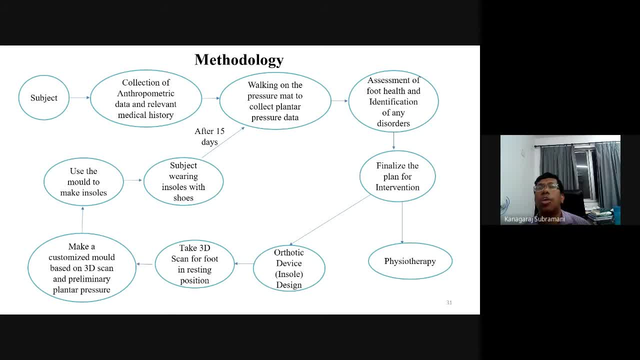 of plan. we do so that that the device can be developed for them and all like that. so when the subject comes, we collect that anthropometric data and we used to ask the stored subjects to walk on the pressure mapping unit. okay, and what kind of a disorder it is there we can identify? okay, and based on that, 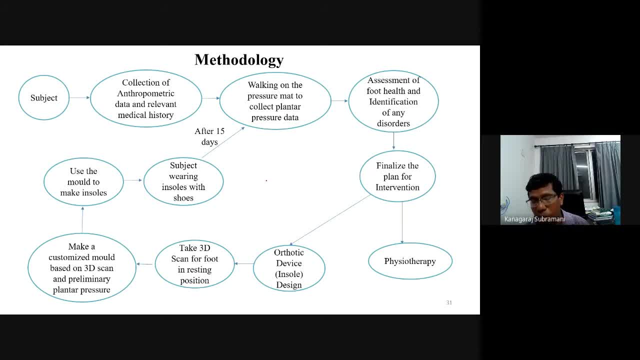 what is the problem? once we identify the problem, we say in our lab we have one of prosthetist and physiotherapist. okay, so we they used to make a report and that will be passed on to the orthopedic generally. our, we will be. 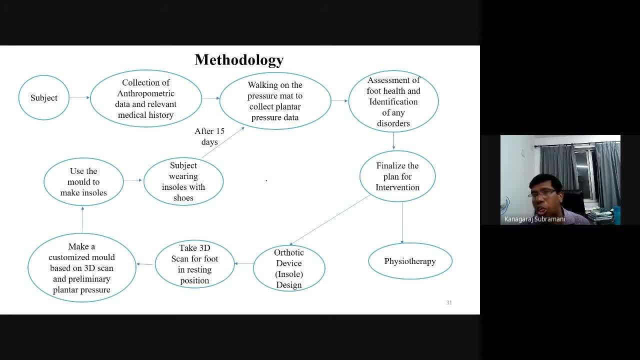 referred with. the patient will be referred by the orthopedic surgeon only. we will be forwarding the data to the subject as well as that orthopedic surgeon, and they will be doing another follow up and all like that. okay, that's what. otherwise, if you need to do some kind of orthotic device, then 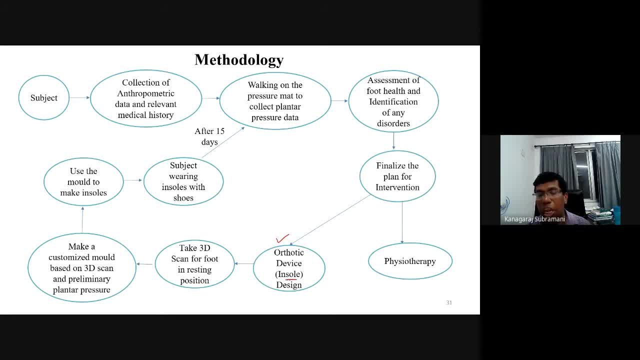 it will be mainly that for all the flat foot, we are making insulin and all like that and we will be taking a 3D scan and of the foot and we will be modifying it. we will be making a 3D mold and we will be filling that with a metamaterial, auxetic based water. 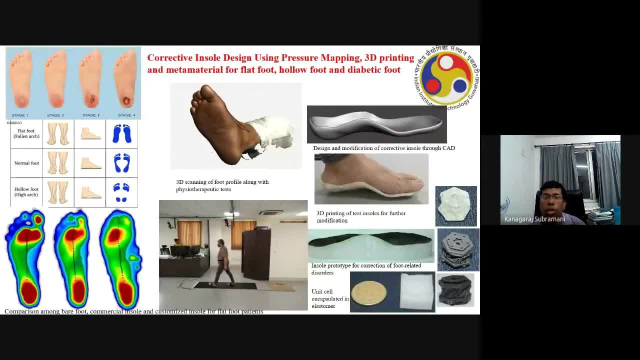 on and we will be making a linsole and we will do that study and all like that. okay, this is what that study? okay, and uh, we will be getting a 3D, uh pressure map. that is, 3D scanning of the food. okay, exact food and navicular test and all we will do entry test, okay, navicular drop test and 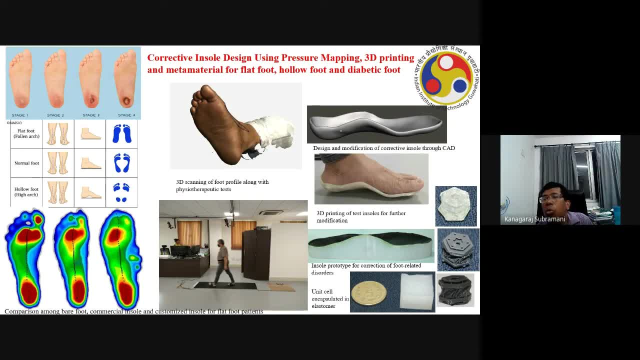 how much we need to adjust it. and after that, once we make it, then we do adjust. we need to give wherever support is need to be given. we will be making that CAD model and this 3D printed test model. we will be using it. this exactly then. after that, we will be making a mold. okay, and in this one, 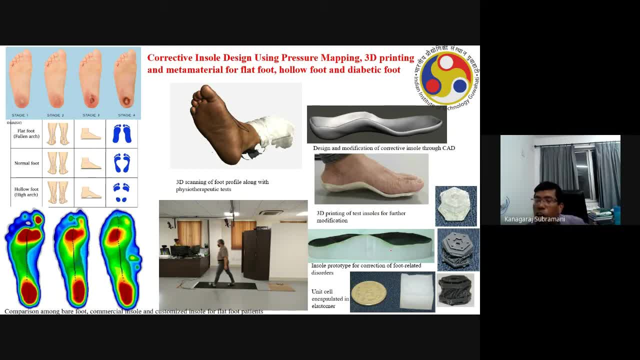 we will be filling it with a silicon line. silicon, we will be filling it in the mold and we will be getting the liner out of it. and wherever we need to give a preset distribution or this, what that unit cell? okay, we applied for patent. also okay with the tata steel, okay, and this will be placing. 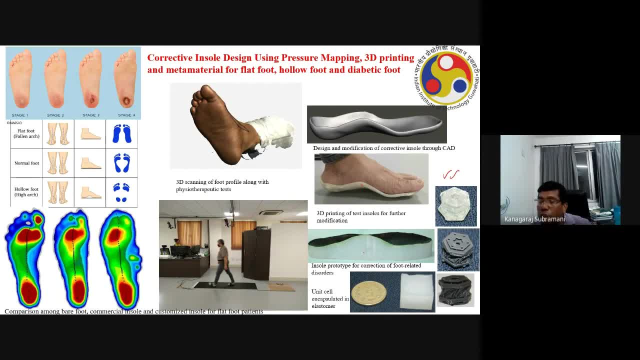 it in a different position in order to ensure, in order to give a support or the preset distribution. okay, then after that we will make the insole and that will be tested with a subject and in due course of time it will be giving a support so that a pressure distribution will be uniform after due. 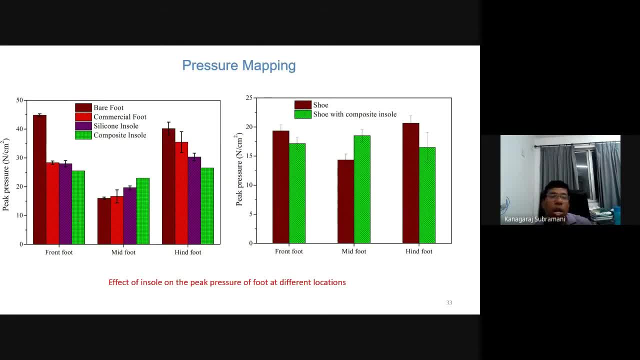 course of time. okay, this is what, what we have tested it okay. so you can see, here in a mid food we could give a support better than a normal case. okay, and in addition, at that heel for hin food you can see that pressure reduction and front foot or the metatarsal also, you will pan that pressure reduction at all. okay, fine, so wherever. 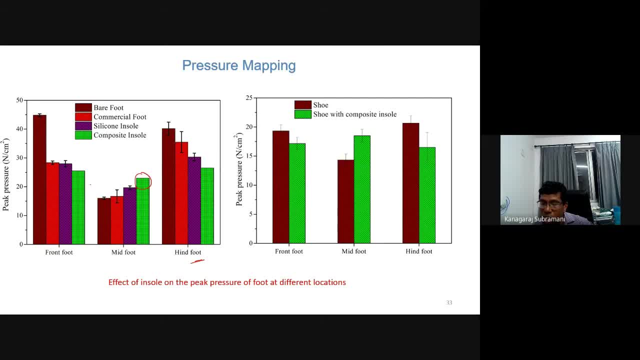 the pressure is need to be released or wherever that support needs to be given. we could confirm it in our study and all. okay, this is with the shoe and this is showing so. okay, with the composite insole and all like that. in the front foot we could reduce it and with foot, we can give a support. 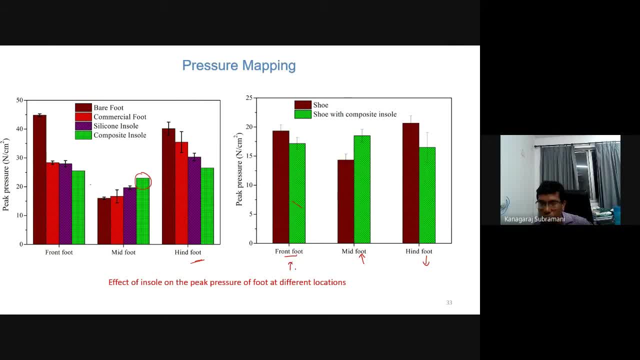 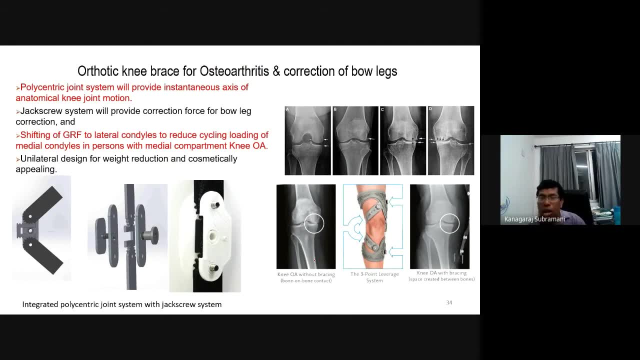 and in foot also, we could reduce the load. that is what. sorry, here we will be reducing the load, okay, and yeah, uh, how much time do i have double teenage? yeah, you can carry on. okay, fine, fine, fine, fine, okay. so this one. another one is: this is one of my. 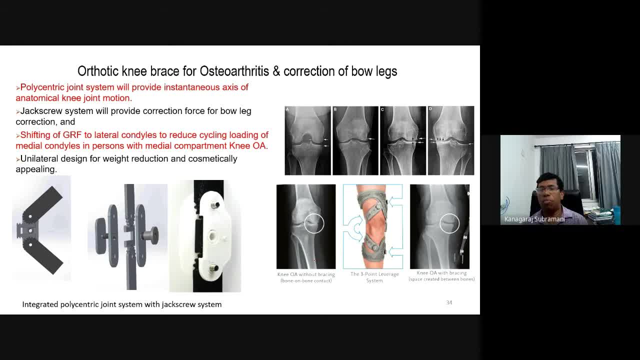 uh, what you can say. prosthetics. along with him, we started to work on it. this is the knee brace. okay, this is what, what commercially available three point river system. okay, so, and it is about a near about 40, 40 to 50 000. it is okay. so we wanted to develop a somewhat. 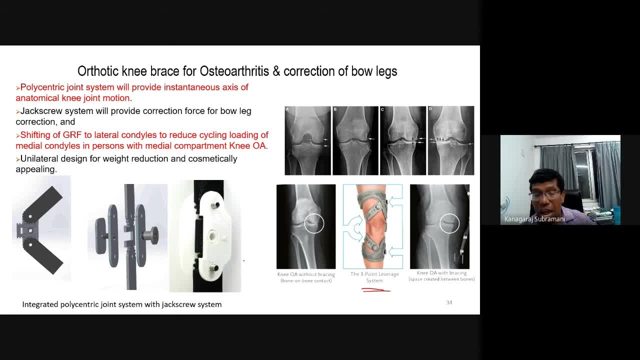 affordable material, a bit of affordable device with a simple the polycentric jack screw system. okay, so here also what you can say: once you apply load in both side there will be a reaction. okay, so due to that reaction, then the gap be in that middle side could be red. 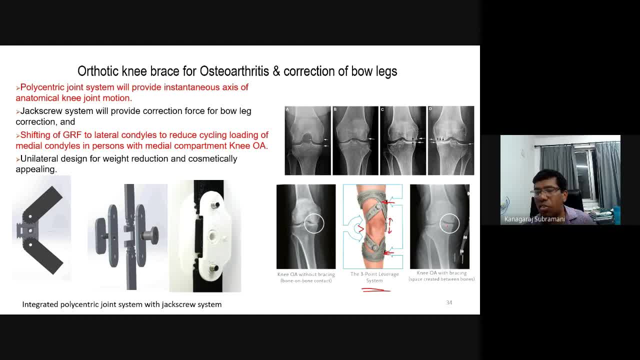 increased. otherwise what will happen in this case? that distance will be very small. okay, or it is in a contact. if you use this kind of that screw system, what is it? what is a new brace? we can unload it, if at all. we could identify this problem at that stage one or stage two with if his personal subject is: 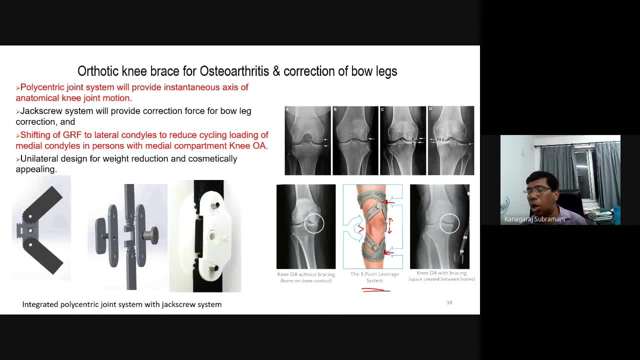 using this kind of a new brace is shifting that load. okay, we can shift that load from middle side to the lateral side. one way we are unloading the damaged part in most of the time. if you see the literature near, about 80 percentage of the subjects are having most of the damage in the middle side. 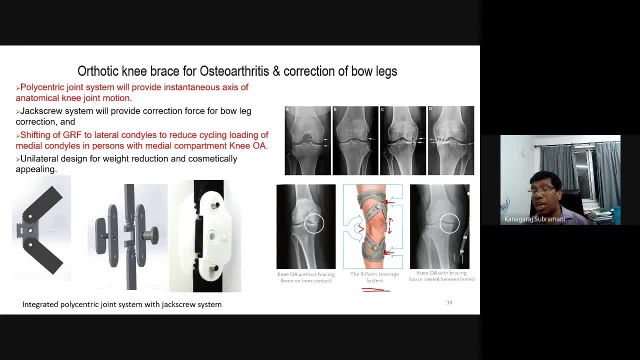 okay for time being. if you shift that, if at all, that problem is identified at a very early stage. if you shift that load from the middle to the lateral, there are two advantages. first is you are not loading the damaged part, so it is getting unloaded, and second one if it is. 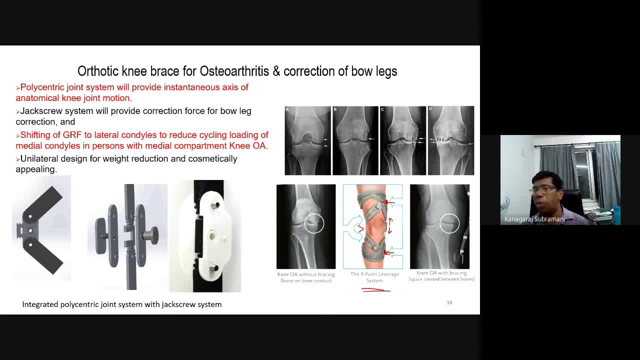 at the preliminary stage, that the cartilage cannot be regenerated, but up to some level, because the people are using it as gel also. okay, so it will help to regenerate the cartilage, that also with the certain level of that damage, so that also we can explore so that, uh, that cartilage will. 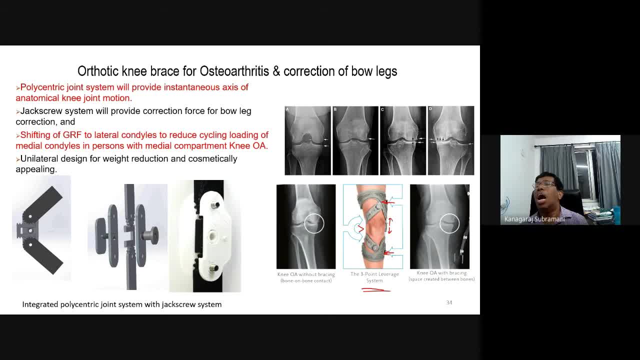 come back to the original shape and size. okay, and if at all, in both cases it is there, then the knee brace can. in this case, it is not a load bearing component. okay, it is just. it will give you a load bearing component. okay, it is just, it will give you a load bearing component. okay, it is. 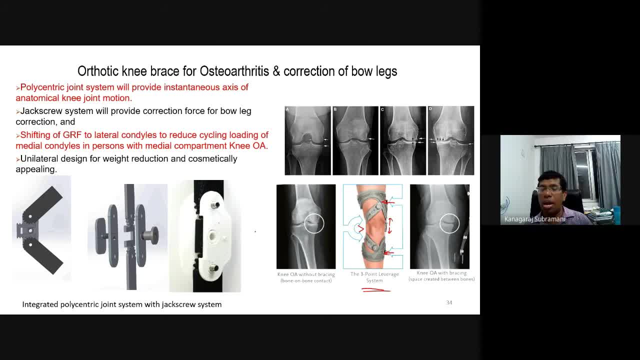 a reaction force. if it is made in a load bearing, load transfer, then we need to use a two knee braces so whenever that ground reaction force will not pass through that knee which is having a high end of osteoarthritis, this can be explored for a person who is not willing to go for. 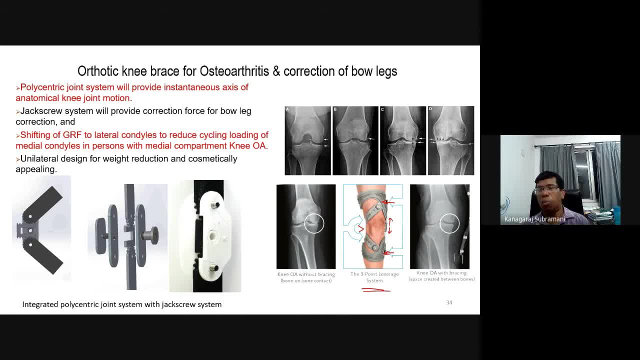 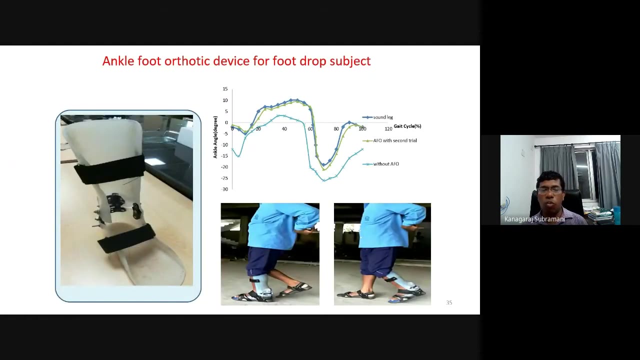 knee replacement surgery or he is unfit for the surgery. in both cases, that low transfer mechanism, it is a orthosis. okay, so you can use those device at that outer outside so he can go for at least normal day-to-day activities. he can do this. is that only at the preliminary stage of our development? okay, and this is a for food drop. 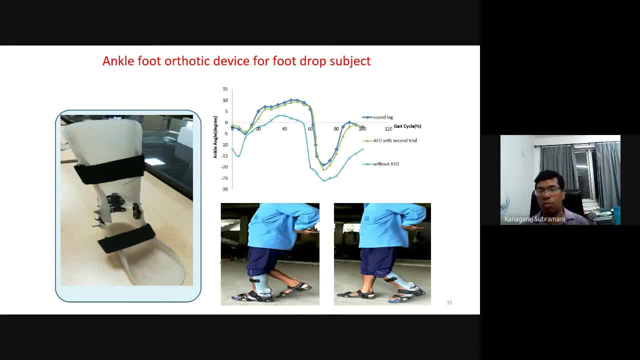 people. okay, so this is what he was: just a flat uh, just with the what you can say, and plantar flexion is not there as soon as he touches, then it will be suddenly a little bit off. so in that existing orthosis we have made a spring control device so that load will. 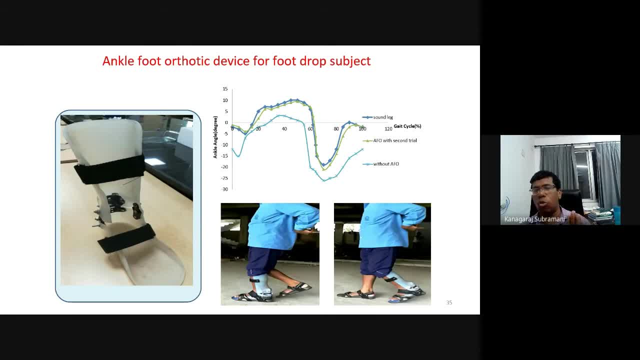 be, the energy will be stored and it will be released, so we'll be having a proper plantar flexion and a dust reflection. this is what, without afo, and with afo, which will be having us at par with the sound length. okay, this is what we have used, it also, and he has been using it, and most. 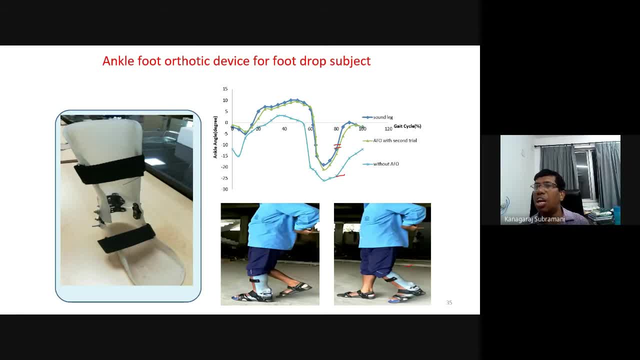 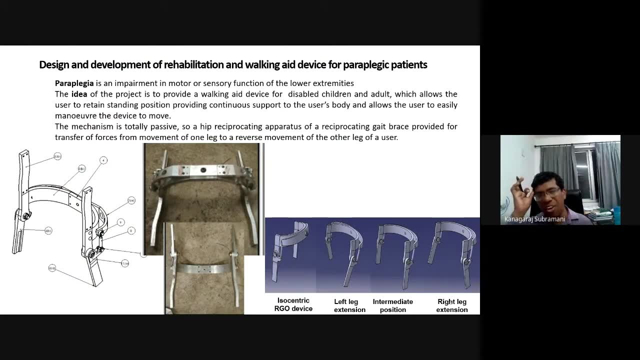 of the cases, all that assistive devices, what we are working we are giving to the subject and they have been using it. okay, it is okay. and this is another device. we have developed it. we have not even tested for a subject, it is for a parabolic equation. okay, so below that waist, their leg is not. 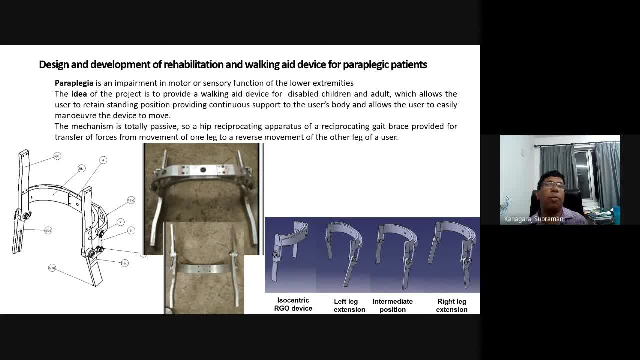 working. okay. so, however, they can rotate their body- okay. so if they could able to rotate the body, this one, this in uh reciprocating orthosis, we can. this rotation motion can be converted into leg movement of it. that is what we have made it there. okay, uh, here we have that modular version so that, whatever 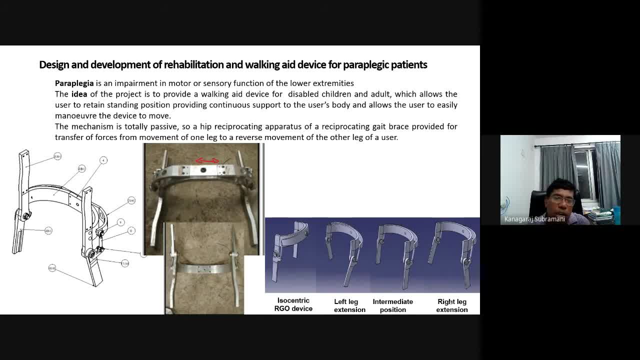 waist size. we can reduce or you can increase it and all like that. okay, we have made the product and that we are not getting that the patient for whom we designed it and, uh, he is not returning. that is what we get to do. that is what. however, we have made the modular version. okay, that all. 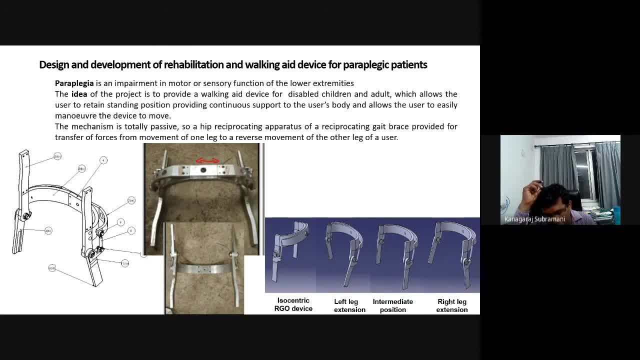 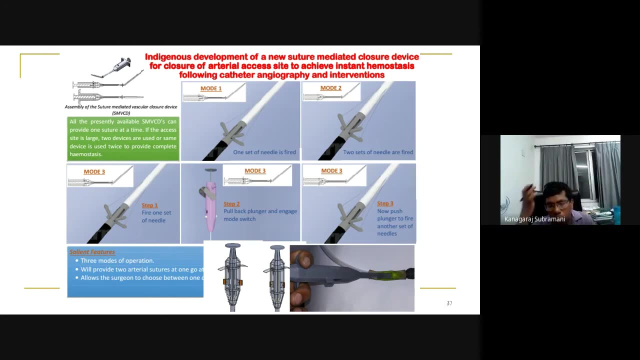 that hip joints and all like that, everything we can make. made it, we have made it and it needs to be tested with the subject. mainly it is a reciprocating orthosis, mainly for a parabolic, and another one is a suture mediated closer device. okay, so this one suppose. when a doctor 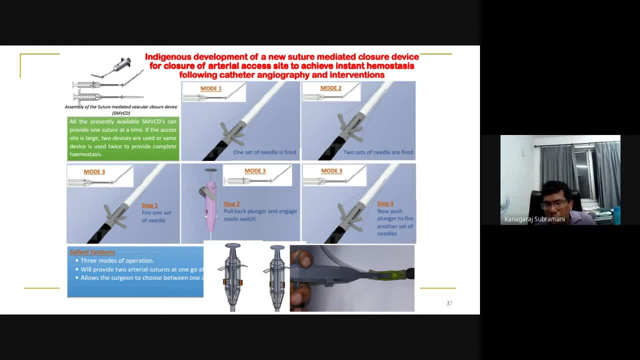 is doing a minimally invasive surgery when they are making a puncture in the femoral artery. if it is a 4 mm size, then there is a lot of devices for the even one, perclose, proglide and all like that. with a single device they can close it. the diameter of that puncture side is more if it is 6 mm, 8 mm. 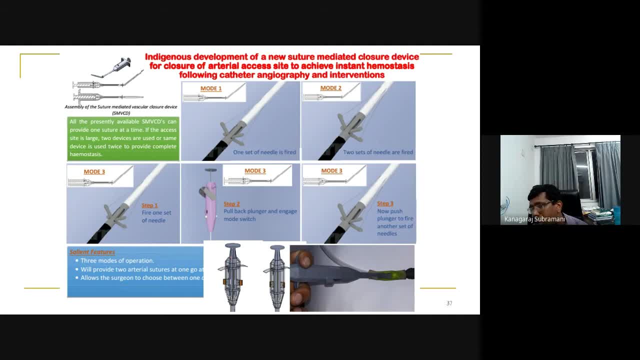 or 10 mm if they are making it because of that device, whatever it is going to be inserted into a femoral artery. so depending on the size they will, puncture sites will be increased. in this case they need to use a one, two device or three device to close the puncture sites. 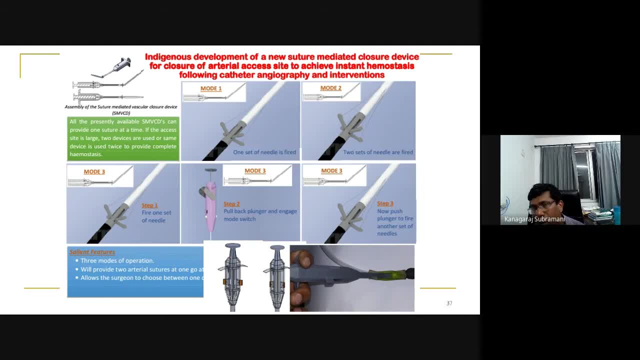 okay, this problem was given by radiologist, interventional radiologist at negrin. so what, we have made it with a single device. we can have a two set of needles. it will be working on a three mode of up, three mode of operation in a one mode. we will inject, we will fire one set of needles. 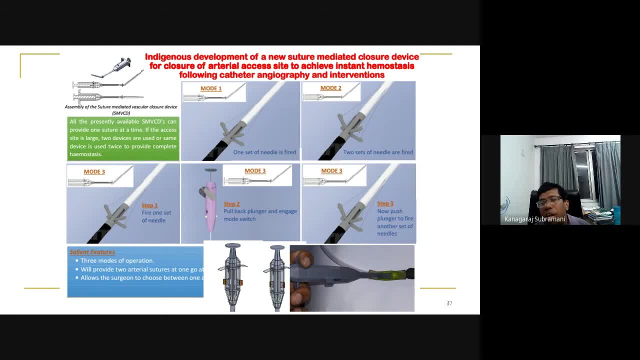 okay, and in a mode two another set of needle will come. it is that when the doctor can choose when he need to operate the mode one, when he needs to operate the mode two, if you want to fire both the needles together, then he can have. okay, in this case, the mode two, both the needle set will be. 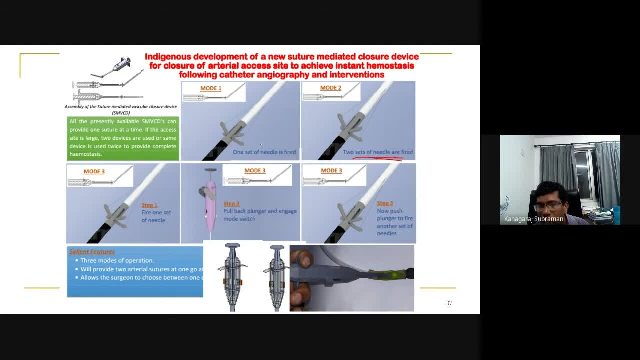 fired and in mode three, first one, he will be using mode one. then after pushing back, then there will be engaging mechanism. then another set of needle will come, so you can have a tenor set of needles, four o'clock lock as well as eight o'clock two o'clock clock, so you can have that kind of. 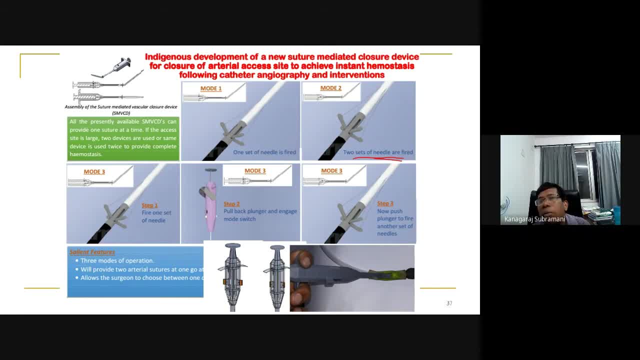 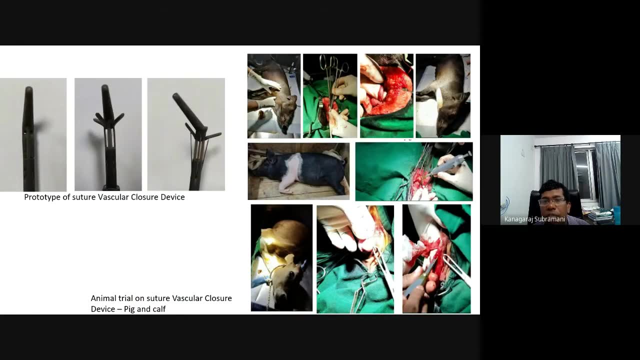 you can close that puncture site. okay, up to eight mm, up to 10 mm and all like that. you can close the puncture site. this we have made the device and we tested it in a three different animals. okay, and what you can say, this is small, two picks- we have tested it and one top- we did it also. 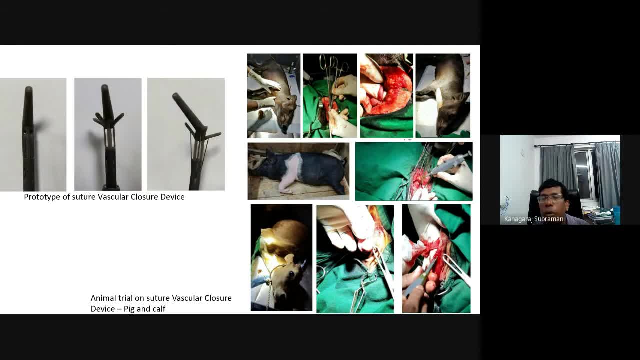 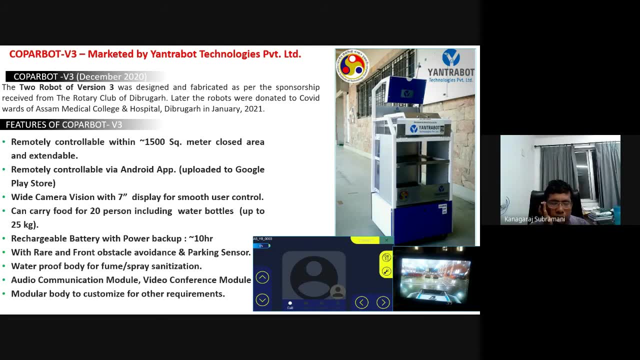 okay, we need to. that's what the status right now. okay, and this is the one. now, what you can say: one and what you can say: uh, one, uh, assistive device, the assistive robot, okay, this can deliver during that corner period. we were asked, we, they are asked, to design and deliver that one. what you can say: drug and food. 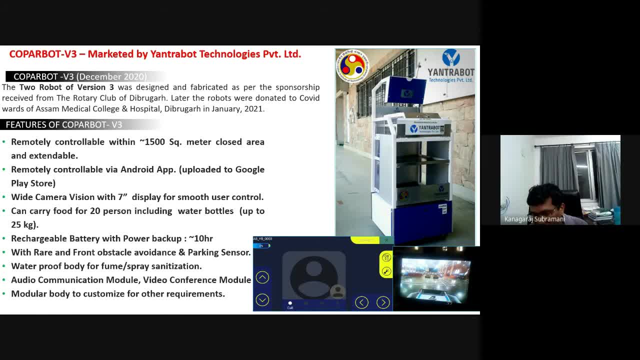 delivery, making food delivery device in, uh, what you can say- in isolated water, okay, and this, what with the one come, we have made it. and one company with yandra boat is the startup company at iat go hardy. okay, we have made it and it was given. also, you know when that uh, then uh, chief minister swan, dr uh swanabal, mr swanabal he. 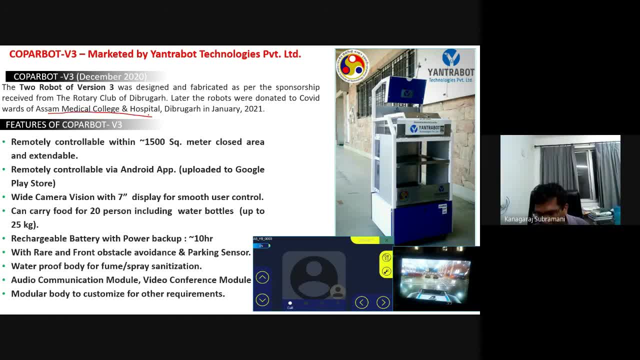 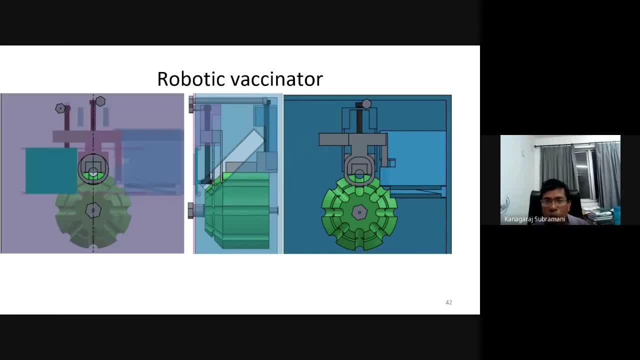 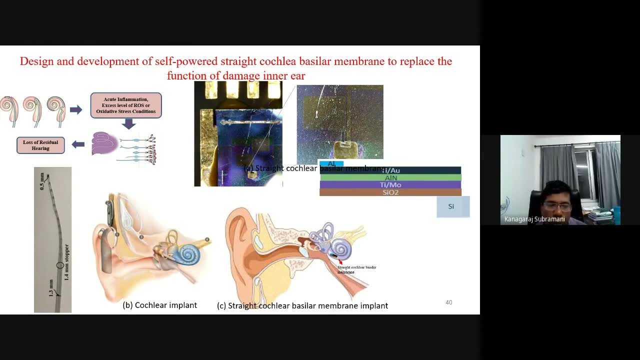 has given to that as a medical college in 2020 last year, and a lot of this is third version of it. okay, and this one. before i conclude, there are two more devices, not more than that. okay, so this one, uh, this is what. what you will be finding it in an existing coupler implant. okay, in the existing coupler implant: this. 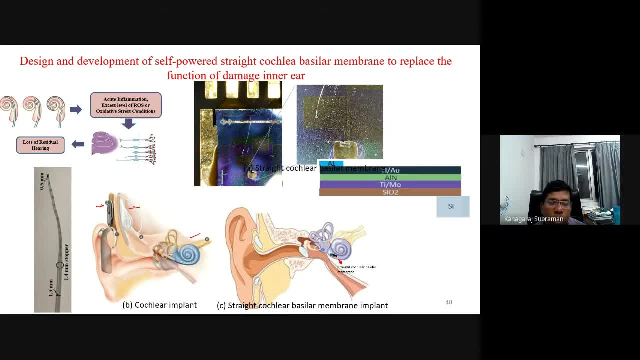 external device and this is the internal device and it will hear that sound you can hear and it will be getting converted into electrical signal and this is a radio. it will be converted into a radio frequency and here inside you will have a receiver. it will receive it and it will convert. 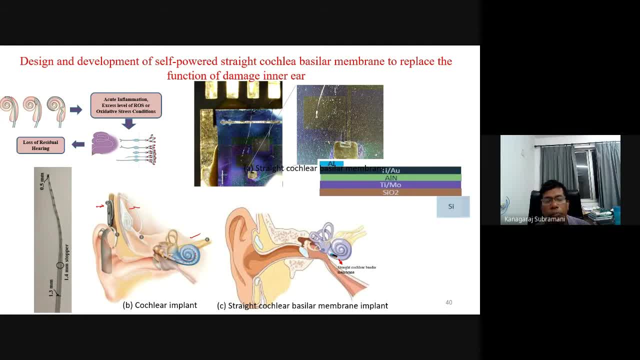 into electrical signal and that pass on to the cochlea. in this one we are working on many attempts, okay. first one is: once you insert that electrode into the system, what will happen due to the surgical procedure? there are a lot of free radicals, okay. reactive oxygen species or species. 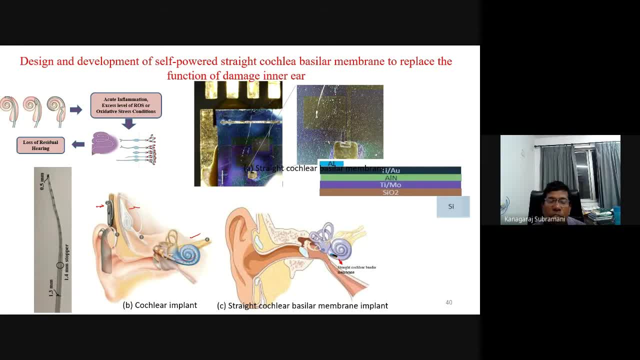 are large amount of it is coming, generated that will kill that residual hearing of it. okay, so that, uh, some kind of a radical, sorry, scavenging unit, hydroxyl scavenging, meticulous, and purely this nanomaterial. okay so get to see cerium zirconia material. okay that we have used it. 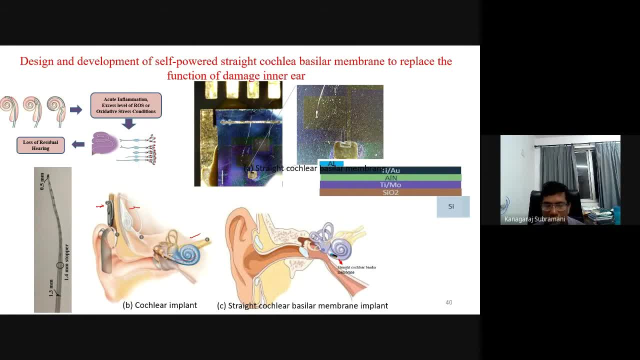 to scavenge those excess generation of hydroxyl radicals that will help to preserve the residual hearing. that is one, and we have tested it, that up see that cerium zirconium, whatever we made it, that we have tested it in animal and even subcutaneous and percutaneous and all, and we have confirmed that hydroxyl radicals are. 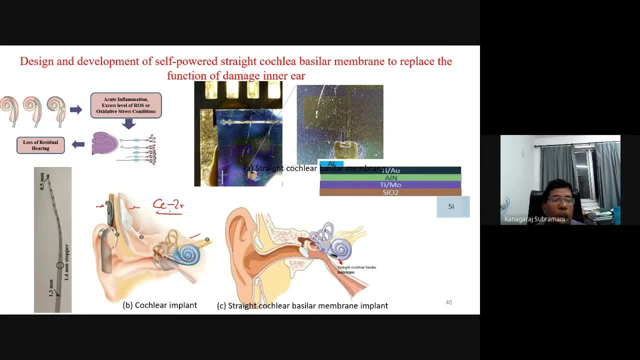 controlled significantly, okay. and another one. this is that in this is that cochlear implant, and what we have proposed is a piezoelectric sensor. okay, this is what that aluminum nitride, with a different layer of what you can see. it is a different nanometer level thickness, okay, and a different. 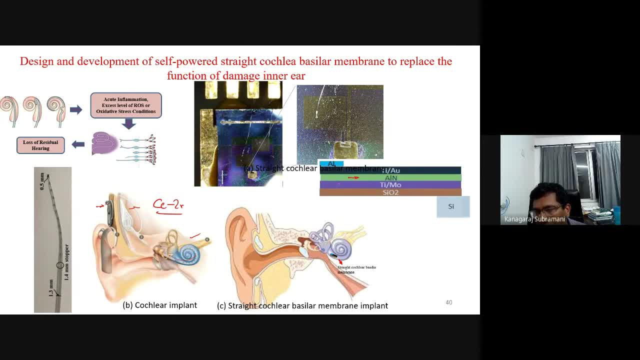 length. also, it is a cantilever beam kind of it, and this is a piezoelectric material and this is the substrate and these are all connecting material, okay, and this is what somewhat uh, balancing one, okay. so in this one, what we have found is that 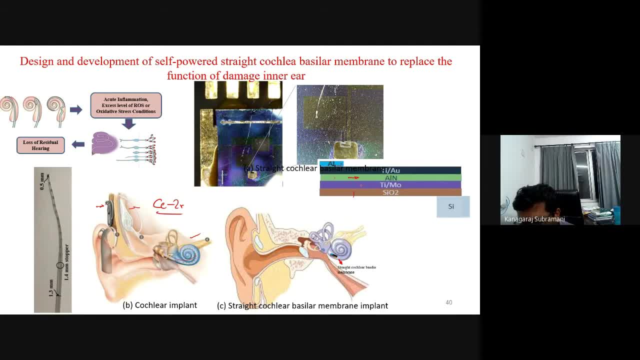 this is a piezoelectric sensor. okay, it is in the range of maximum of three, uh, three thousand micron. okay, that will be, and this will be light up at, so many cantilever beams will be made and it will be connected depending on the sound wave pattern of the particular subject. after that, it will be fixed. 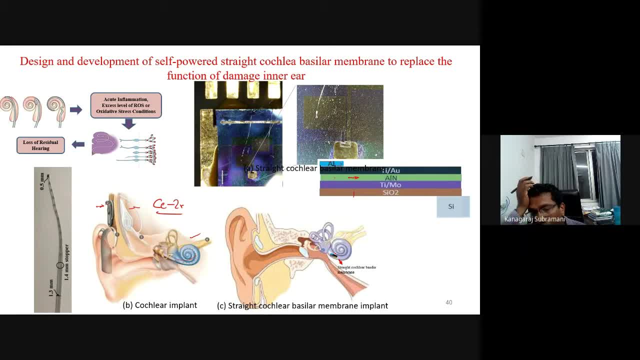 within the cochlea, near the ground with- okay, sorry, near the mobile window. and this is our hypothesis right now. we have made that sensor and our in vitro studies are going on our hypothesis that this: once you fix this piezoelectric sensor inside the cochlea, so here in this case, 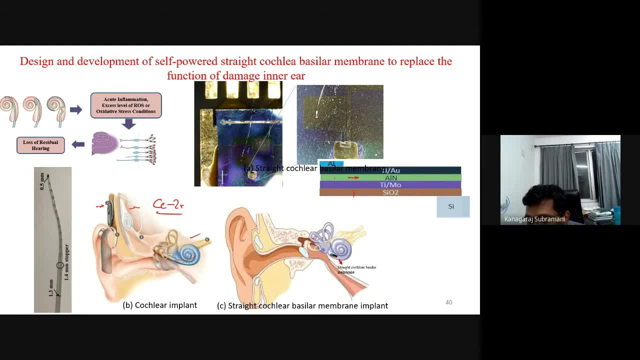 here in the outer ear is working and the outer area is working, middle ear is working, so inside that waves will be getting a transfer. this movement will be transferred in the, in the cochlear fluid. it is nothing but a phosphate buffer solution equivalent. so this waves so as it is a piezoelectric. 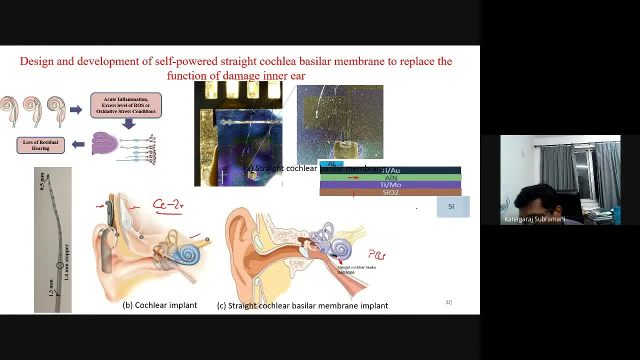 metal it will give the pressure wave will be transferred to the piezoelectric metal. it will give that a signal, so that signal will be passed on to that nerves and it will go to the brain. so in this case there is no need of again that outer air, outer. 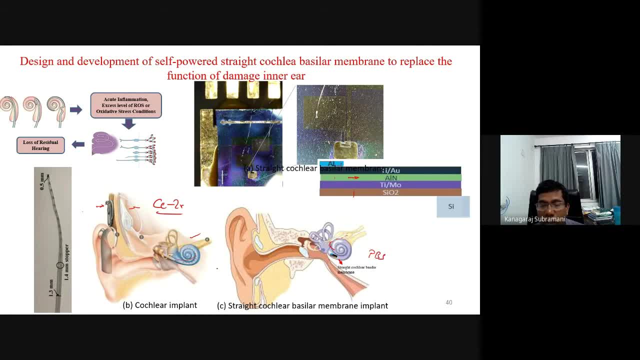 outer component, inner components, and this electrode is insertion and all like that. everything could be avoided. so this is small piezoelectric sensor that could be implanted in that inner air. that that will be auto power here also. there you no need any separate power generator, power medium, because that way, whatever it is getting generated, that will be helping to. 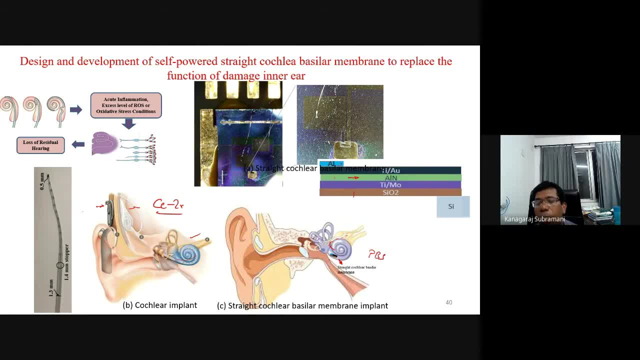 generate that electrical signal that will be passed on to that. okay, this is what, what we are working on it, this is what what we have already made it okay in ISC Bangalore, and now we have developed that in vitro test setup and we are working on it. okay, that is what it is, maybe that. 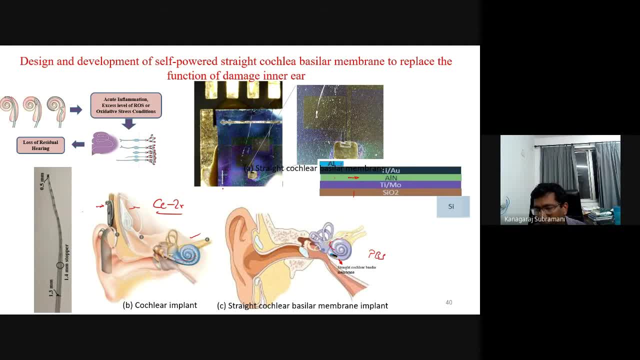 as it is a that length is 300 micron and that thickness is. length is maximum is 3000 micron, that is 3 mm, and thickness is it is about 120. it is around 120 nanometer and these are all around 30 nanometer and all like that. that is what it is, okay. 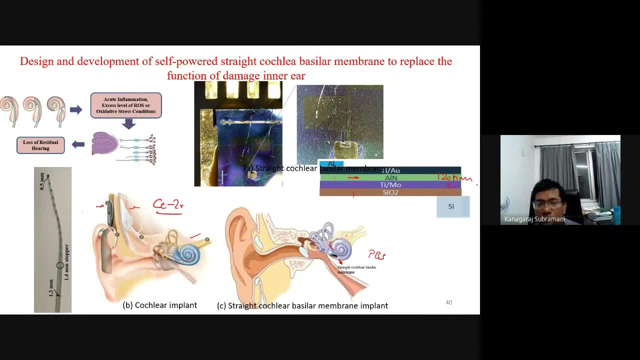 and this is what what we are working in. another one in the same, in this case, sorry, in this category. okay so, when that electrodes are inserted into the cochlea? okay so if, as it is a closed medium, the pressure, even one, one mm is inserted into that window, what will happen? the pressure is. 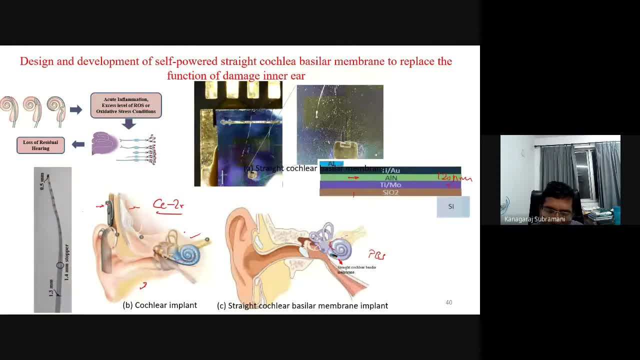 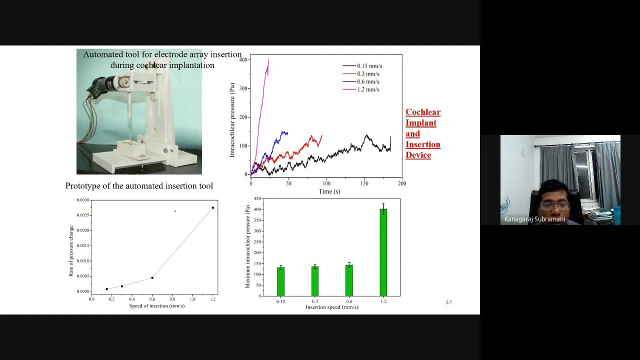 getting build up enormously, so they will insert one mm, then after that they will wait for the subsidized, then after that they will be inserting it. okay, that is what we have made it: an automatic electrode insertion unit, okay, so, whatever that speed we wanted, this is what we have made it at a 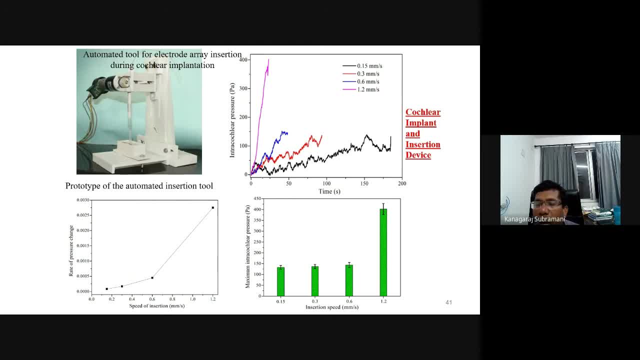 different speed level. okay, inter cochlear pressure and what level we need to insert it so that that fluid cochlear fluid pressure will not be drastically increased. okay, this is what you can see here. insertion speed: if it is there, that maximum pressure level will be around 150 Pascal. it is within that, then there will be no issue. 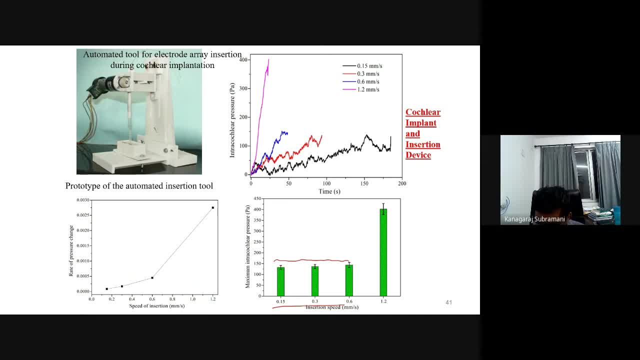 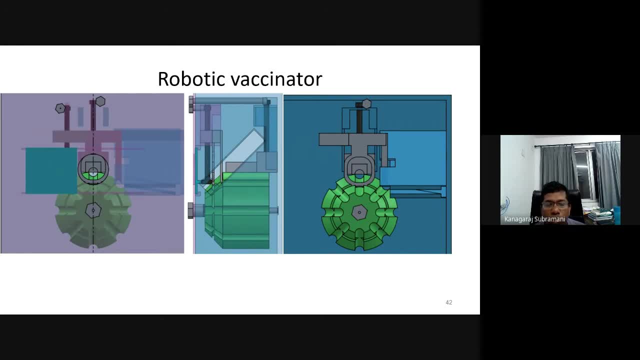 okay, so we developed that setup and we did the study. okay, and another one is last. one is okay, this one, the robotic vaccinator. okay, so, as, as you know, that you know, due to that covid and all, a lot of people are going for vaccination, okay, that is now. it is a manual vaccination. this setup we have. 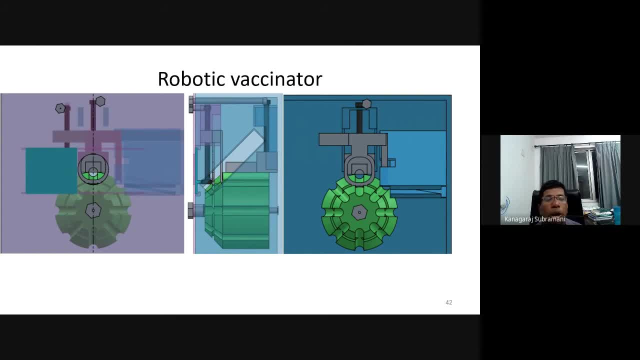 designed and developed also. okay, so, uh, this one, and in this case, what has happened? it will be automated. this robotic vaccinated, automated, and that wastage of the drugs could be reduced. lastly, okay, if they are using a or 100 subjects near about a meditation, that what you can say, that. 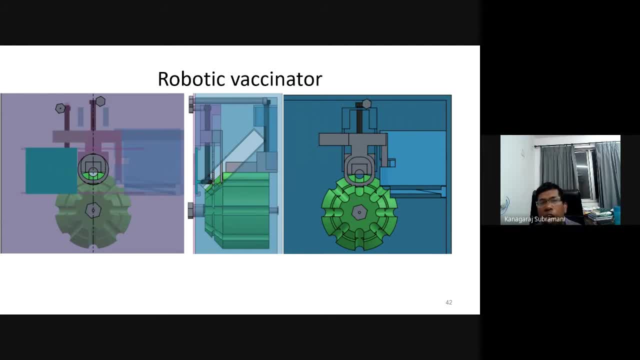 managing drugs worth of five people is getting wasted okay in a normally if you take everything. so if we could save that drug, whatever it is, medication, whatever is getting wasted okay in a normal if you take everything. so if we could save that drugs, whatever it is reducing as that, whatever it would be. 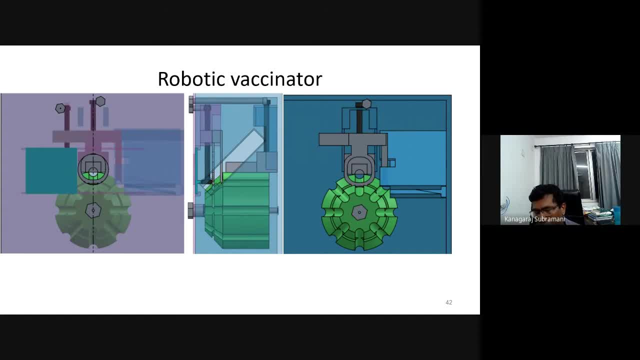 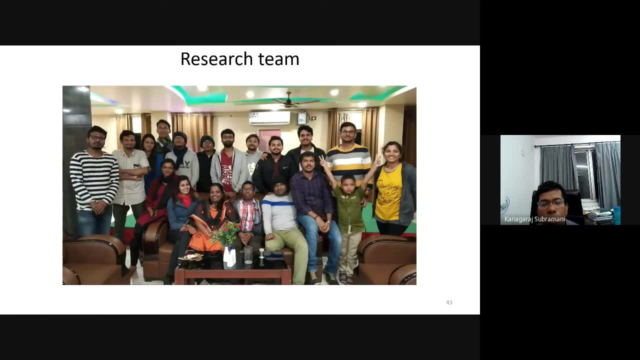 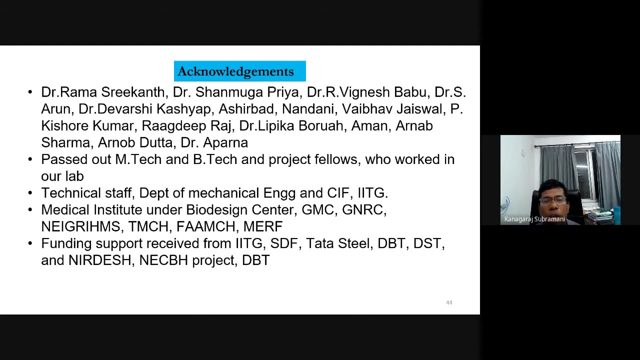 it is being used for vaccination. in addition, we could make it automatic: this product is ready, okay, just as it is industry project. that's why we put it like that. okay, this was our research team and i this. i like to take that opportunity to acknowledge all my students, phd students. 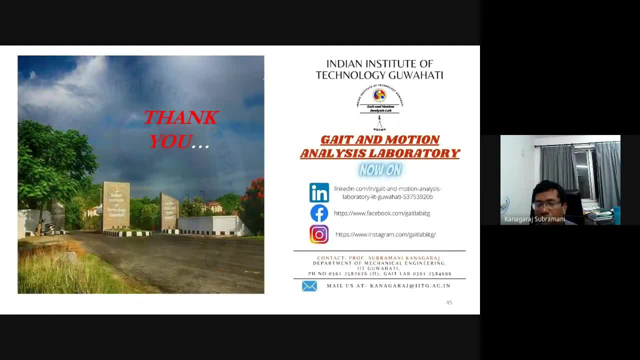 mtech students, projects and other funding agencies and all like that. with that, i would like to thank you all. that's all. this is our gate lab. if anyone is interested, they can join in linkedin all kind of activity. whatever we are doing, we are updating that. you're all most welcome to visit iit guwahati. 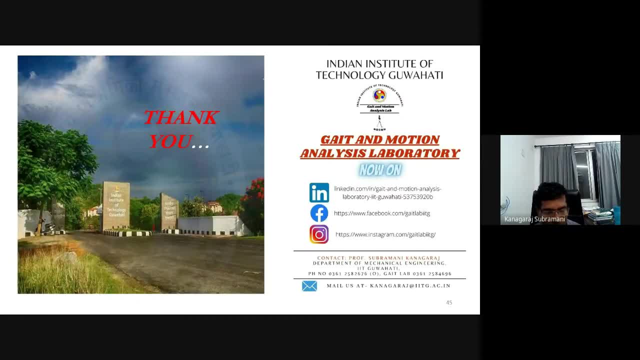 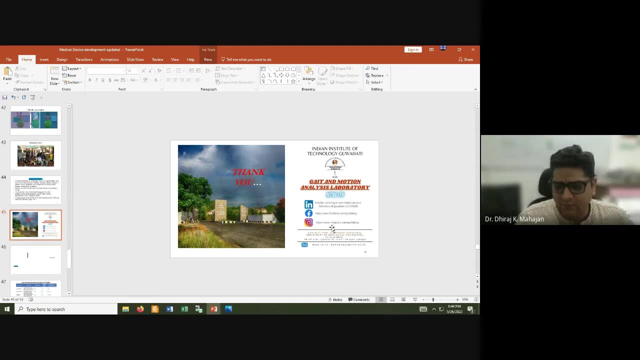 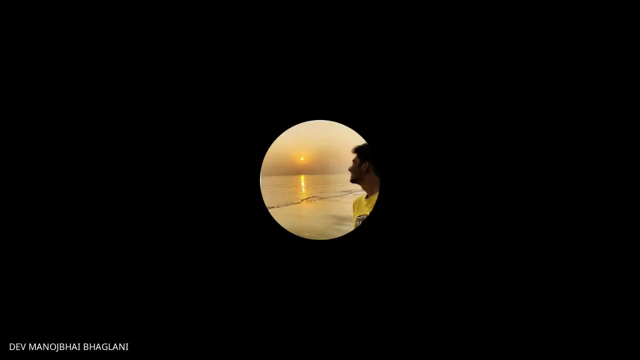 and visit the lab and visit the facilities. okay, that's all from my side. yeah, yeah, thanks a lot, sir. thanks for a wonderful talk. so, um, yeah, so the top is open for questions. yes, yes, sir, i didn't get about that leg that. why can't we use knee joint and ankle joint together? 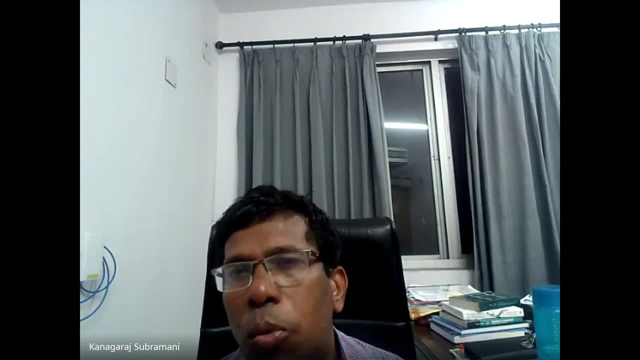 even if you talk about that ankle joint itself. we had given option for uh, plantar flexion or c flexion, as well as the inversion, aversion or supination pronation. you can say, but the patient when we are trying it, at the time only we realize that two degrees of freedom. it is not uh because 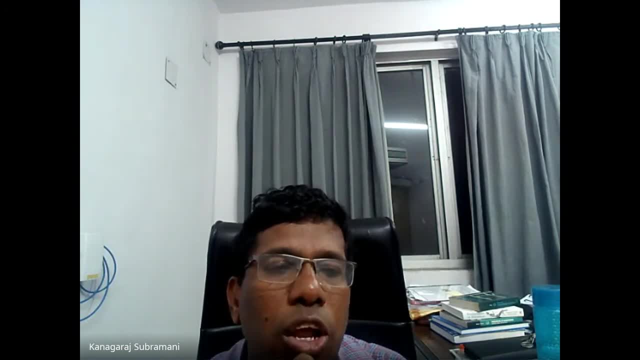 they are really in the same level of freedom as much, but still in the same level of freedom trying at first time. okay, so we have stopped them. we have stopped one of the degrees of freedom like a inversion aversion. we stopped it. we have given a provision for locking it and right now we can. 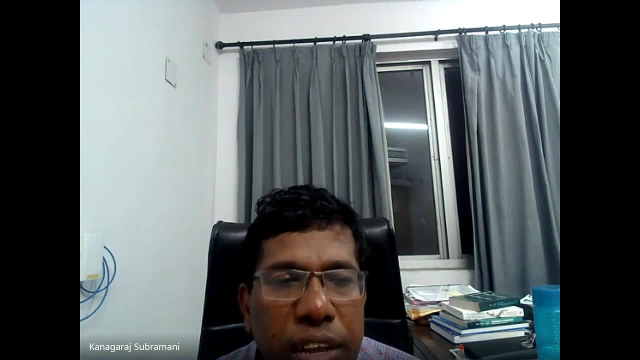 have only the plantar flexion, dorsiflexion. so once the patient is comfortable to walk, maybe after a few months and all- then we can unlock that inversion aversion. okay, that is the situation. but if you have only having a variable in that hip knee joint and variable in the ankle joint, 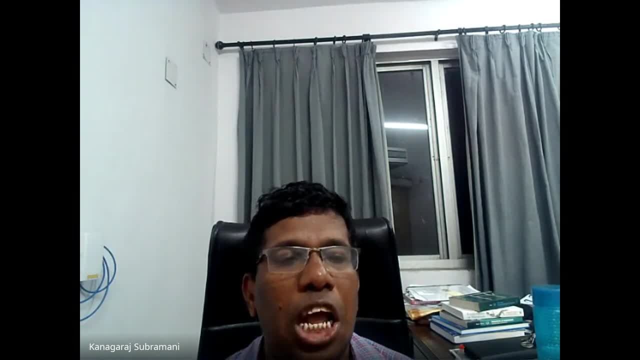 it is not at all desirable from the safety point of view, if at all it is required. there is no doubt if it will be required. but let him go with knee joint for a certain period of time. let him go for six months. let him be comfortable. otherwise what happened always- fall of peering will be there. 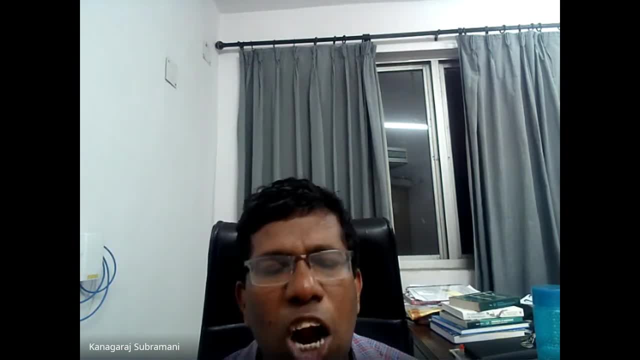 so due to that, his walking pattern may not be at par with the sound leg, so that this is from the experience only. but practically, if he speak, everything can be done okay, so we need to use it with knee joint. okay, after that we can go with the ankle joint in ankle joint also, you need to go with only 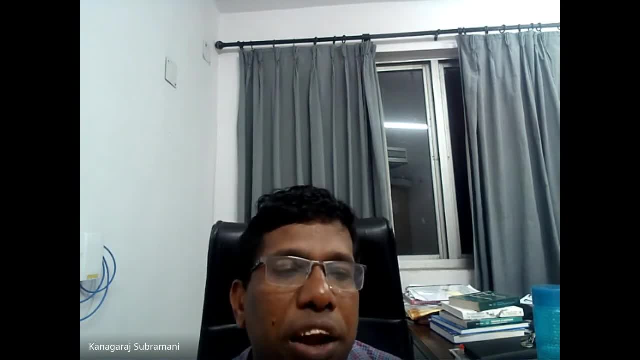 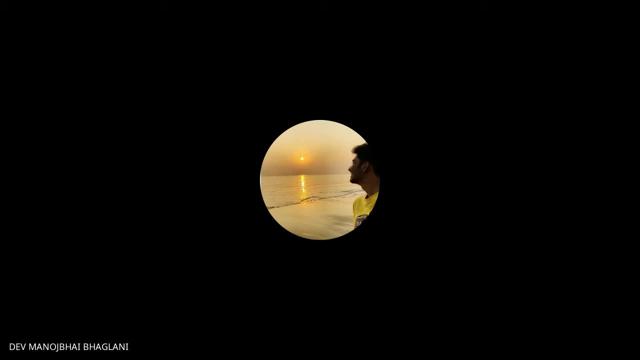 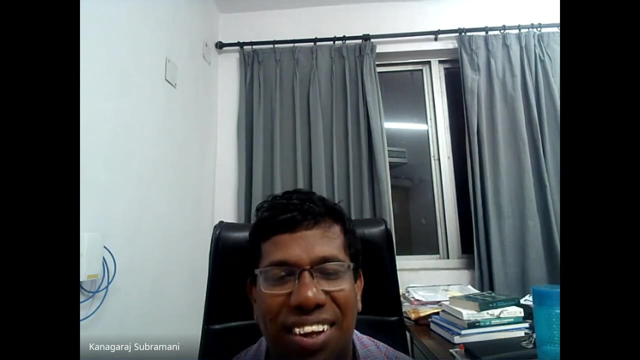 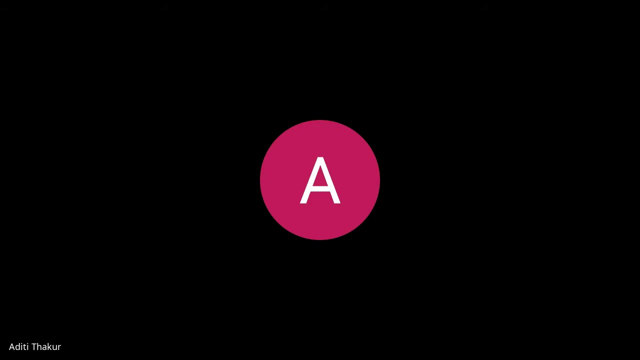 one degrees of freedom, then we need to bring that second degree of freedom later on. okay, it's a practical problem. okay, so it is not engineering. so my doubt was like the many things which have been proposed here, for example, like, uh, the prosthetics which are being used, or the implant, the cochlear implant thing. 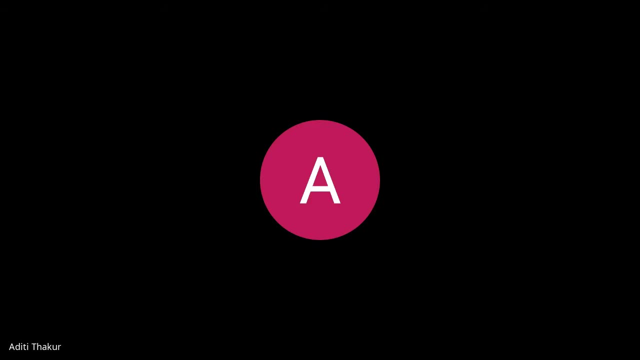 uh, like in, maybe in that specific case, if the if there's a patient and that patient has already undergone a surgery for the things which are already existing, they already have that electrode thing uh installed for their issue. now, if at all the new development comes out and it is uh, it works properly. so, like, is it possible that the person who had such a kind 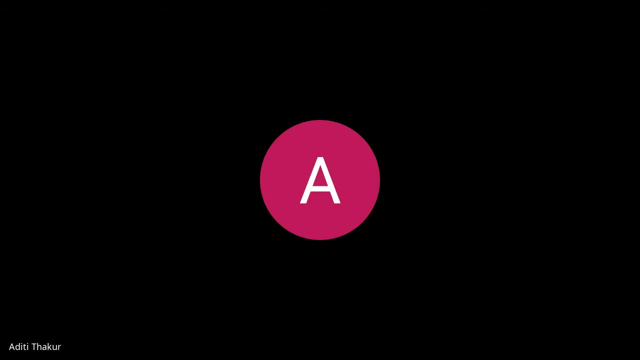 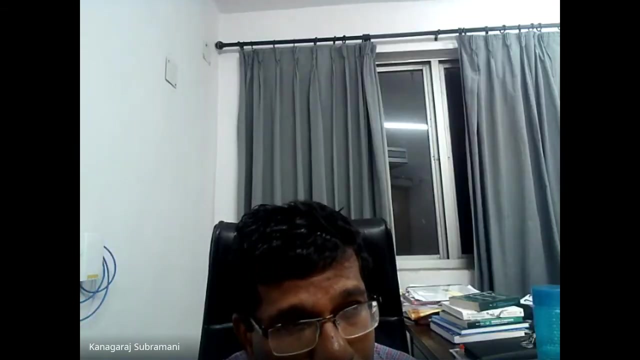 of surgery can utilize it or not, like, maybe due to some surgical things which happen primarily, like: can they use a second thing? and if they can use a second thing, will there be any complications because they had used those those things before? this is about a prosthetic or implant you are talking about. 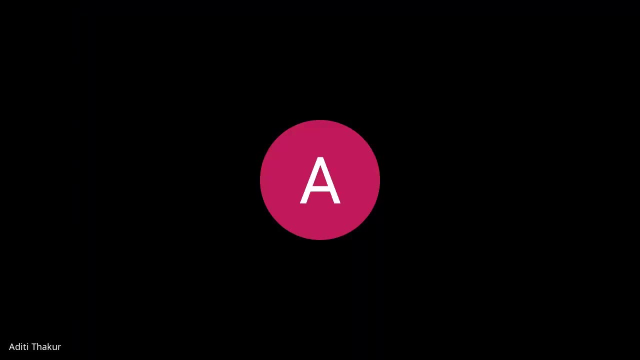 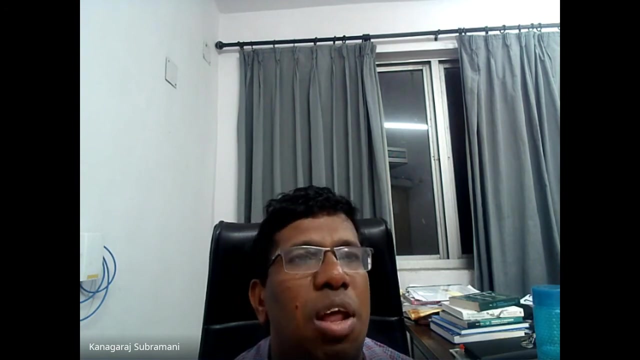 uh, implants. in here i'm talking about implant. okay, implant that has tabular cup- okay, the thing is that it, whatever we have made it, it can be integrated with the existing system. okay, it is not. uh, we can uh, as you are talking about implant and a hip joint implant, if i write. 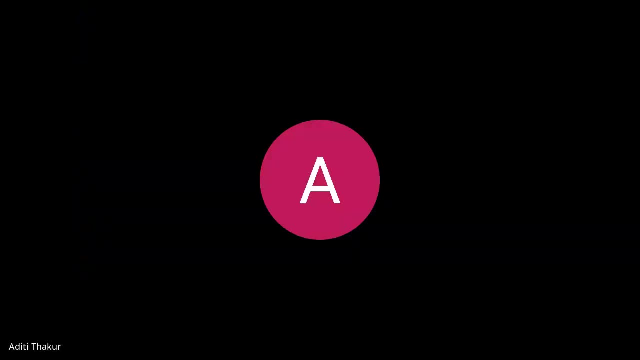 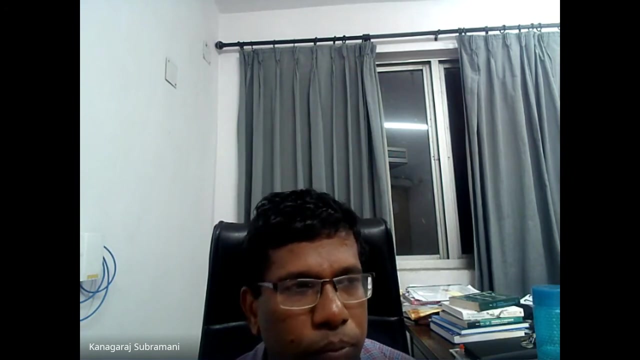 correct if i'm right. yes, sir, yes, okay, so it is something we expect, that the patient will be going this surgery once in lifetime. okay, so you, otherwise what will happen? say, at the age of 50 he is going for that new hip replacement surgery, then generally it goes for metal and polymer or ceramic on polymer. it goes for 15. 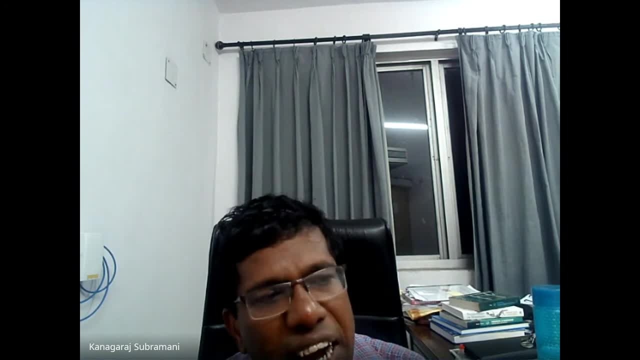 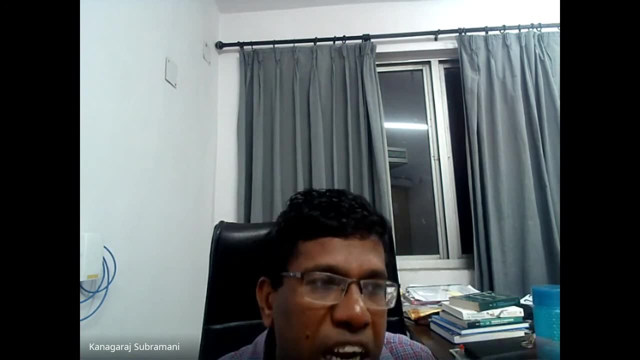 15 to 20 years, at the age of second, it needs to be revised. 100 percentage: it needs to be revised. maybe when it to be revised, that is depending on the activity of the particular subject, the patient. if his activity level is more, then the rate of here will be more, then there will be a. 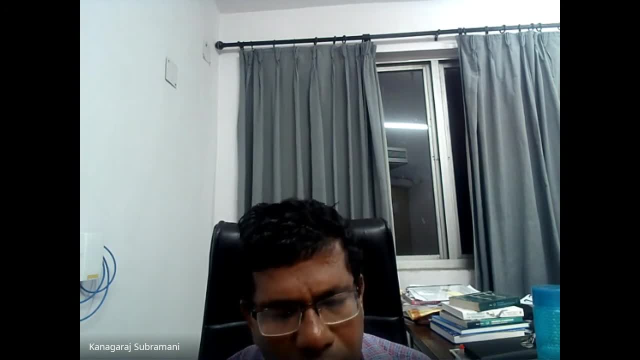 lot of complication comes maybe due to in. there are, even without the- uh, what you can say- without any role of the patient. also that infection related issue comes: he has to go for a replacement and the wear of the implant that also. he needs to go for replacement and the failure breakage all. those things are there, assume that everything is perfect. then also, the patient needs to go for the surgery after 15 to within 15 to 20 years. that is the lifespan. okay, so you are expecting at a 30- 50. he is using it at the 70. when he go for that revised surgery, his body condition will not. 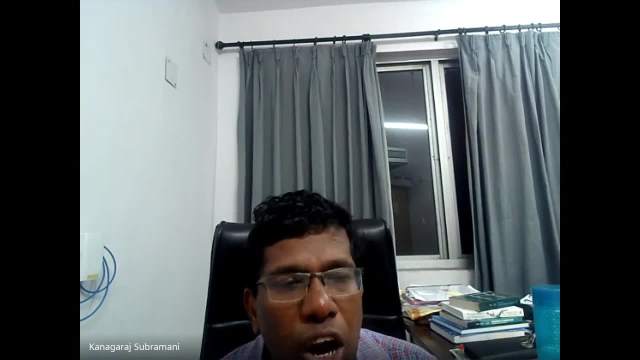 allow him to go for a higher end surgery. that is what our doctor always tried: to postpone it so that another he may need the surgery only for 15 to 20 years. after that he does not need it at all. okay, it is not a fleck and play kind of it. that's that if you are working on a prosthetic or orthotic, 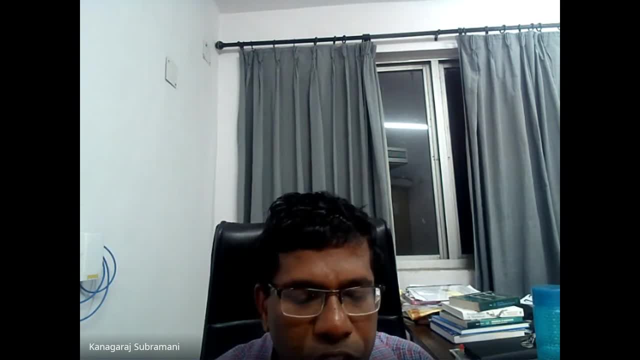 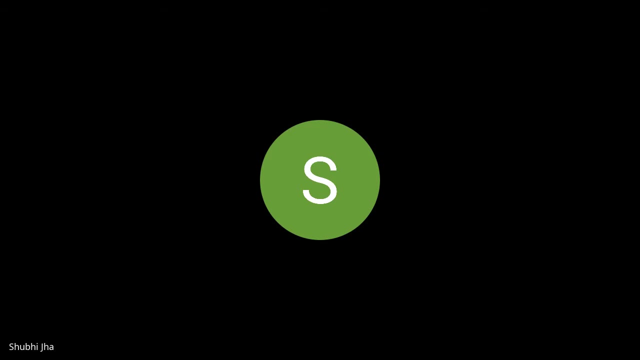 device. no issue, you can go. if today you are wearing one and you don't like it tomorrow, you won't replace. that is not possible in case of the implant. okay, okay, sir, thank you. so this is should be, and i am a b-tech third year student from the idm university. so so my question is that after a hip, 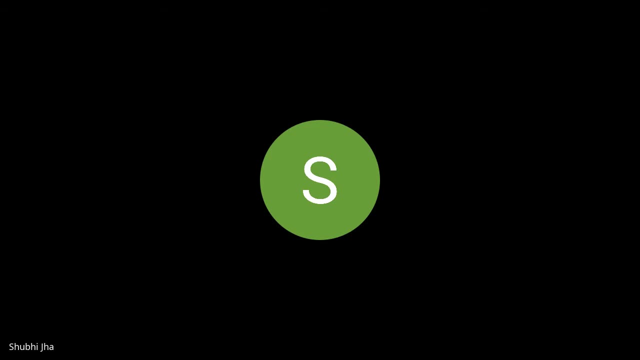 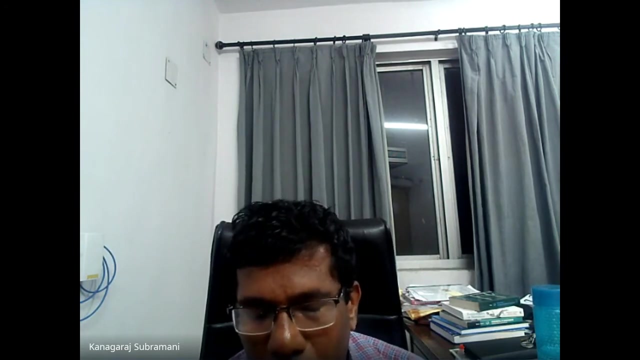 surgery is it possible to reduce the loosening of joints because of the load pressure? so like can we reduce this loosening of joint? okay, loosening of the joint, okay, generally, what we we see from engineering aspect, okay, the doctor can tell their medical reasons. from engineering point of view the loosening generally comes. 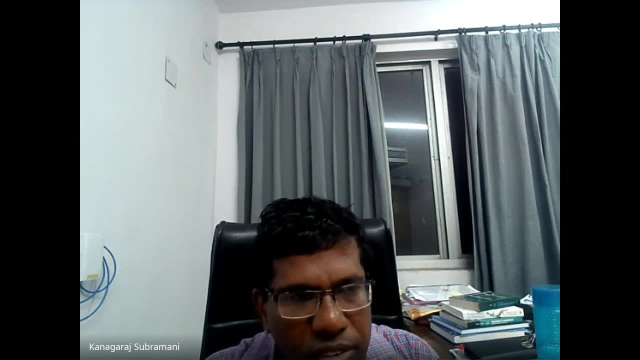 because of that debris generation, that whatever debris is coming, it may trap between the implant. then loosening will be there, then there will be fretting there and all is possible. okay, then if there is a gap between the implant and the bone, then a perfect load transfer will. 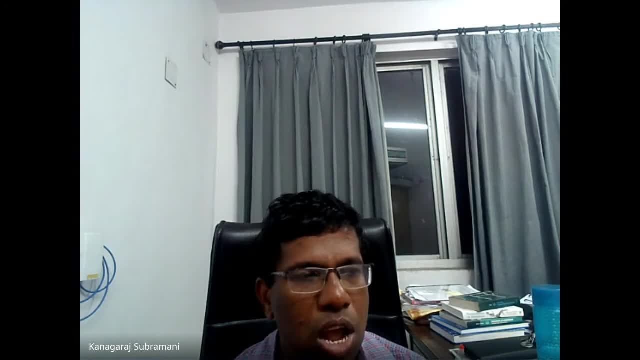 not be happening from the implant to the bone. after all, that implant is just maybe in the femur. it is about one third or one third length of it. after that load needs to be transferred to the femur. then if it is a gap is there? then perfect load transfer will not be happening. 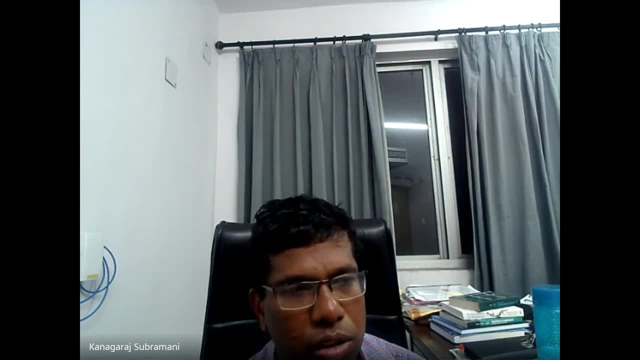 then a patient will have a pain, if at all. any gap is present there due to the wear debris. i hope it is working. yes, it is from my knowledge. okay, because doctor, that's what i'm saying- doctor can say different version of it. we are seeing it from engineering aspect: that debris, it will be accumulated. 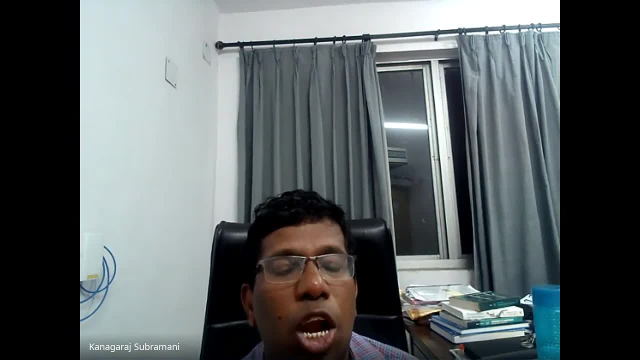 between the interface. that will be damaging that perfect load transfer between femur and that implant. of course, this is something we are discussing with with general patients that in general, will not be available for access and the information that we will be able to provide to the patient is much more accessible for all the benefits of the implementations. 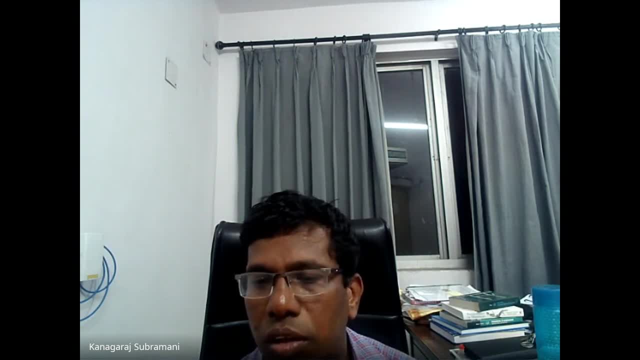 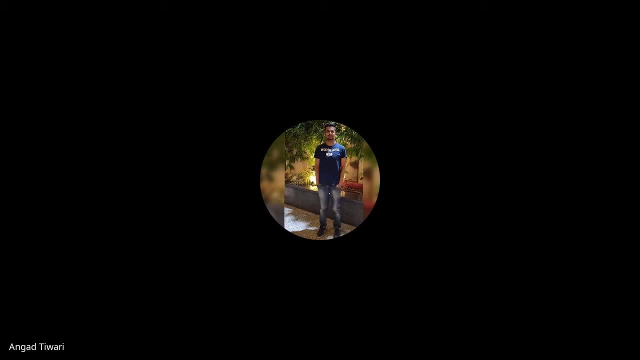 so i have my hopes and insights on this. yes, yeah, right, good evening, professor kanaka raj. my name is andre and i'm an intern doctor at government medical college. hsi, the aspects and the name plan that you talked about, uh, it was an enriching experience. uh, i. 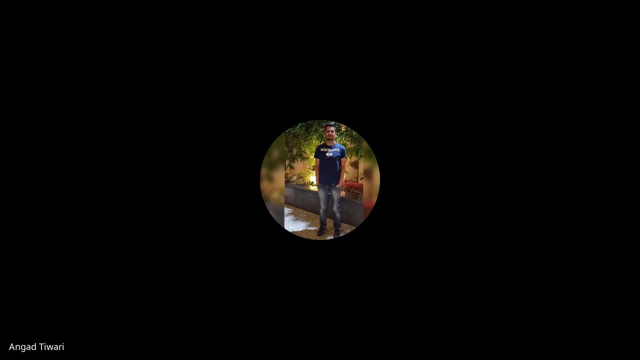 just have a query uh regarding the material that is being used in the prosthetics that the that the iit kohati has developed uh like, uh personally, i have seen that uh, the kind of prosthetics, especially the jaipur, which is very popular in the country uh the patient tends to and india's 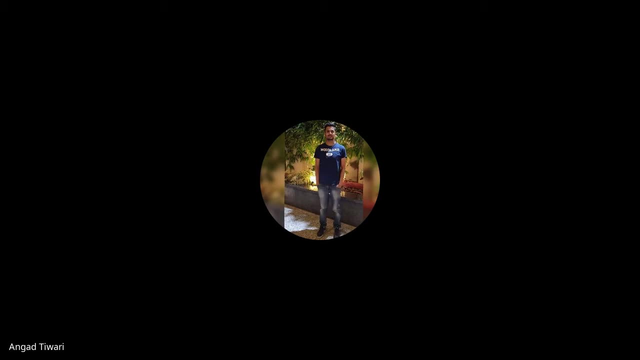 insects. india is a tropical country. uh, the patient do have the hyperhidrosis, which is the excessive sweating right, so like uh, and they tend to develop contact dermatitis or problems like contact dermatitis and stop by demand. so do you think uh, the kind of prosthetic uh which the iit kohati has? 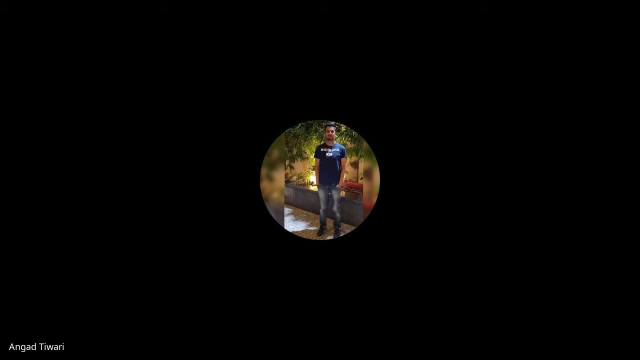 developed uh? does it address or does it have any long-term implication on the material of the prosthetic being used due to the excessive sweating? or does a prosthetic or does address the issues like the contact dermatitis which is commonly seen in the checkerboard? okay, thank you. and in this case, 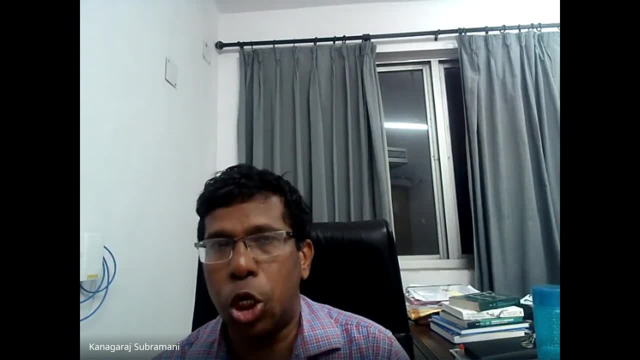 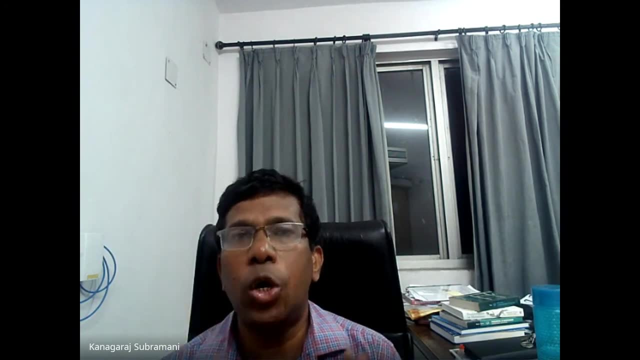 what you are telling me is that the iit, kohati, has developed a prosthetic which is very popular in the. that mainly on the socket related issue. okay, so, as you have seen that in one of the study, what we are doing is, uh, once we do that analysis in that socket, wherever there is a less concentrated area, 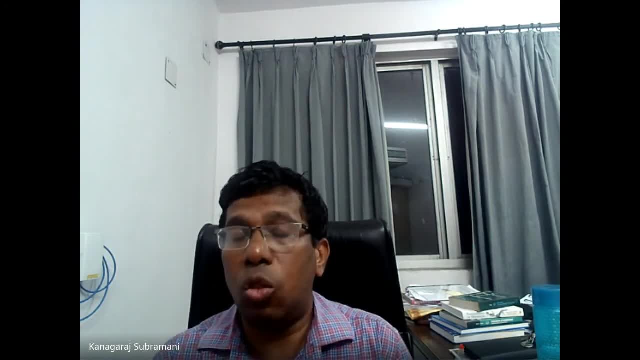 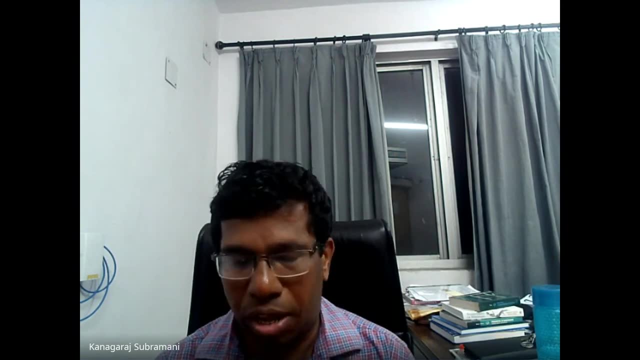 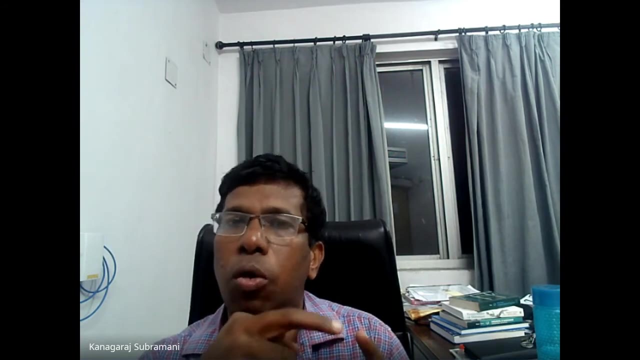 stress concentrated area. we will be having a- though we have not made any socket like that, but that is what we need- to have a topology optimization of that socket. when we have a oval or maybe there's some space over it, what will happen? we will be ensuring about uh air circulation within that. 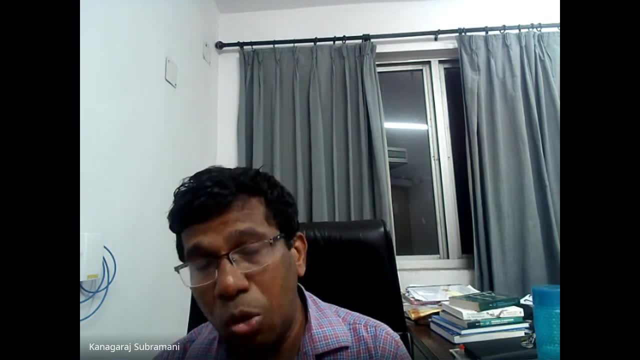 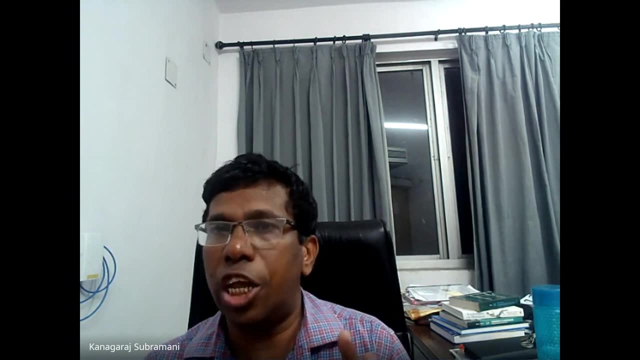 okay, so that the sock, that one, we are using a conventional socket with the prosthetics and we have not made anything like that. but if we are doing analysis in this one, we can ensure that cavity or the hole in the socket. one issue is that once you make some cavity or the hole in 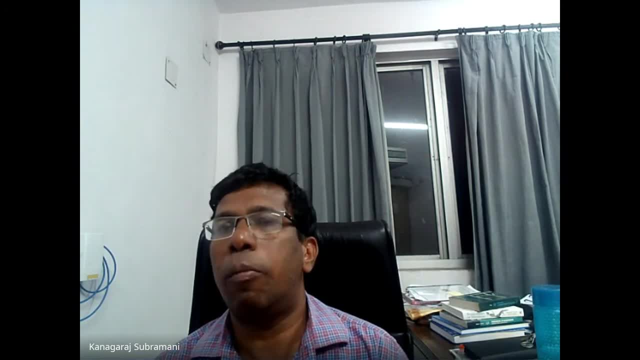 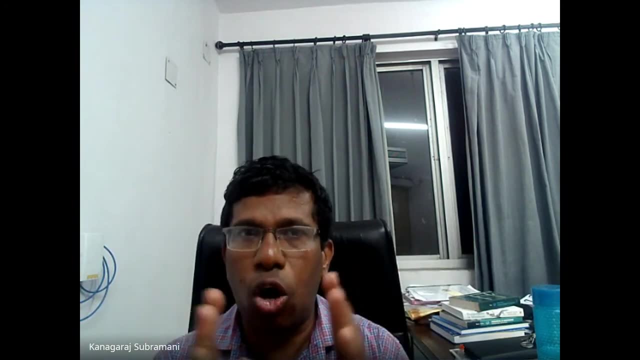 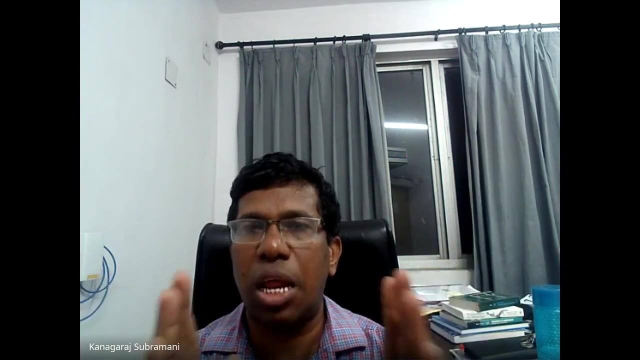 that socket. we need to do that analysis once again because what will happen in normal case? we need to do that compression on. we need to have a compressive load on the residual stem and if you have some cavity, what will happen? the compressive load acting on the stem will be reduced. 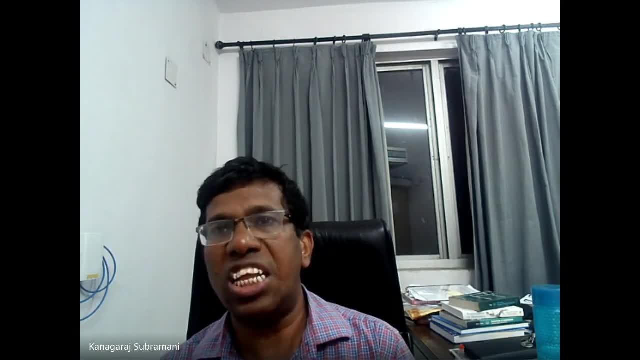 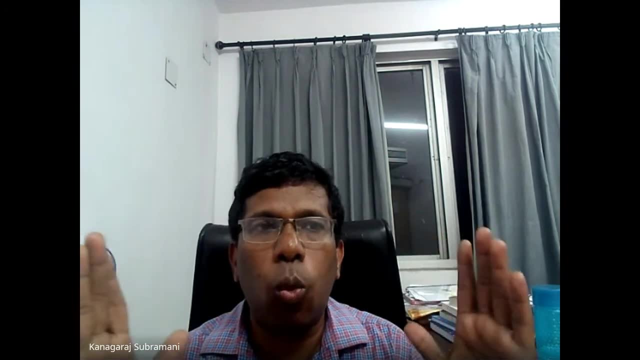 then it will. we don't know what will be happening on the because for engineering side you can have a cavity and just reduce the stress. but that compressive force, what is required over the stem, that will be reduced. that is what we are working on it: how we can ensure that same compressive. 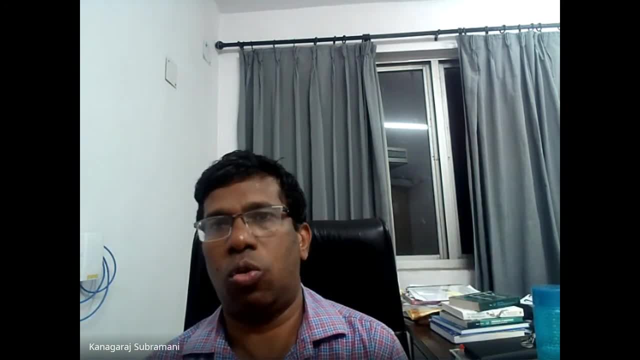 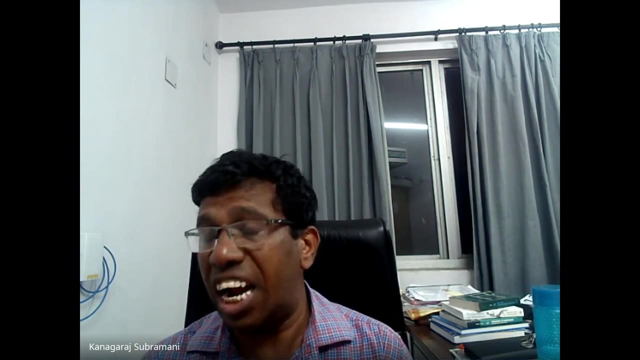 load acting on the residual stem is reduced so that that adduction on that residual stump could be reduced, not at the cost of the functional activity of it. however, as you are talking about that uh sweating and all like that, maybe what you can say: uh, somewhere we can have a breather with. 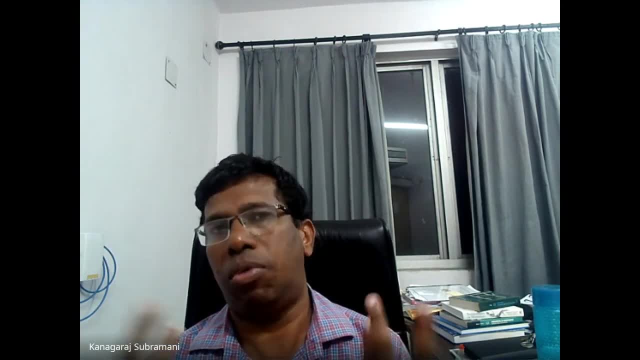 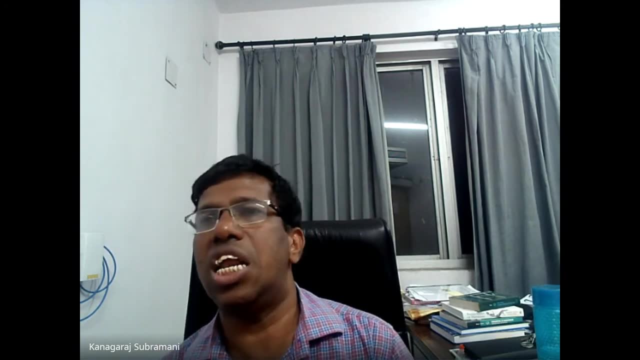 that liner, whatever it is being used. we can think of a breathable liner so that, uh, it could be absorbed and maybe air circulation and all that could be possible. that it mostly it comes with a breathable liner so that it could be absorbed and maybe air circulation and all that could be possible. 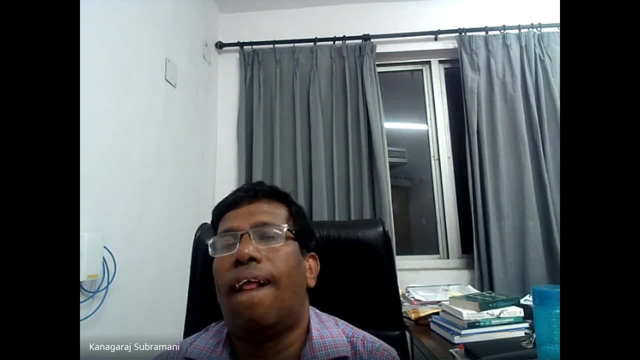 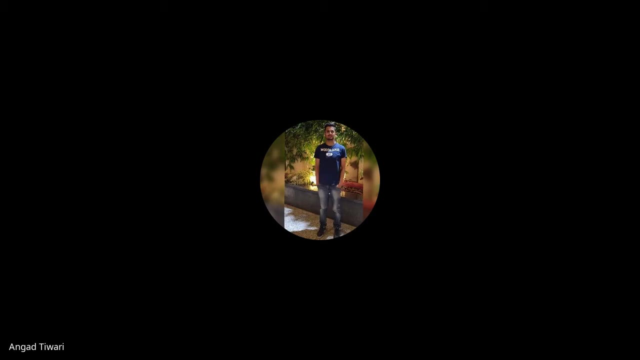 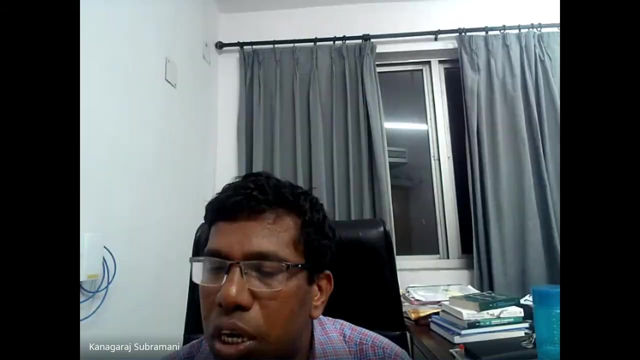 we need to work together, then only, it is good we are not grabbing on the part. whatever section study we did, we have not made anything. however, that analysis is going right, sir. thank you, thank you, sir, thank you. uh, yeah, any other questions from anyone? no one question is there in a chat box. okay, what is the state of this ultra high? 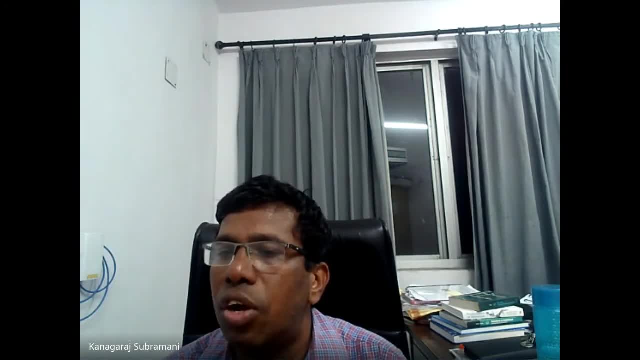 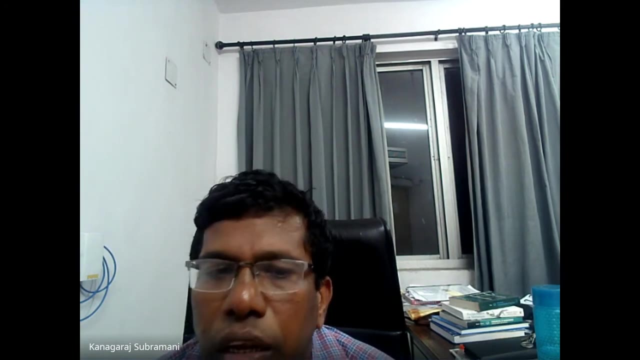 multiple relevant at high temperature, when they are really concerned: the functioning of the state of this relevant at high temperature, high temperature. mr danis, are you there? oh, uh, can you please what high temperature you are talking about? during a presentation you would you made a mention of? uh, how that uh? 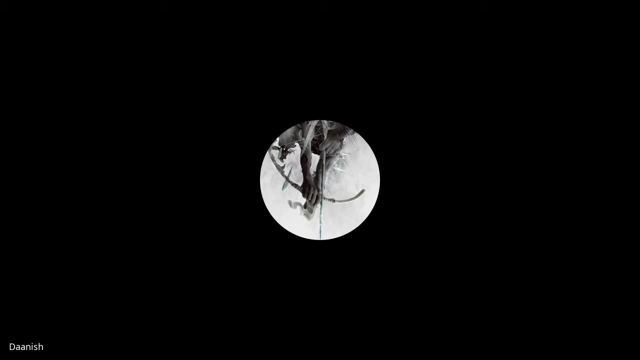 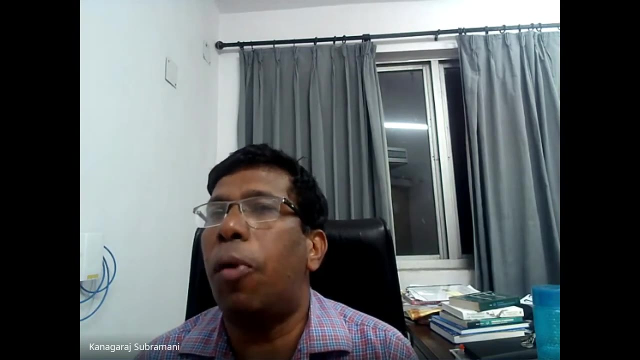 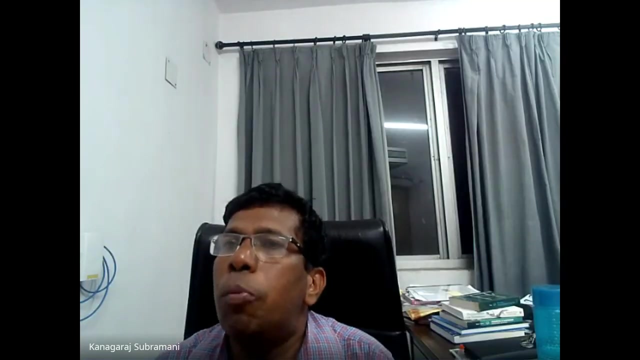 that material, that polyester, behaves then, see, you need to process the polymer. though the material is going to be used inside the body, this temperature is not increasing more than 37, but you need to process the product. processing temperature will be high. you need to have. it is around 165 degrees celsius, которую. 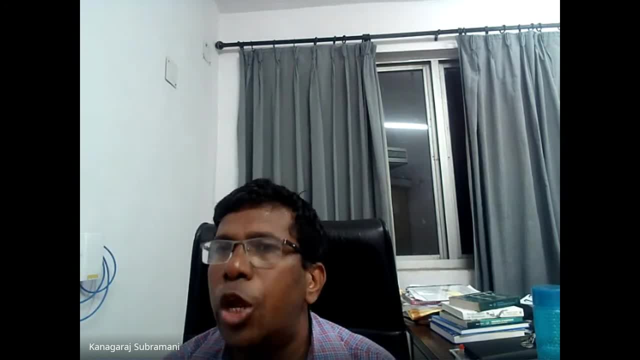 we need to process it, you need to from the raw material, you need to have that desired product. okay, and the uniqueness of these polymaries: it is having high melt flow index and it is a molecule. molecular weight is around five to six million gram per mole. okay, so due to that, it even at the 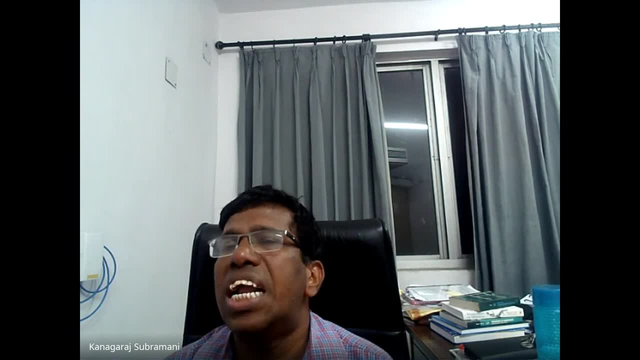 molecular weight is around five to six million gram per mole. okay, so, due to that, it even at the molecular weight is around five to six million gram per mole. okay so, due to that, it even at the million gram per mole. okay so, due to that, it even at the melting temperature. there is a keeping of that. 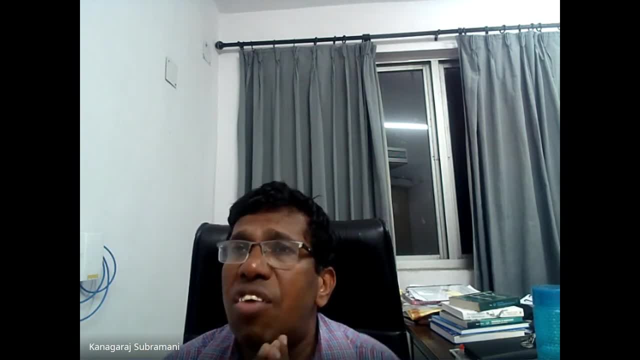 ため ni mucho y esto zomunsga. it gives population whether you want to have this polymer. if you first take it, it even at the melting point. also, it will not have a flowability. okay, it will behave like a solid, only highly discussed material. this one, that is what it is- not being processed in an injection. 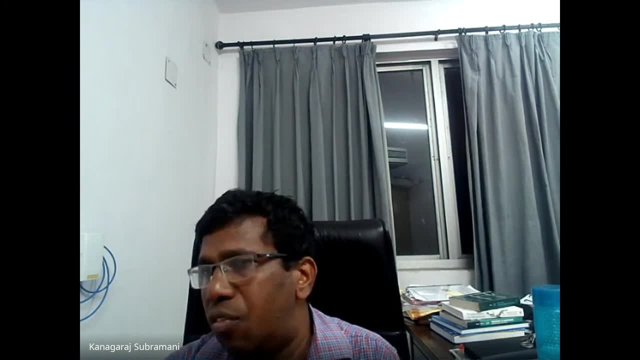 molding and all like that. so you need to. what we are generally, what we it is available in the market, is extruded rod from that. people are doing a machining to get the desired file right. temperature means i mean the processing temperature right. right, it does not have anything. 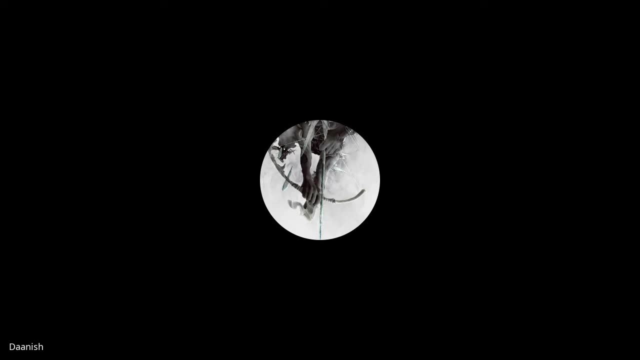 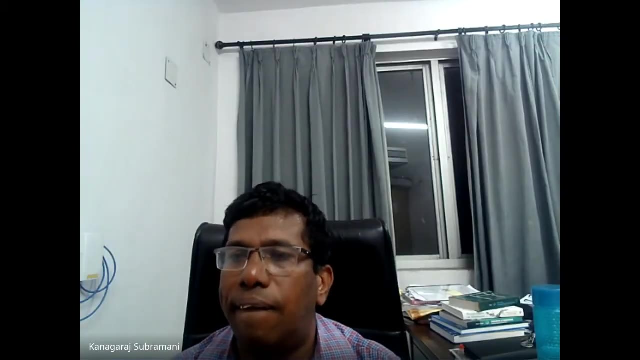 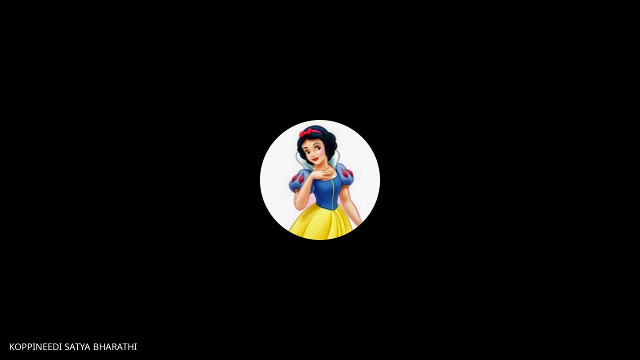 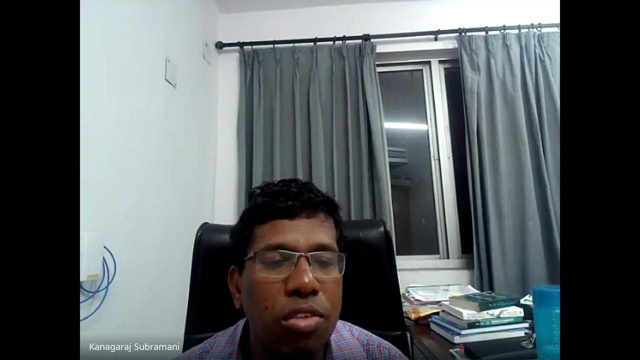 to do with what behaves inside right? no, no, no, no, right, thank you. thank you, sir. i just wanted to know again the method that was used in aneurysm. please introduce yourself first. introduce yourself, then we ask your question. yes, sir, hello, i am satya bharti, third year. 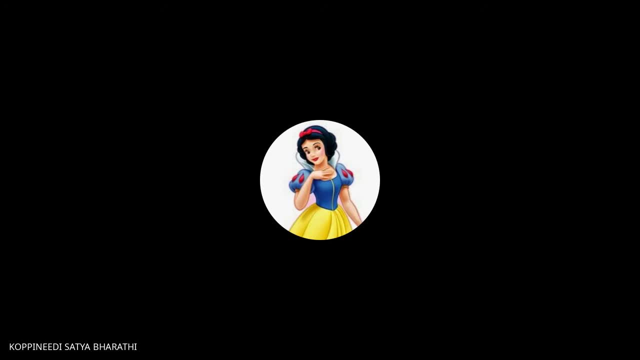 mba student from surat kujrat. sir, i just wanted to know more about the aneurysm uh treating method which you have discussed. it for the printed, yeah, yeah, yeah. so in this one, that current technique is filling that aneurysm zone with. 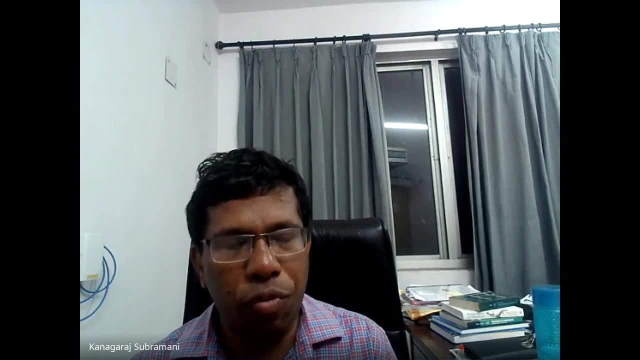 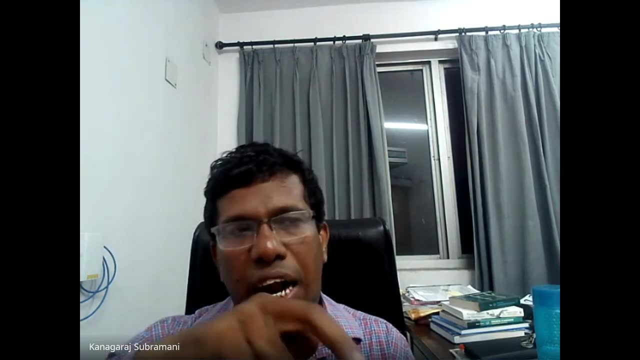 a platinum coil. that coil will be inserted into the femoral artery via the catheters and once it- uh, they will be just, it will be a coil kind of it. it, once it reaches that aneurysm and it is filled, then after that there will be catheter, will be detached from the- uh, that coil. 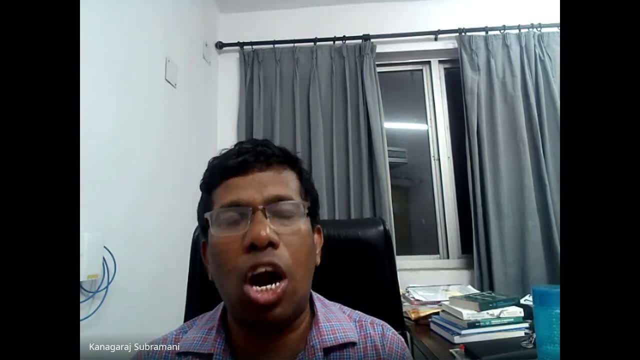 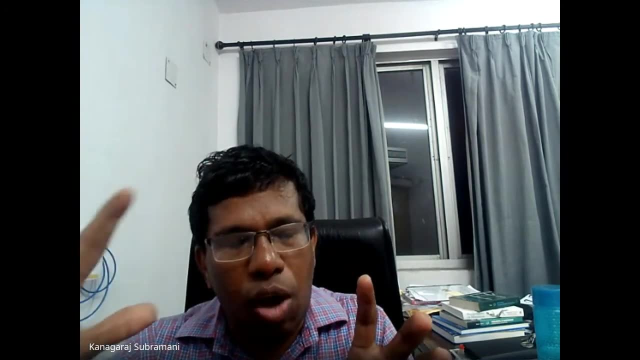 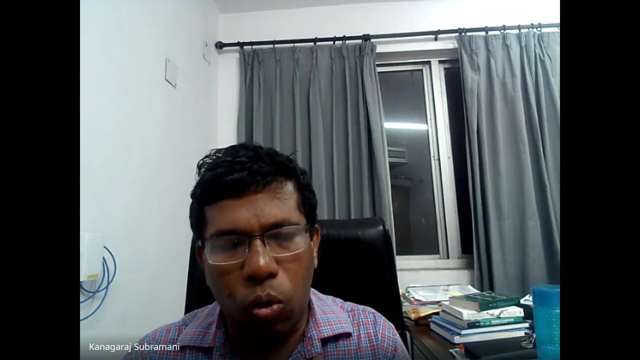 however, that limitation is that the packing density is not high. still, there is a blood flow. okay, and already this is something. blood vessel came in the form of a balloon. okay, that it is. it becomes so soft. okay, the continue. if we are allowing the blood flow, then 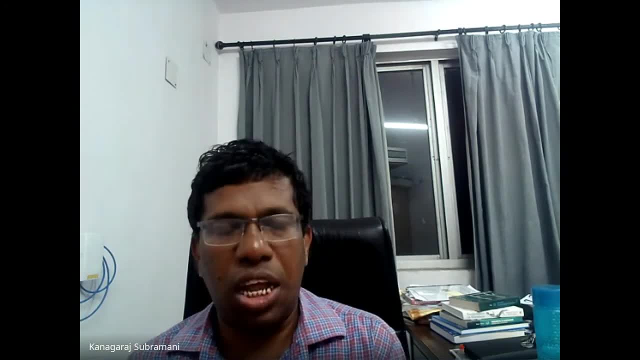 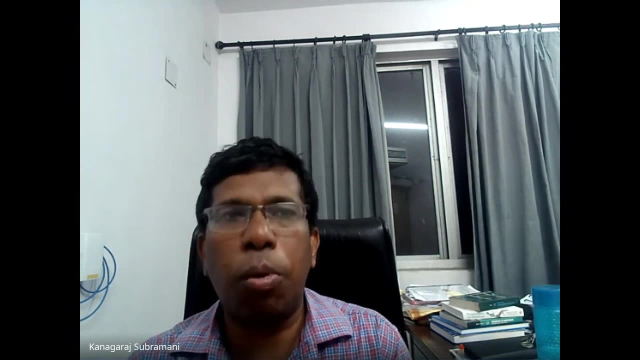 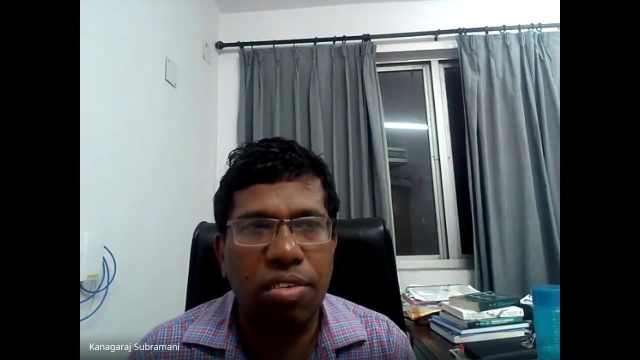 at some point of time, even after filling also, it may burst. that is the reason why people are going for a liquid and embolic material like onyx and all like that. what we are proposing is that solid embolic material. once we get that pattern, aneurysm, shape and size, we will make it a 3d printed uh. 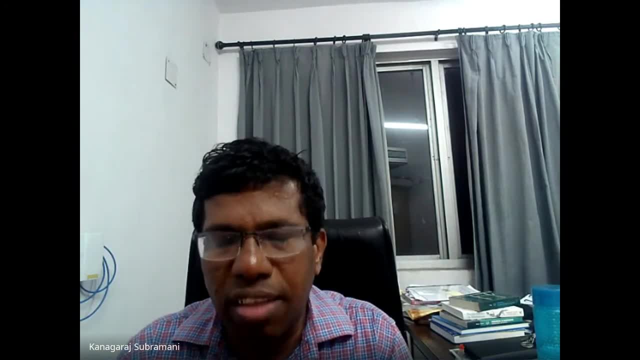 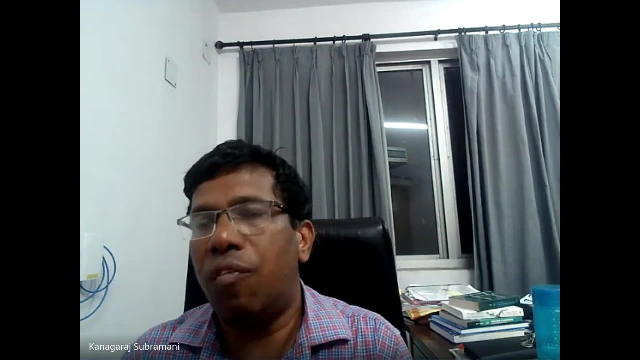 polymer. we will make that product of the same shape and size with 3d printed. whatever i have shown, it is a enlarged version. okay, we are not. we have because it is for we need to test it outside before we go into the animal and all like that. that is what we have enlarged. it's the size and 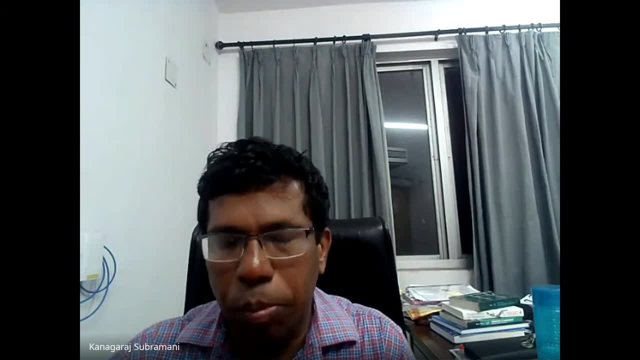 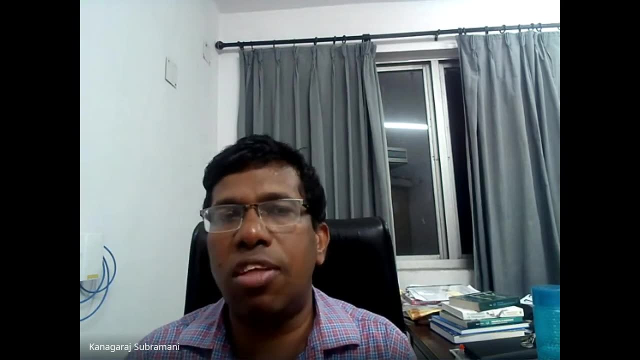 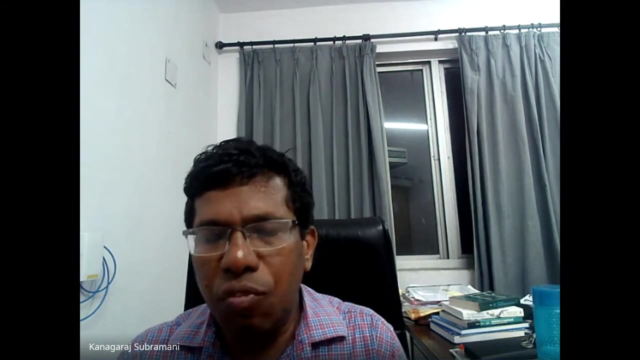 it is some size and we have made uh with a shape, primary polyurethane with radiopack material. here we have used nano barium sulfate because, being a polymer, you cannot see it under x-ray. that is what sulfate, to reduce the concentration of the radiopack material. then we have got the shape of 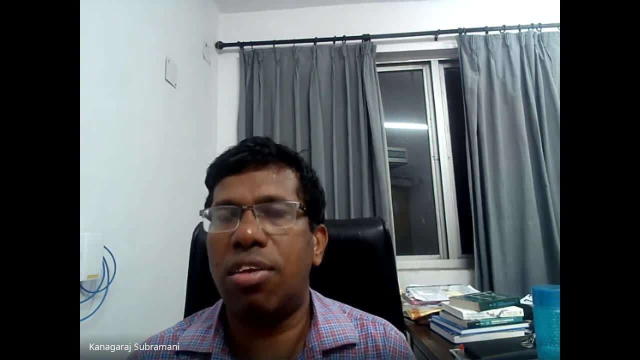 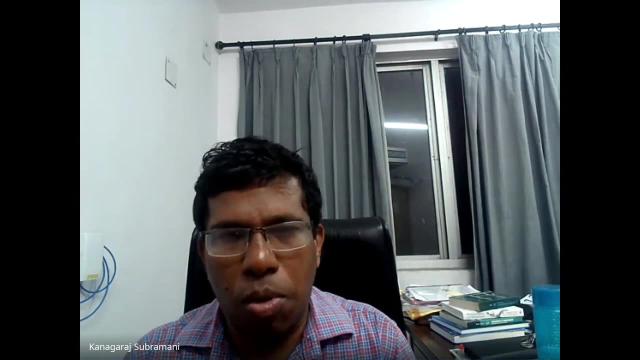 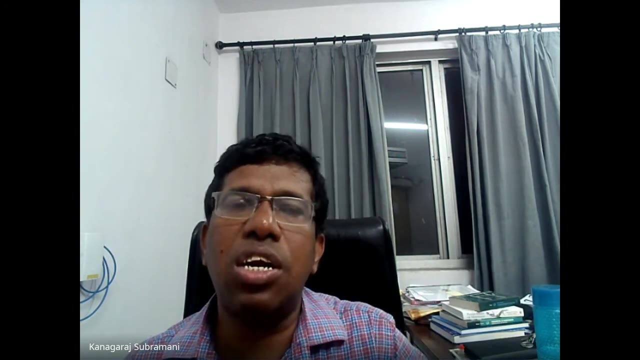 that aneurysm? okay. then for an in vitro test. what we did? we got some kind of a shape, okay, what some kind of a irregular shape kind of it. then we converted in the form of small wire and it was inserted in the catheter, kind of it like a tube, okay, and that we have inserted into the artificially. 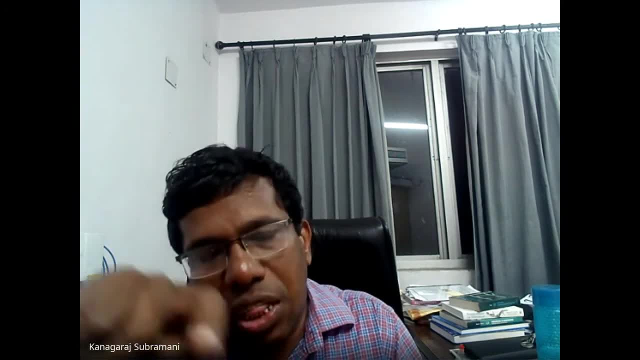 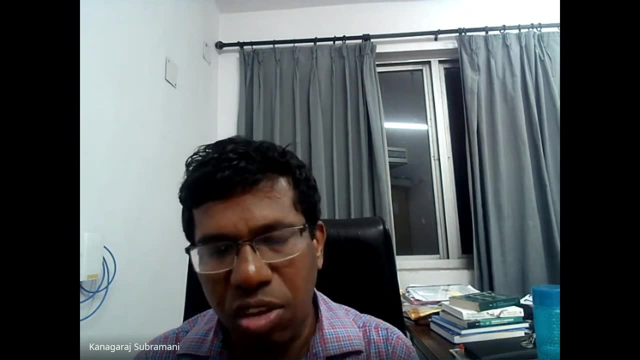 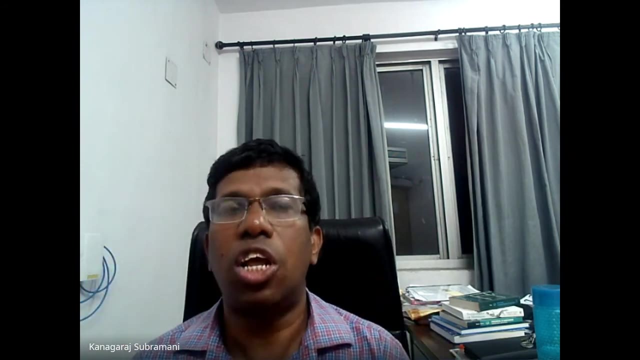 made blood vessel. we have made with the silicon rubber, with aneurysm, with the analog size, and we have inserted this polymer, shape, memory polymer. we have inserted into the cavity and after 5-10 minutes we saw that we could get the same shape of that, the initial material. 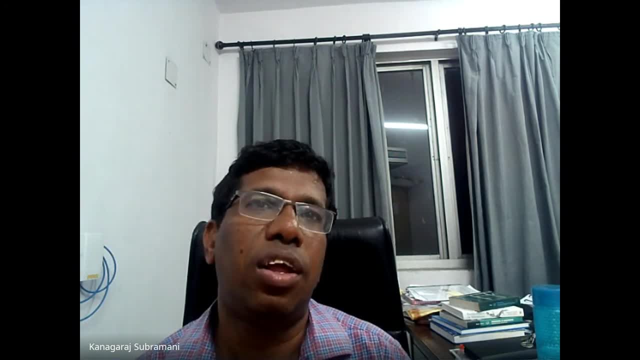 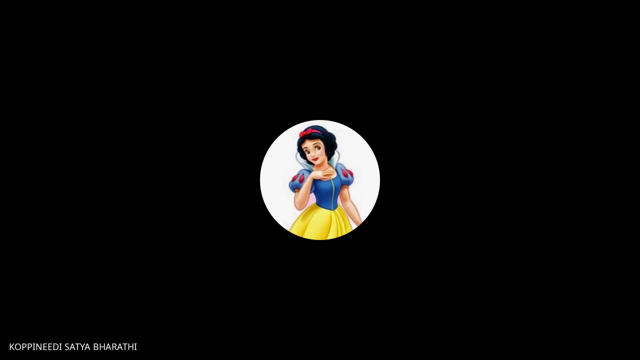 that is the proof of concept. we did it. so, sir, it will prevent the high blood flow through it so that it may not burst out. no, no, it will not. that is what it will be. it will be in the same shape. it will be in the same shape. it will be in the same shape. 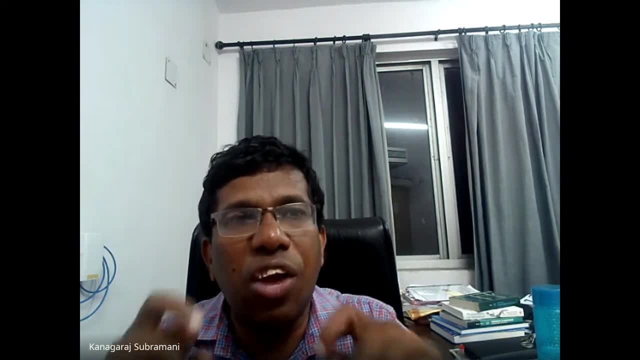 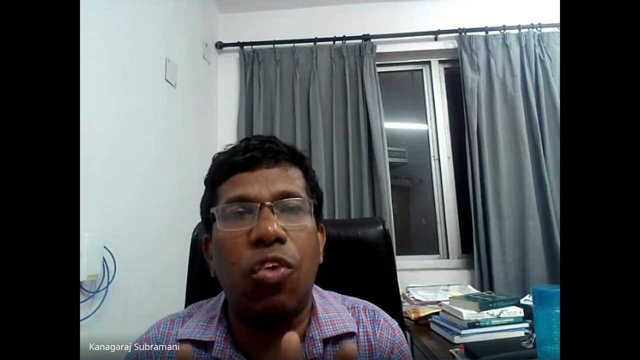 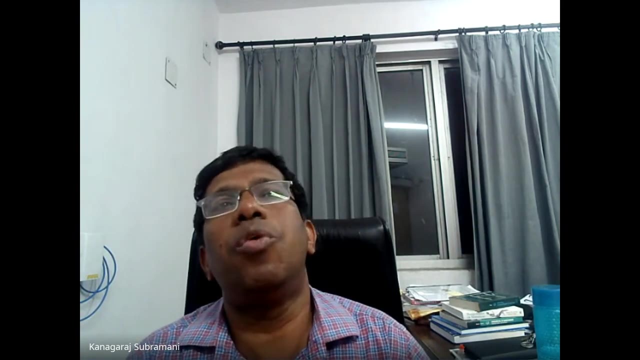 till 10 minutes of time. till 10 minutes it will retain its shape. that is what we. i said we need to play with shape and size so that until 10 minutes it will not increase its size. once it reaches the, once it reaches the desired destination, then we will allow to increase. we come back to the original. 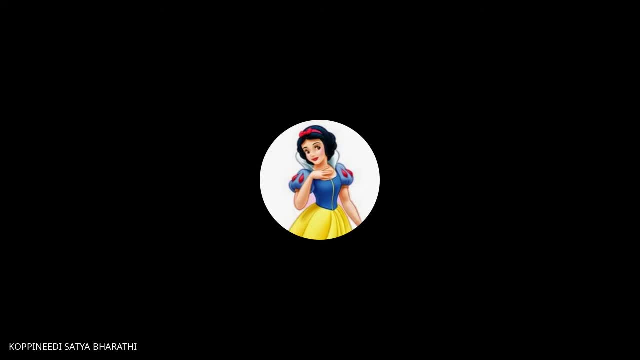 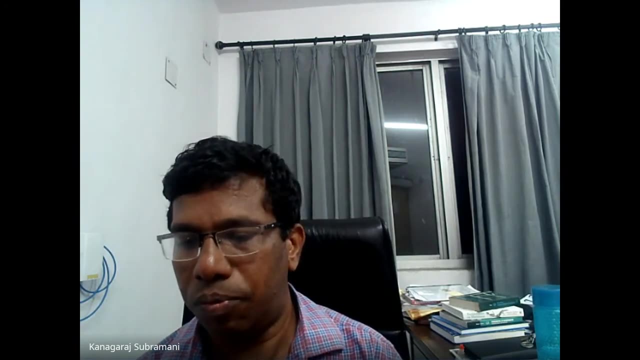 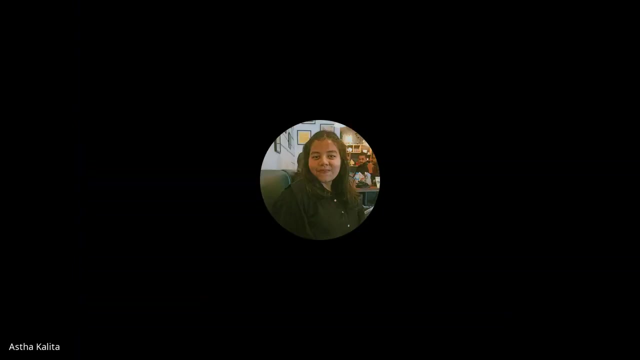 shape and size okay. during inversion, nothing will happen okay. thank you, sir. thank you, yes. good evening, sir. i am third year chemical engineering student from assam engineering college, guahati. so my question is that, uh, in various international paralympic games, are they using the third generation prosthetic leg or are we even in the scope of using a higher level of? 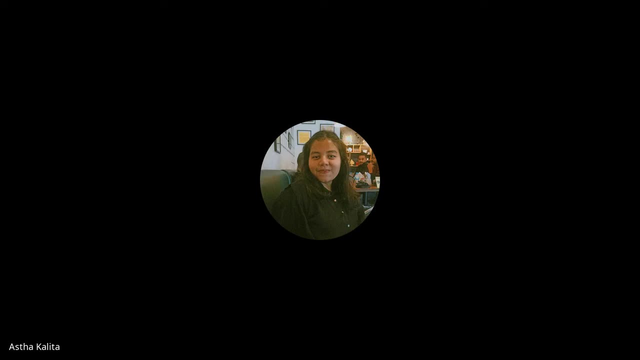 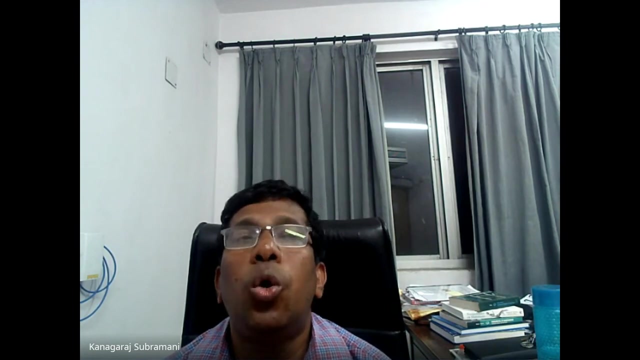 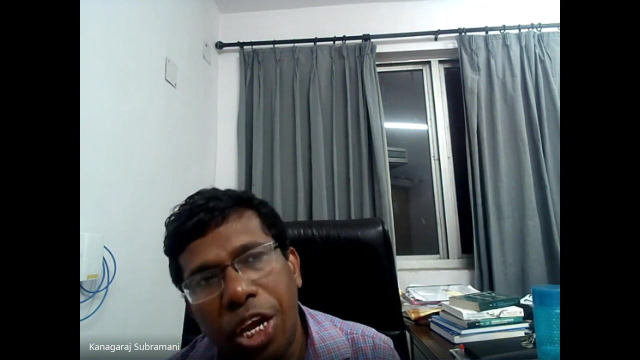 higher generation of leg. see, when we started, our first objective is to. we need to. the patient needs to go and do his daily activity. okay, that is what, and it should be affordable. your if and we can go with what you can say: robotic arms and all like that, robotic legs and all. it is a monocle, it's a high. 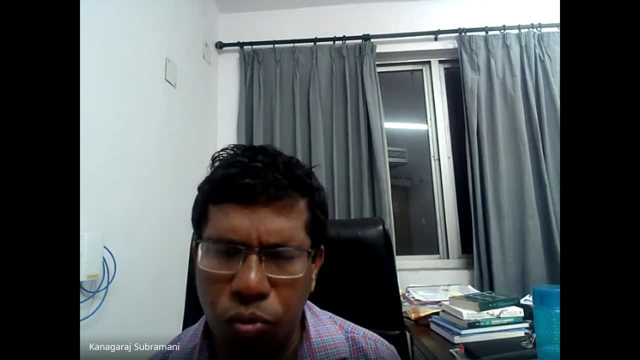 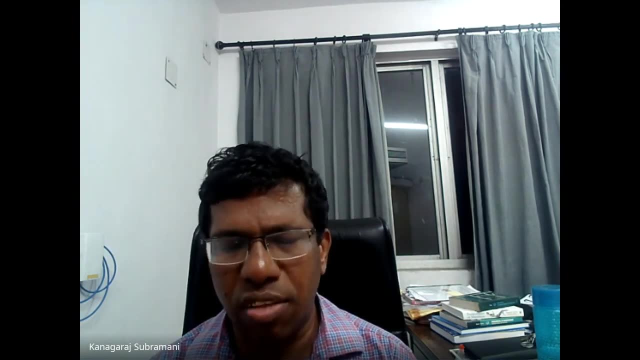 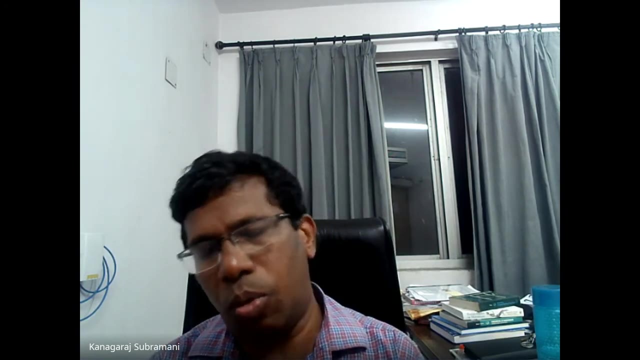 end device it is, it turns into fuel lags. okay, and that our requirement is: many people are having not having the prosthetic device. many people, in the sense 80 percentage of the disabled people. okay, are that people with a locomotive disability are not having the device because it is not? 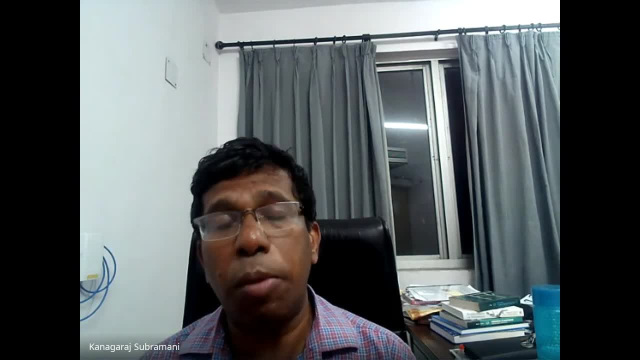 affordable. they it, if the product may be active device may give that the gate pattern will be at par with the sound line. okay, and however, if you make with the passive device, it may be little bit inferior. okay, it may not be exactly the same percentage of the robots. okay, so it is achievable. every material self-contained and free of cost, okay, or it will be much less existemooh, baby, it may benefit you in making the device. it may be easily available through AMQ of theёз of the basehowever, if you make with passive device, it may not be exactly the same percentage of the вже. 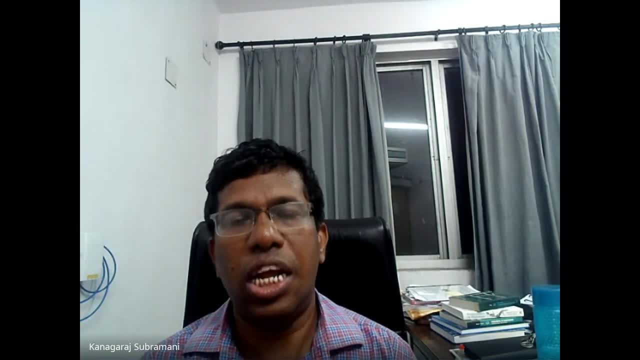 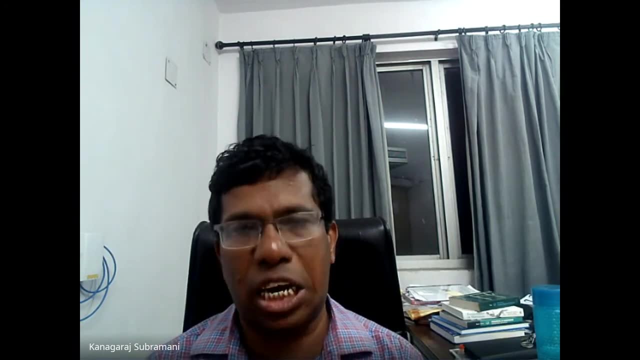 device. okay, it may be not have the device. if the device does not through the PSMD is considered according to the of a gait pattern of sound like. it will be little less, however, if you could able to reach 75 to 80 percentage of that activities, normal day-to-day activities and functional activities, excluding 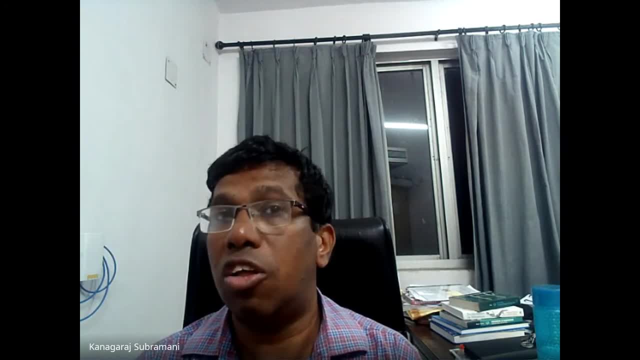 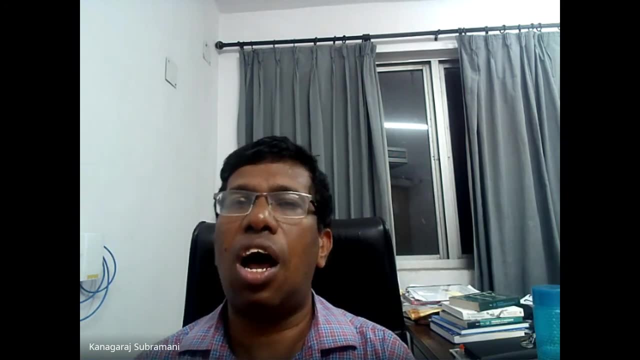 the sports activities. okay, uh, that sports activities excluded in our design. okay, he can go fast walking and all like that. he can sit in a car and all been that much is feasible enough, okay. so fourth generation: if you are bringing an active one, see in this all three cases. we have done a. 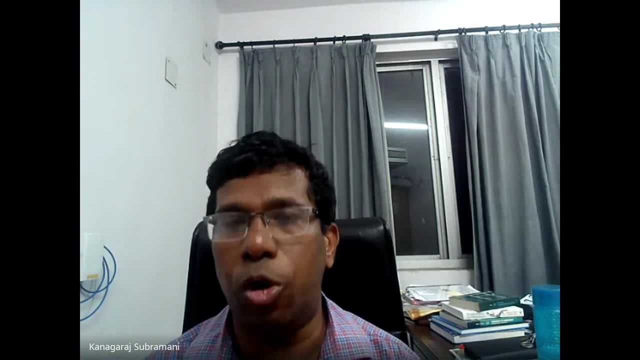 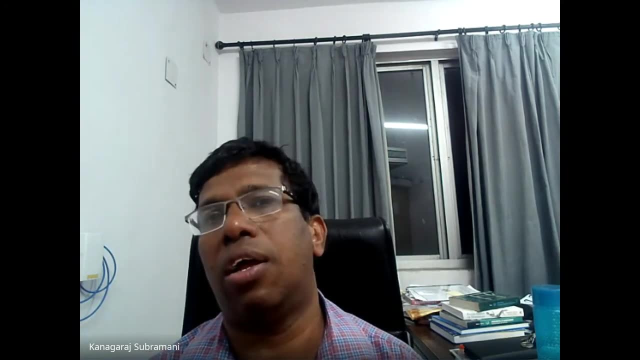 testing and we gave that prosthetic device to the amputees. they have been using it. okay, if you are using an active device, we will be testing a subject and we will be collecting it back because of- uh, it's a cost we it cannot be offered affordable for the research of him also. 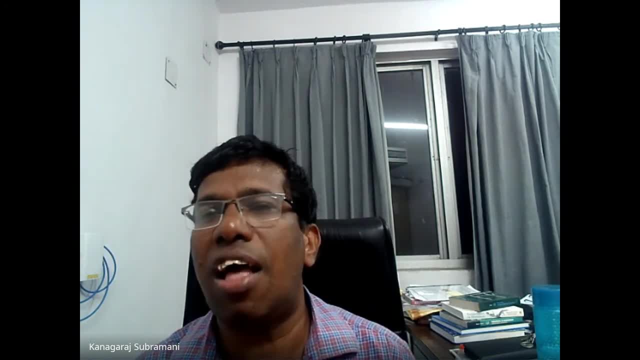 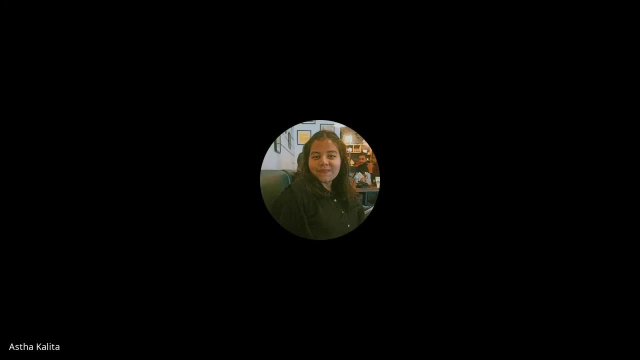 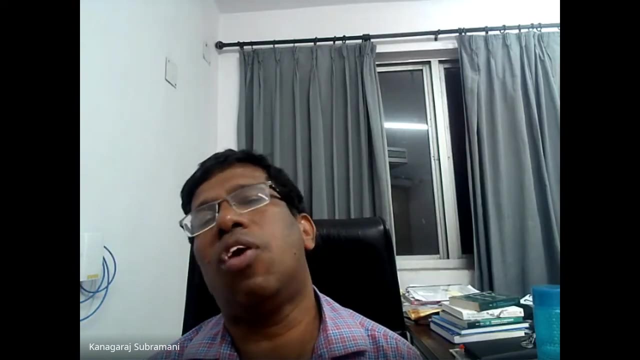 as of now, we don't have plan. if some sponsoring agency are asking us and they are giving money, we don't have any problem to take it forward, okay, so so what will be the best prosthetic material prosthetic material you can for a patient trial? you cannot say nothing. is the best, okay? it will be varying from person to 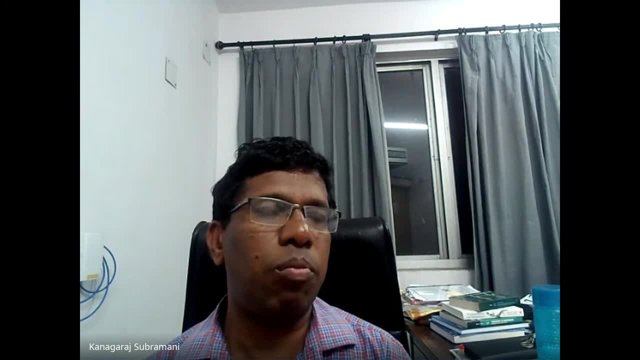 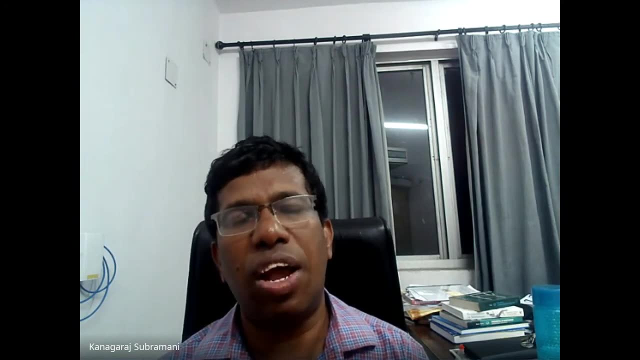 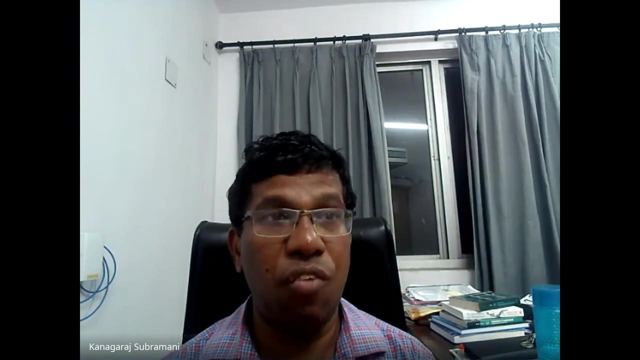 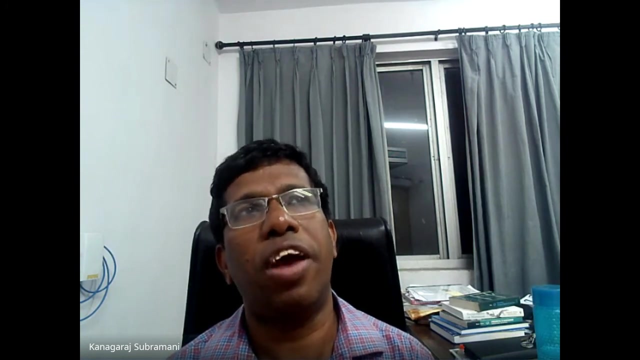 person. okay, best in the sense. uh, first we need to see about the functional activity. suppose if, whatever we have made the device, that device was for maximum loading of 100 percent, 100 kg load person can use it with the factor safety of uh, what you can say? we have tested it for four, three, five. zero means 435. 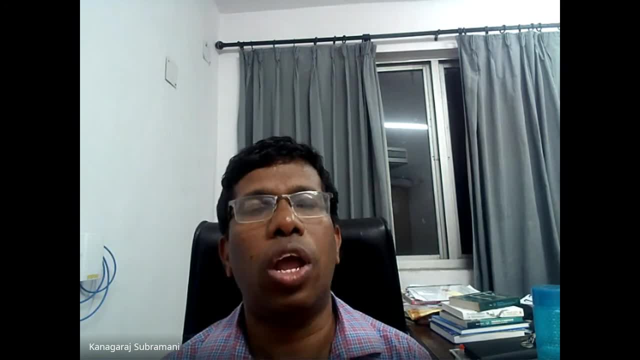 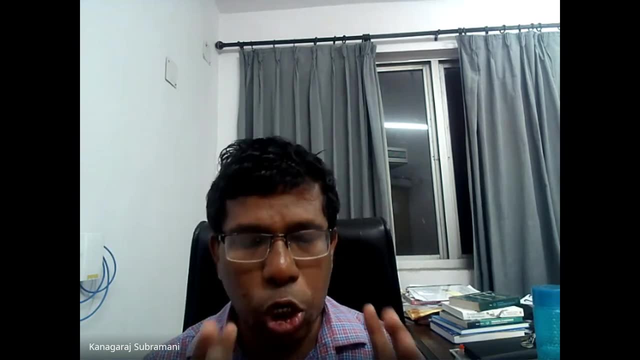 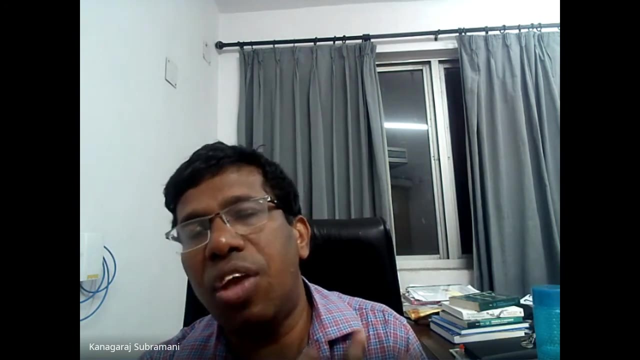 and it is about four. four after safety of 4.3. okay, 100 kg person can use it. so we need to ensure that when he is fourth hundred kg person, when he is using it, it should be stable enough and stability is the first criteria. okay, that is the way we need to take it forward. the mid which material and 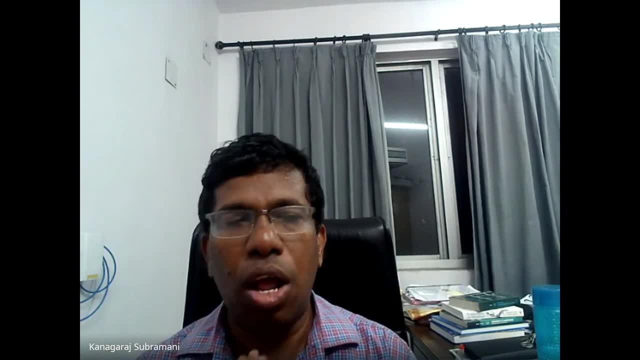 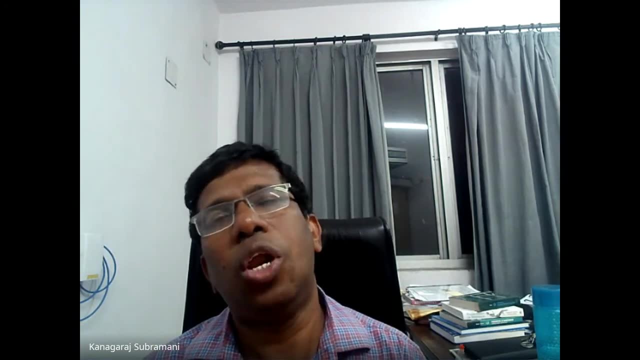 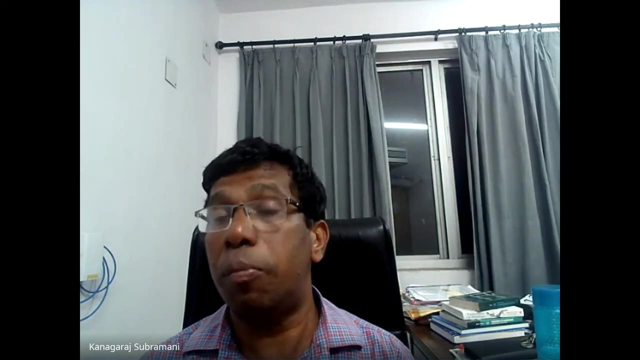 all. anyhow it will be, the device will be covered with the normal foam kind of it, so his leg will be looking like a normal leg only, as everything will be covered. so we'll go with that is what we started with the nylon. so whichever component is there we have made with the nylon and whenever 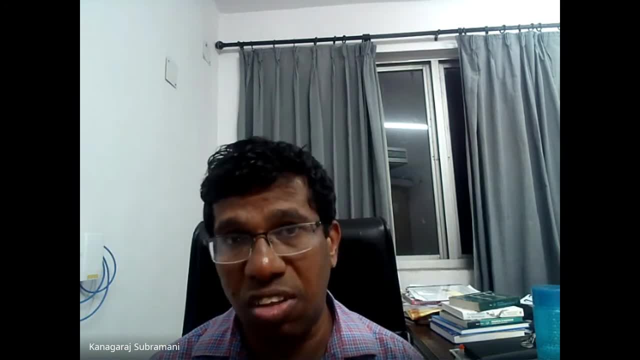 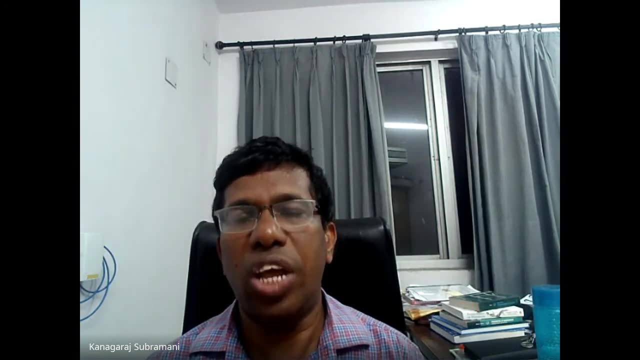 metal part is required. we had gone with the aluminum alloy 6000 series and wherever the thread and all comes, we have used a stainless steel 304. okay, we have reduced the metal quantity as much as as many mass possible so that the prosthetic leg will be. 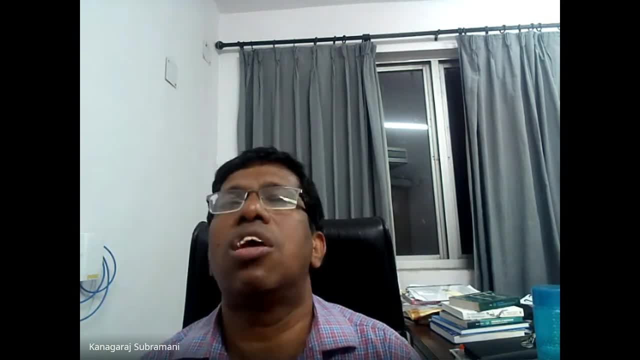 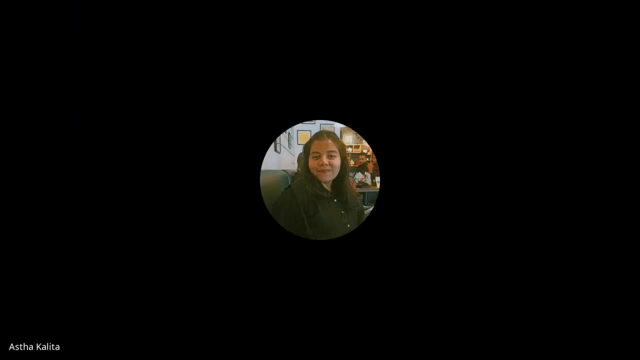 weight of the prosthetic leg will be at par with, uh, his sound leg. okay, thank you, sir. thank you, uh. uh, great news though again. uh, um, my name is angus and i'm an intern doctor at the government of jazi. uh, i've just another. 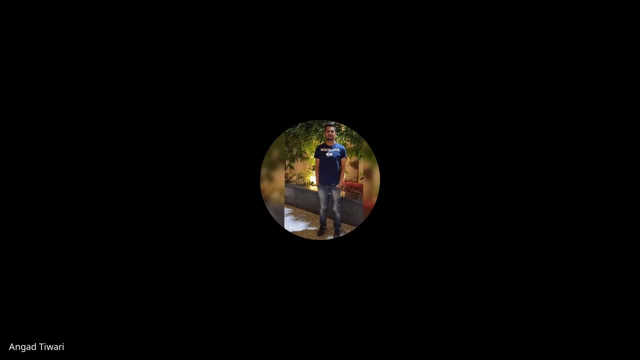 question uh, regarding the uh memory polyurethane that that is being used for the endovascular uh vascular embolization. uh, i've just uh. i just want to question what, what, what actually happens if the aneurysm uh eventually burst? so, since i believe the kind of material which is being used, 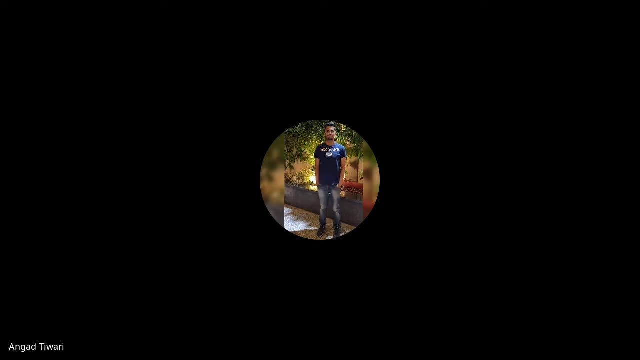 for these procedures are biological, non-reactive. so let's say, if the aneurysm burst, so what? what actually happens? does it get eventually get absorbed in the body? does it stay there? and if it stays there, will it have any risk on the uh, on the um, the further embolism which can, which can? 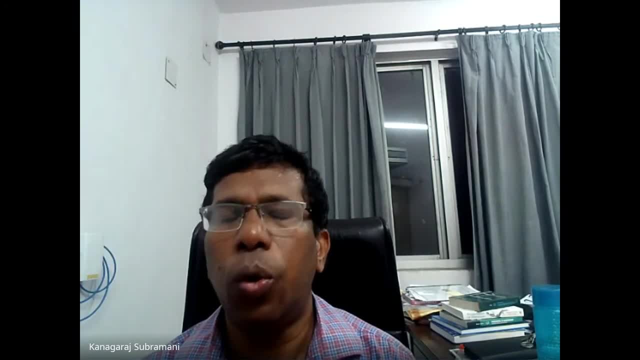 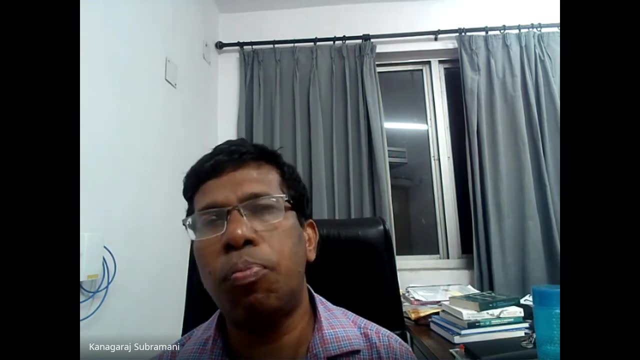 have another impacts actually, uh, thank you. actually we did that biological study. we confirmed that the biocompatibility, hemocompatibility and all like that and this polymer is not a degradable. okay. so if it is burst that uh, uh, mostly you will find that the brain, only that aneurysm and all it is a dangerous in other place, if at all, it's the birth. 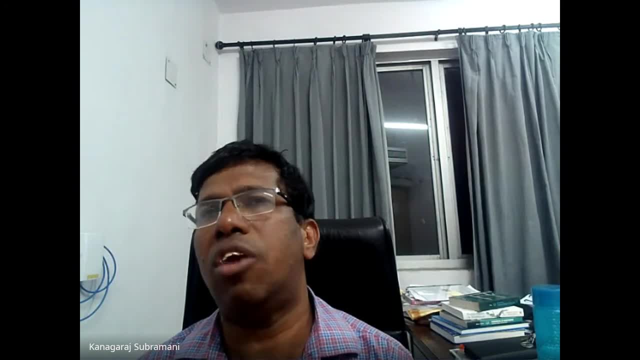 anyhow, the blood hemorrhage will be there and he will be treated, so during that time it can be removed, as it is not degradable, as it is. having a radio pack material, you can identify the location of it, right. so so does that imply that this product has certain limitations? 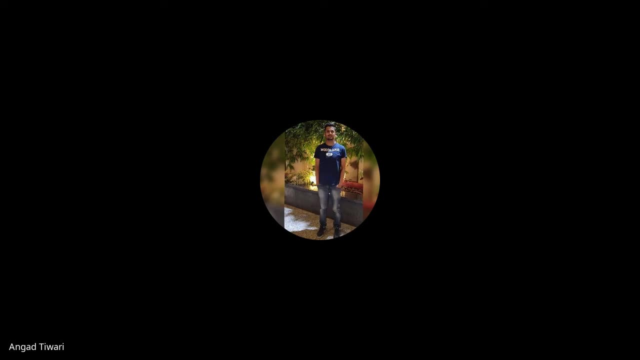 like you said, uh, if there is an aneurysm in the brain, uh, and, and the, let's say, the aneurysm, the brain eventually burst out. so, uh, will it have any implications? uh, any biological implications. even if you use that platinum coil, also, if it is burst, it is going to go with that pressure, it is. 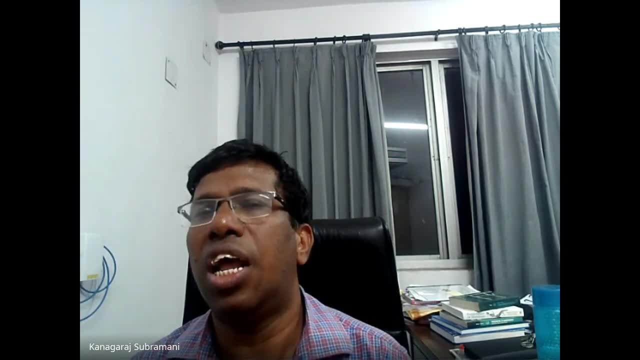 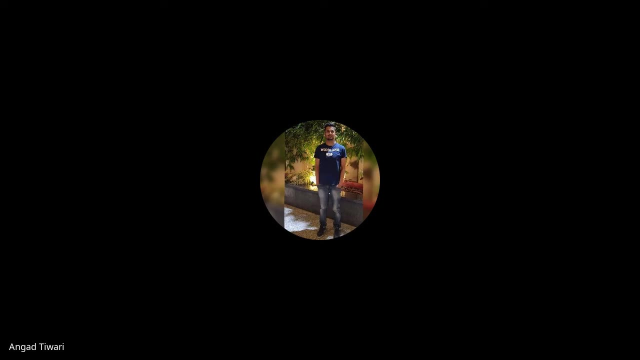 soft tissue also, it is going to damage the soft tissue. so the same thing: that impact will not be there because that is the metal and this is the polymer, so that the impact force will not be that much. uh, what eventually happened to it? like the aneurysm has already burst out in materials. it 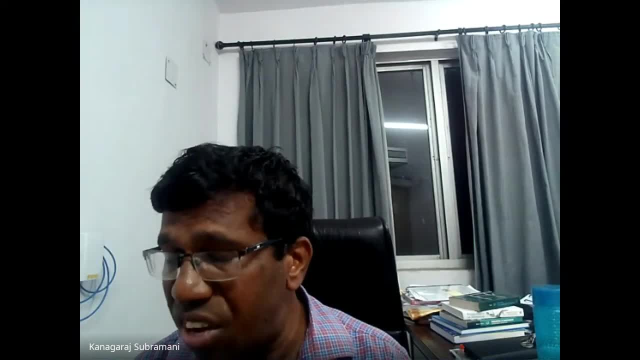 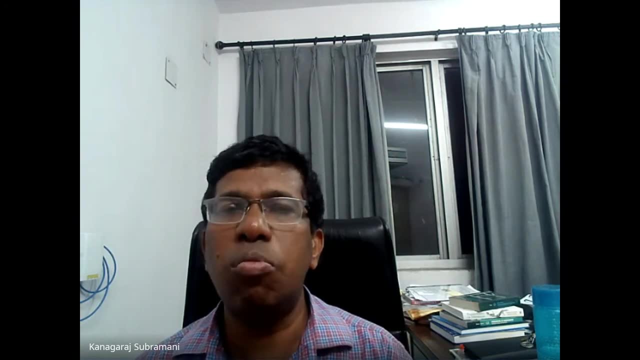 is in the contact with the body, so it will not have any issue. that is what we did: the biocompatibility, hemocompatibility test and all we did it, and it is very good and once it is burst out we have. till now we didn't think about it, but as we already completed that, 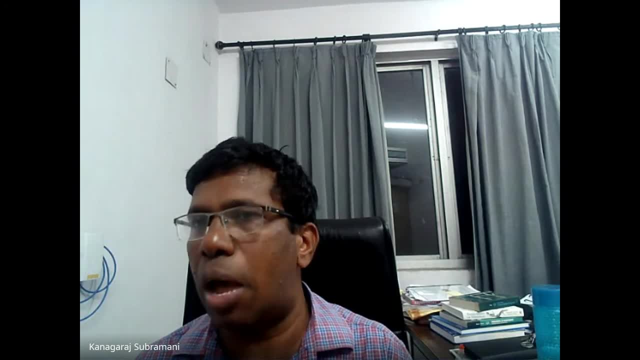 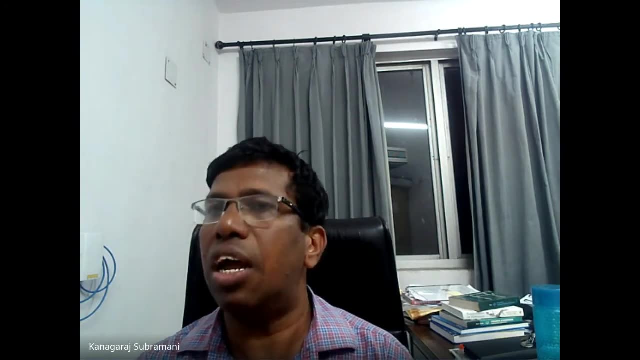 hemocompatibility, biocompatibility study and all nothing happened. nothing has happened, okay, on the tissue and all like that, and even animal study also we did. but that in that context only. i am saying: hopefully nothing will happen. however, there may be some issue with the physical impact. that is 100 sure, right, sir? thank you, thank you. 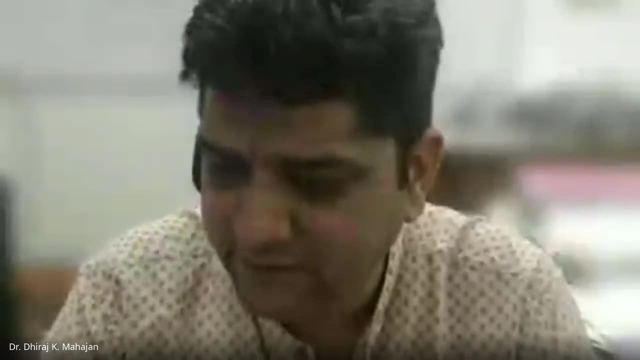 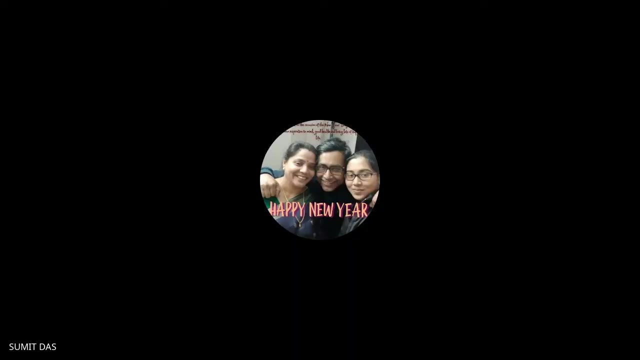 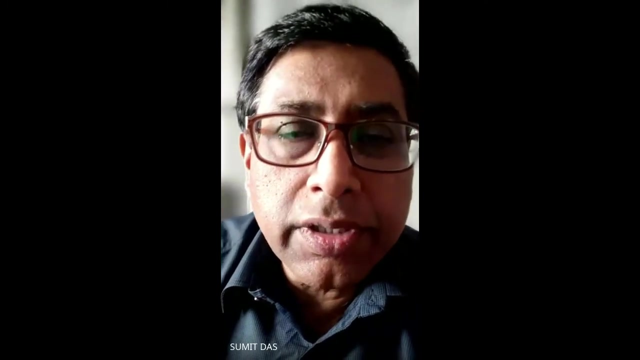 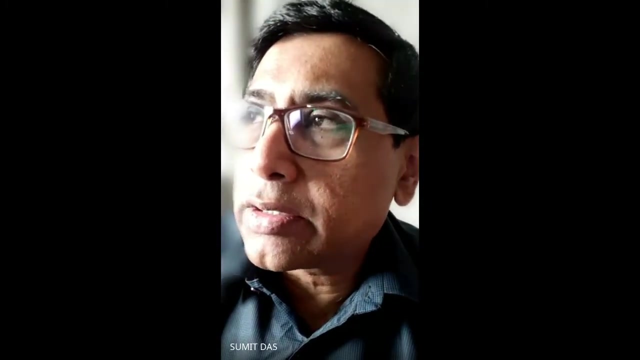 yeah, so that is very intensive discussion. so any other questions from anyone? so? so thank you, professor kanagraj. i just i was really impressed by the quality of questions from the cohort of students here. uh, very interesting uh. uh, just to just for my curiosity. uh, you know, when you said that there is a lot of uh fabrication involved, uh and customization, 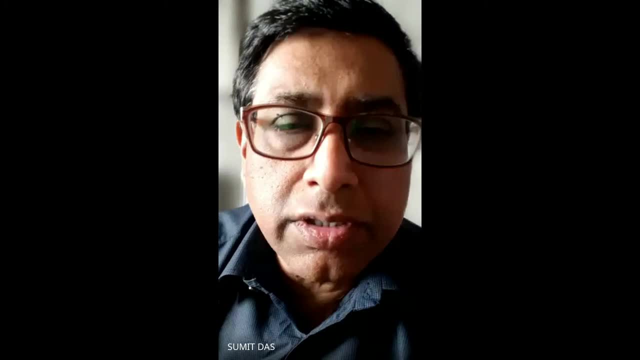 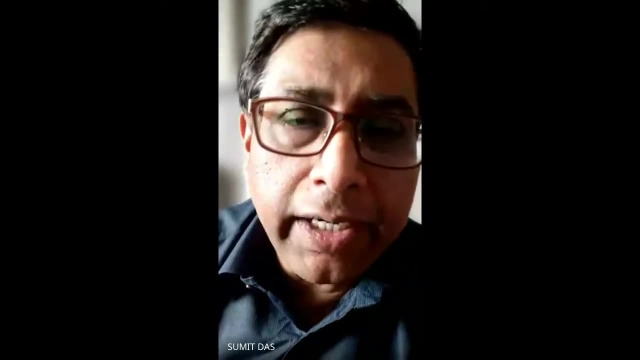 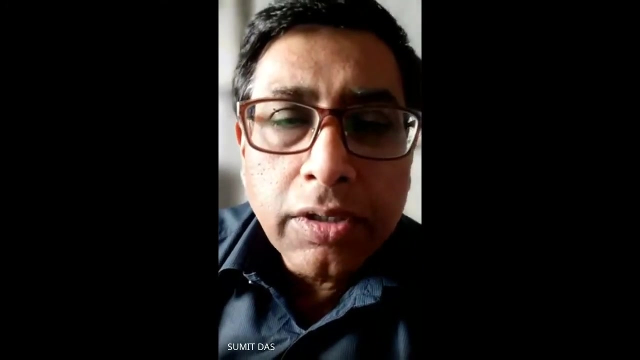 involved? uh, because it was each patient is different. uh, especially looking at this, yeah, so so how, how do you think the world of additive manufacturing? uh, because i think some of the questions that i think angad was asking regarding sweat and so on, so if you, if you adopt a additive manufacturing kind of approach, where you 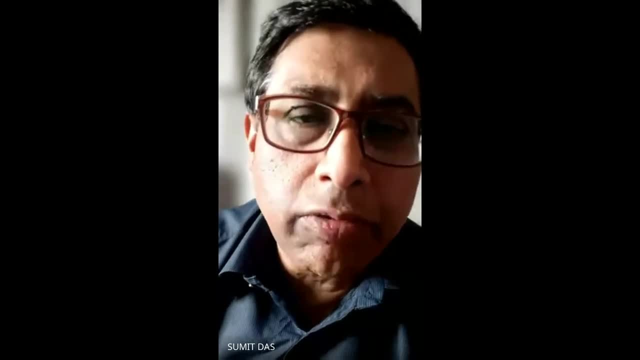 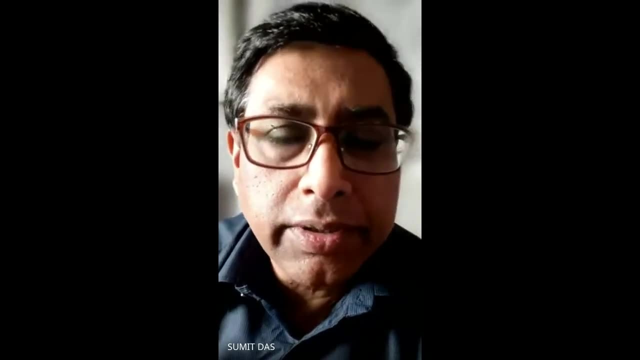 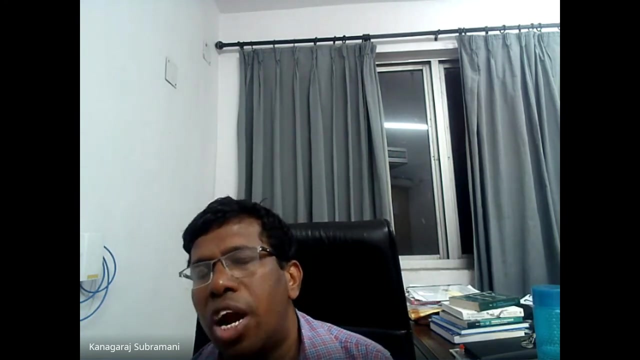 could have different kind of materials built one into the other. do you see that technology matured enough to be integrated with this kind of development? it could be possible, because that, whatever the socket needs to be made right now we are thinking about some kind of one-way wall. okay, so right now the fixing is 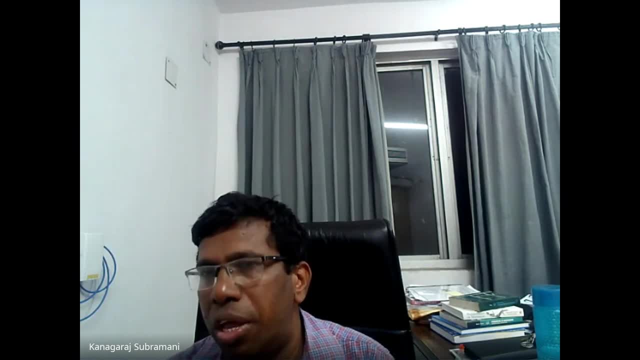 only the mechanical fixing, like a stocking at layer and ava. we are being. it is being used. in addition, the friction is not coming. friction is there okay. however, if you make that one-way wall due to the compression, if the pressure is released, vacuum is created that will hold it. 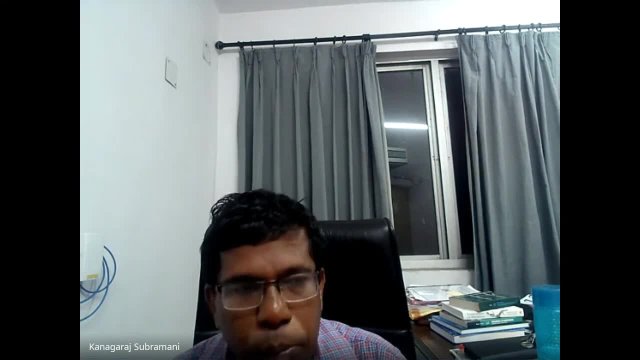 okay, that is what that clamping how we we can best we can clamp it okay. in addition, we have some holes and all like that, the breathable liners and all but uh, if we are going for a 3d printing and all like that, uh, i have bit reservation. i don't know, because we have not looked into that direction till now. 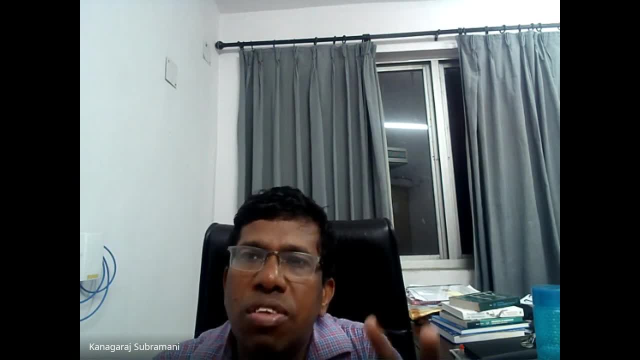 so the thing is that when you are making it, you may be generalizing something, because generally it will be mass production and all like that. when you are generalizing the material at that given time, if you are saying something there itself, the purpose is left. you have more people working. so we need to think of patience, specific kind of that time also. 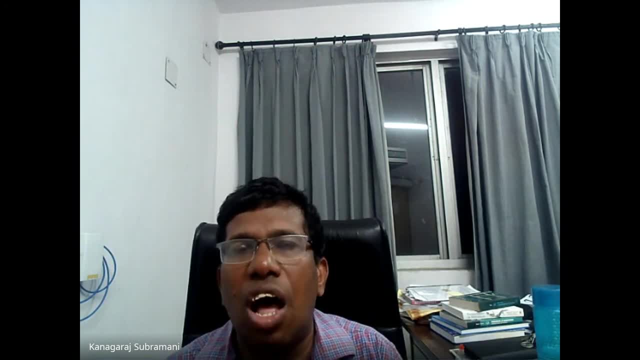 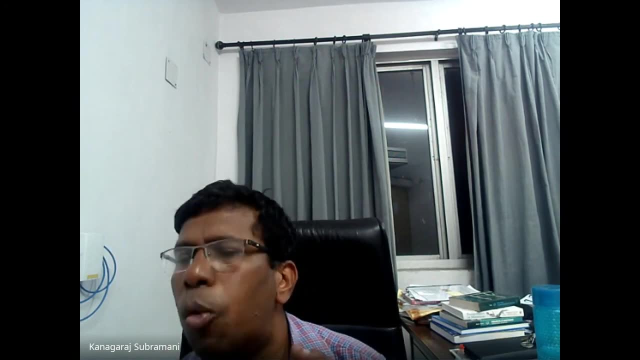 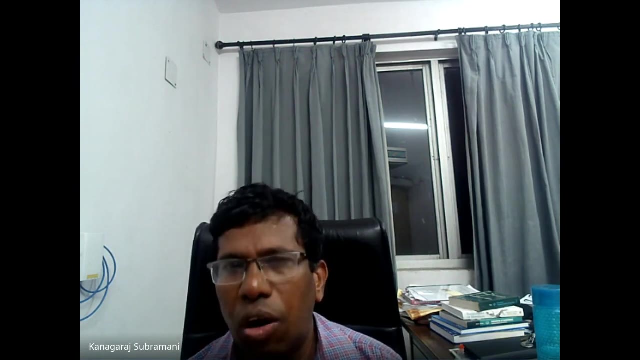 when? because at least 10 subjects you are collecting, it all, 10 are different sockets, fracture of fracture and the bone prominence, because mostly the issue comes with a bony prominence that we cannot generalize where it will be falling. okay, so because we should not say, being from engineering side, we cannot say nothing. 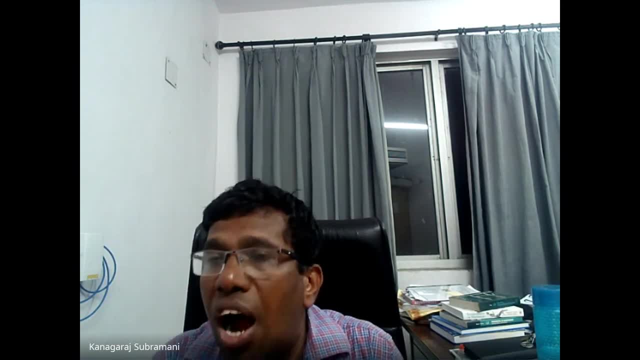 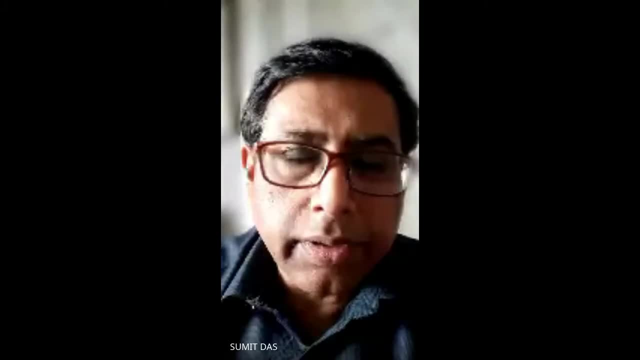 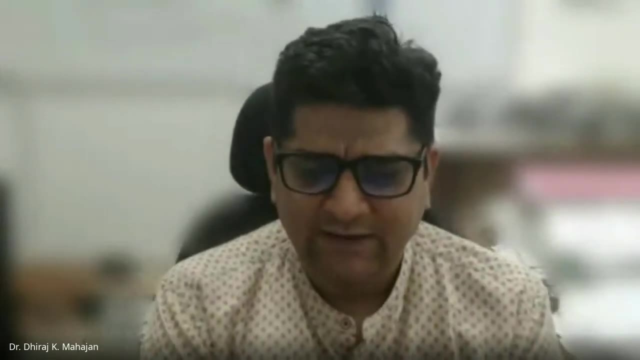 is possible. it is possible. however, we need to do a lot of iterations and we need to come with a plan. we need to do a lot of study. yeah, okay, thanks, doc, thank you, thank you. so I also have one question: that in in the implant, the hip. 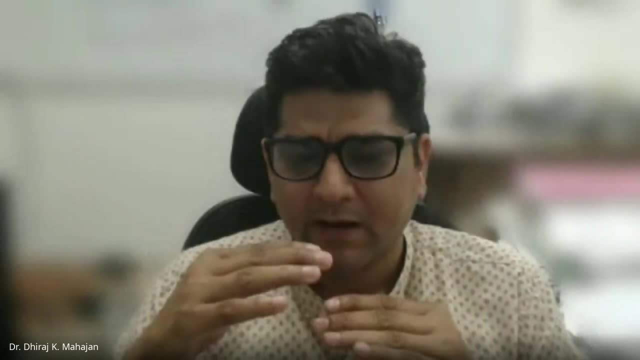 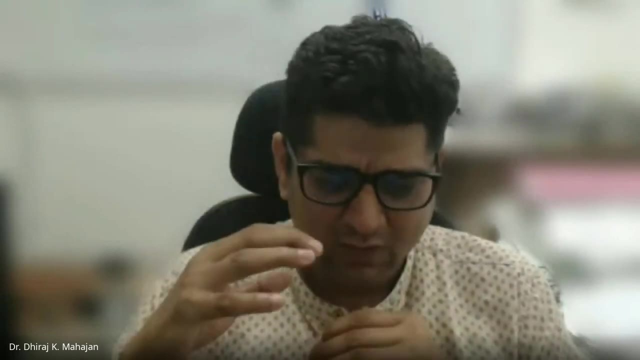 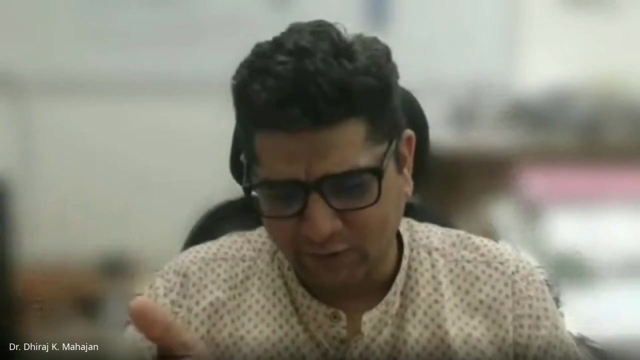 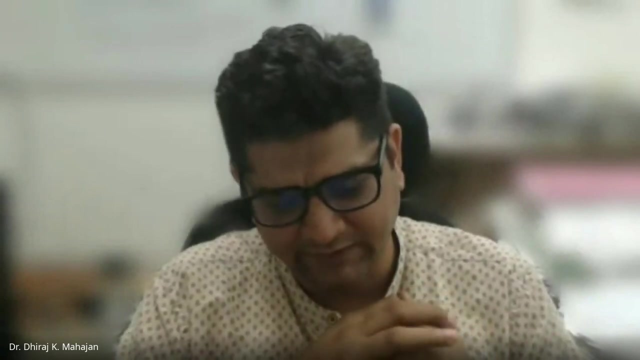 implant you are. you are basically the polymer. the HDP is in touch with metallic material. so so how does this addition sustain? like, for example, we are also doing some some hydrogen, high pressure, hydrogen storage cylinder development there also this metal and polymer addition is coming up as a problem, do you? 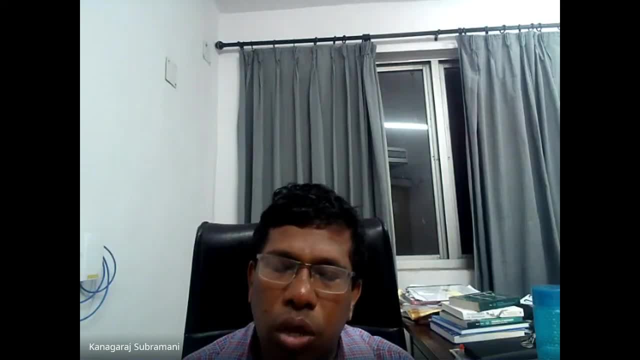 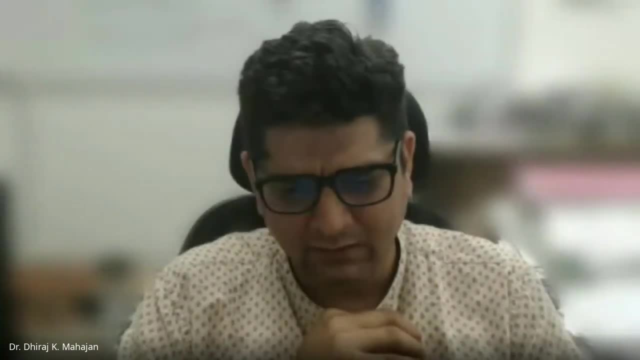 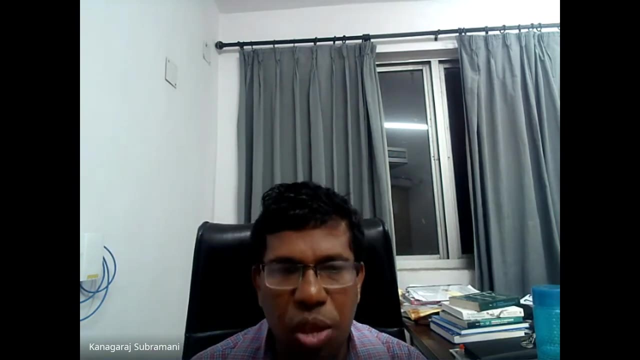 see some shearing issues. okay, thank you. in a normal case they are mechanically interlocked due to roughness or mechanical groove will be there in the metallic backup- okay. and in the polymer also. whatever we made it outer periphery is smooth, okay. in practical case it will. 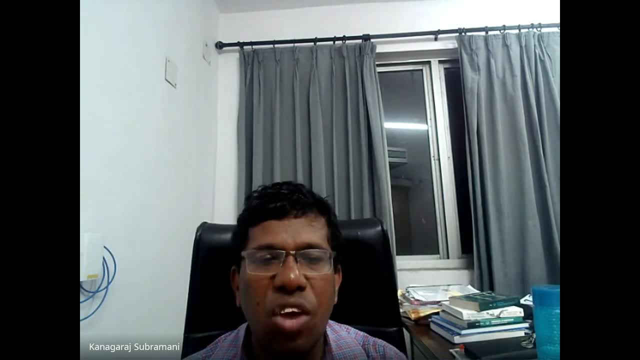 not be that. it will be having a lot of grooves. that will be exactly fitting with the metallic backup which is going to be fixed in the pelvis. it will be interlocked in such a way that what you can say, nothing is damaged. okay is only with the mechanical interlocking. 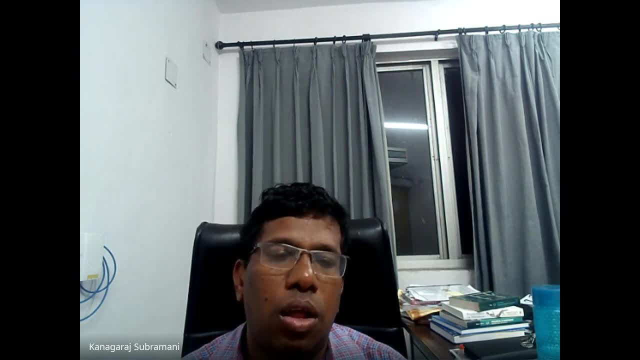 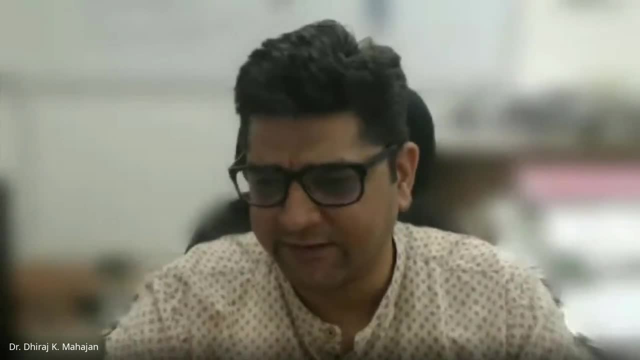 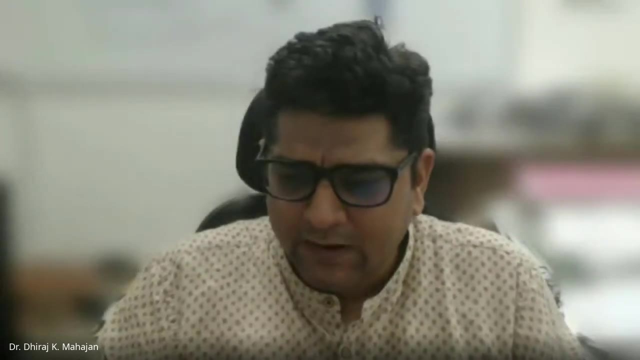 there's no other fixing technique. okay, thank you. thank you, yeah, um, yeah, so, uh, sir, I think it's it's a wonderful talk from the second garage and, uh, I think, student really had a very fruitful discussion with you. uh, with this, I I would invite uh Dr sumites to give his closing remarks. 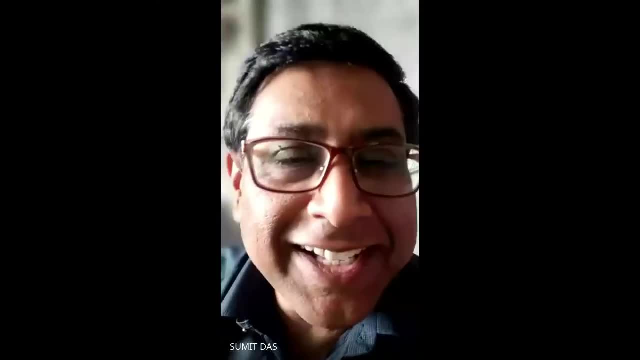 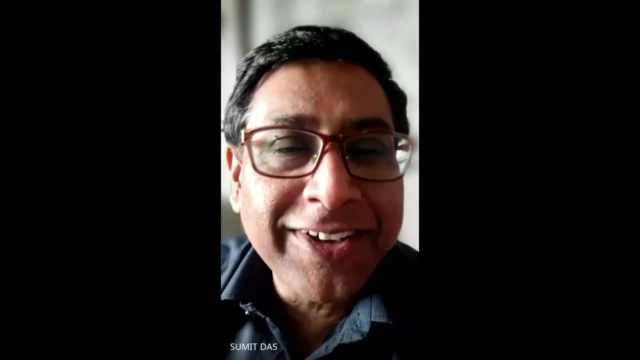 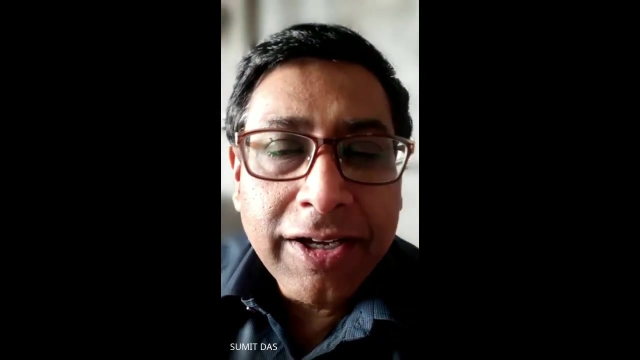 com, no, so so what else can I say? so? uh, I think I know Dr Kanakraj for almost like 10 years and I think he or more than 10 years now, doc, he has always been very passionate about bio implants and uh, prosthetics and so on and uh, I would definitely request any of the students who 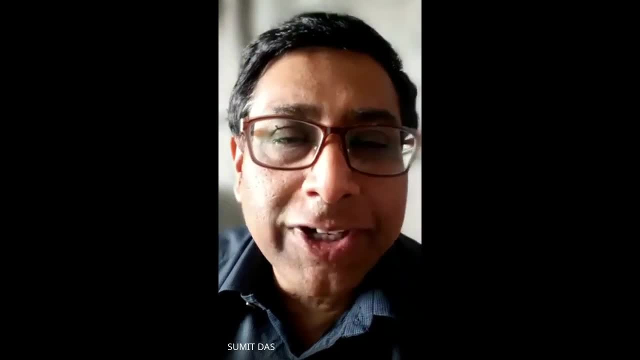 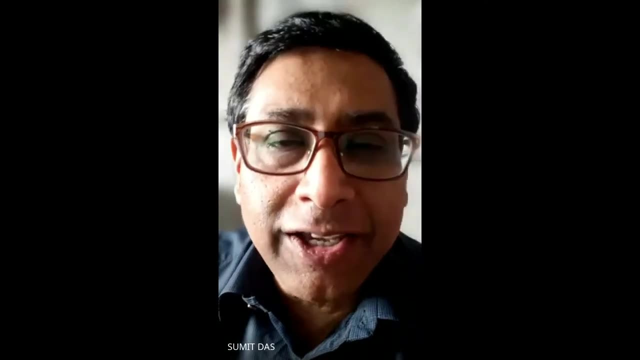 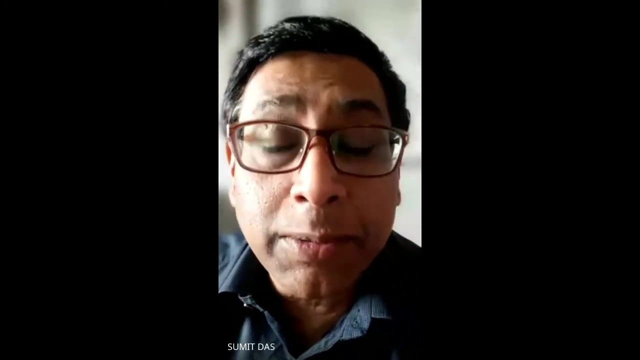 are going to that part of the country, uh, on behalf of Dr kanagraj and iit Guwahati, to definitely visit his lab. he loves to show his uh, his contribution, and I think he- I think since the first day I met him, he always has this thing of doing something good for the society. 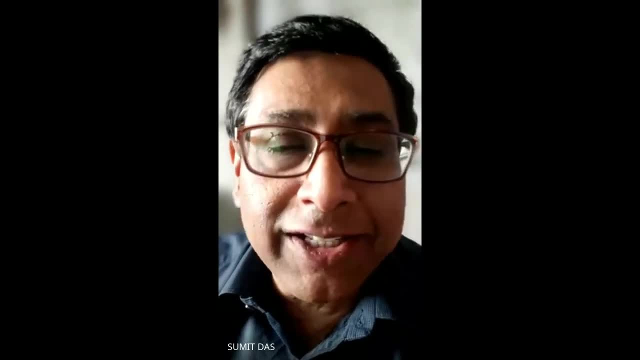 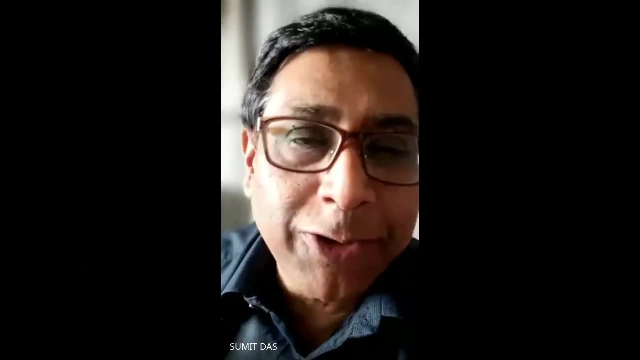 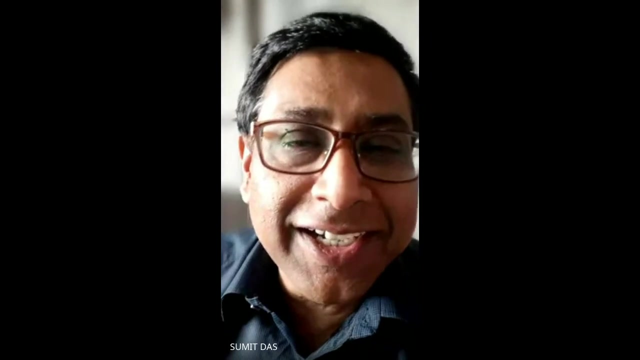 I think that's why, irrespective of the fact that we might have just worked for almost like three years on some project from some government of India, project on carbon nanotubes and so on- But we have kept in touch because of something or the other that he does for the social cause. 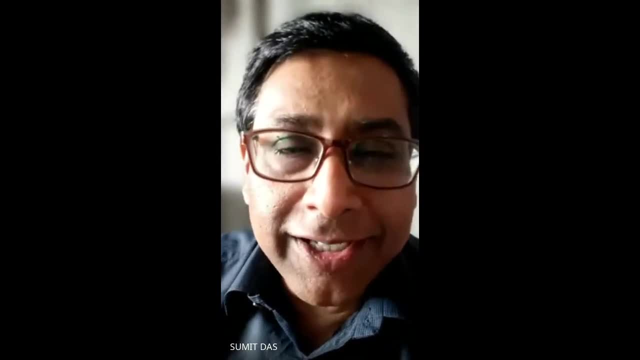 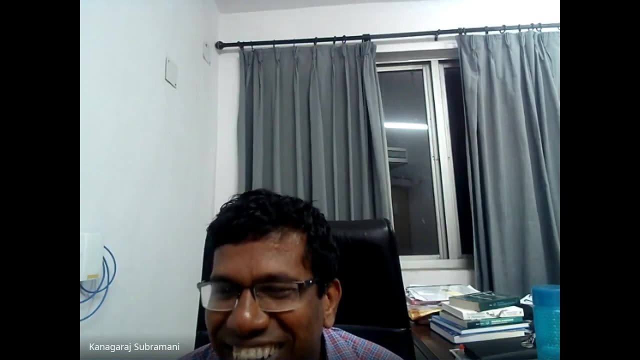 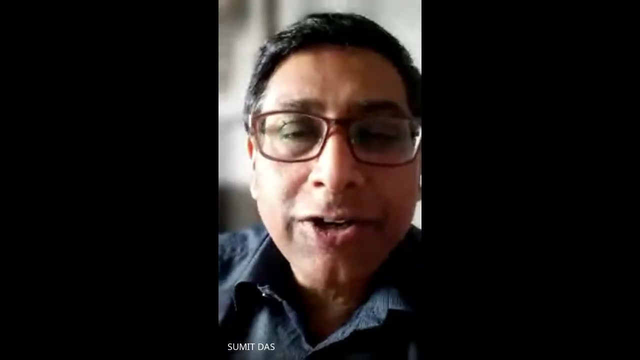 And so I think when we were looking for this course and a speaker, I think we couldn't get someone better than you. So thank you, Dr Agreed, And I'm sure you and your students, if they are interested, they can join this cohort that we have and they can add value from IIT Roper side and particularly from AidKriya. 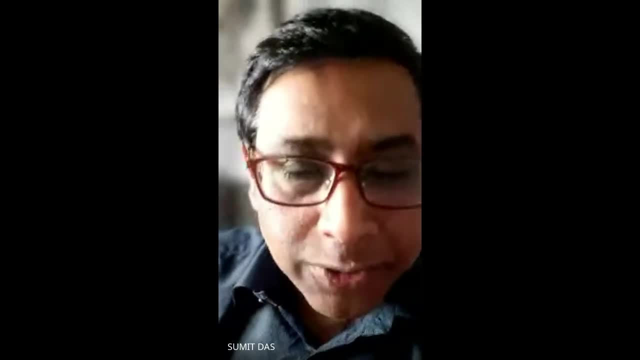 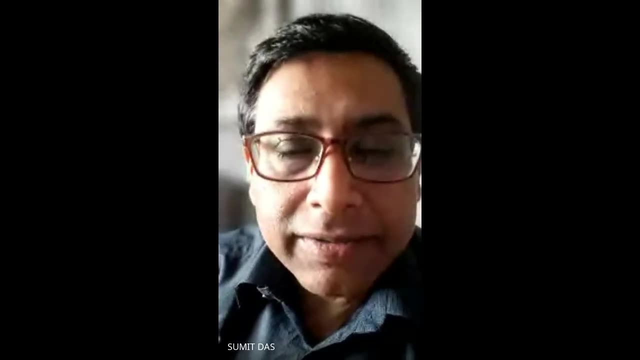 I think. Thank you, I don't know if Sujithesh is online. I'm not able to see Sujithesh. would you like to say something? Would you like to add something? No, not audible, sir. 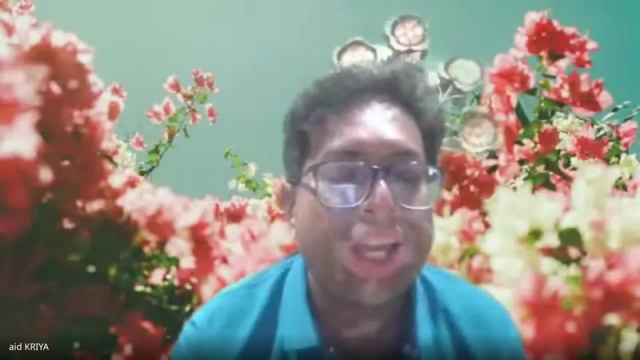 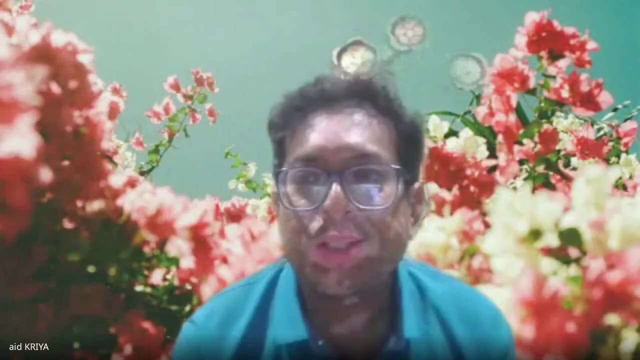 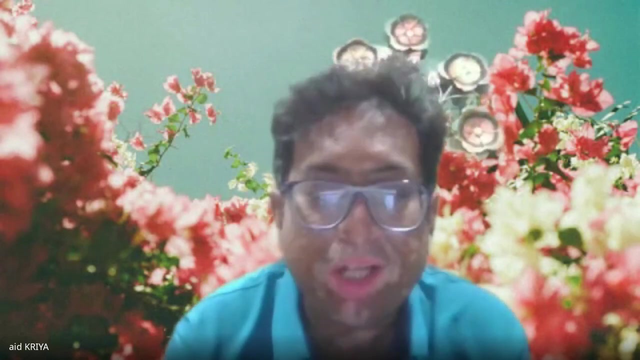 Sorry I was on mute. No, no, I think you and we spoke in February and we also looked at some collaborative effort specifically on some product lines that you know can be looked at it from the remodeled arthritis And we'd be happy to you know sponsor fellowship. 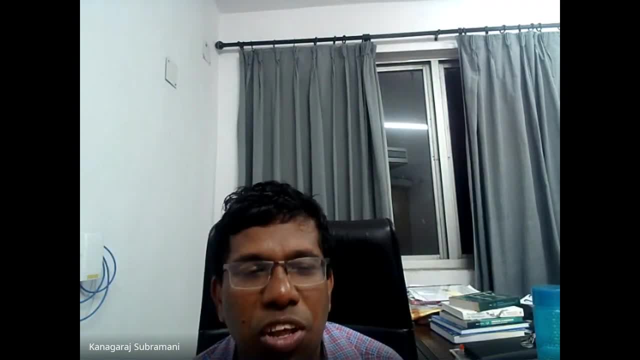 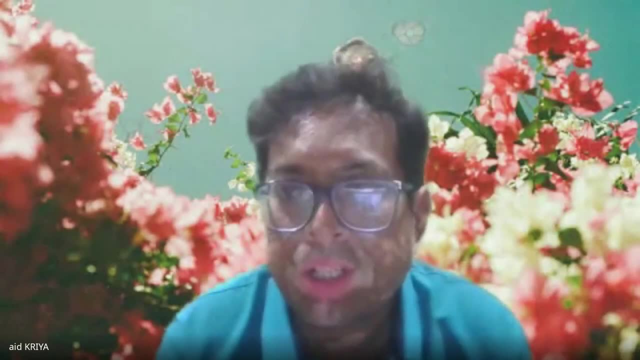 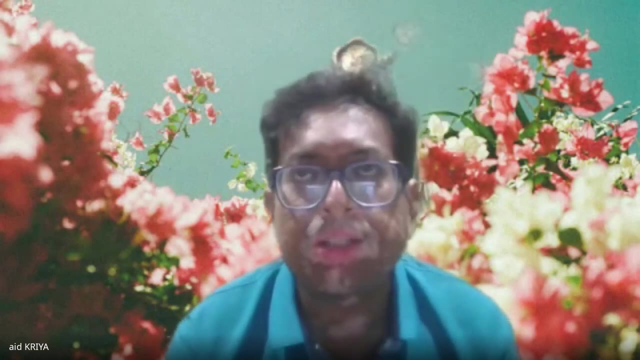 One of my students. he's a physiotherapist. He started to work on that, So we're looking forward to that And I'm sure that in some of the assignments projects that this ADUTH one will have, I think this is a you know, your lab and you and your team. 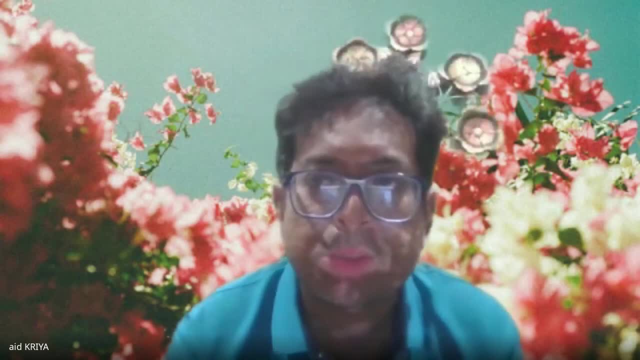 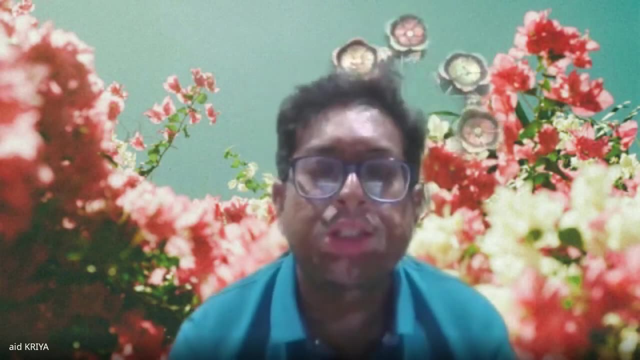 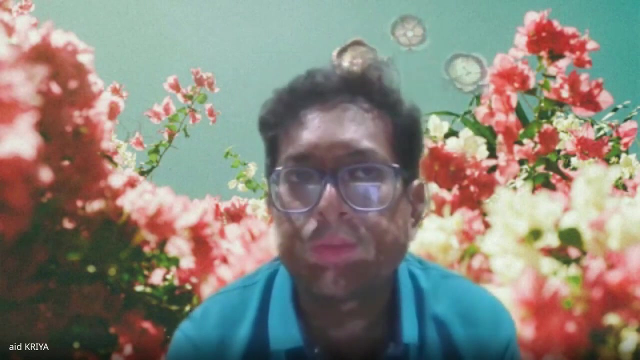 I think these are some of the good reference points. So I'm sure this presentation of yours- Already there is a recording. I think there's a lot of information so people can go through it And I'm sure they can take some reference points and cues to you know for their own projects. 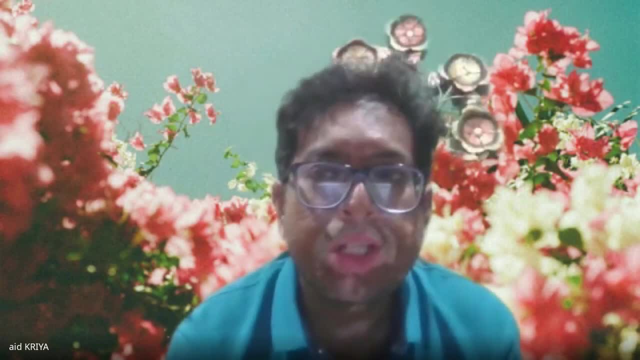 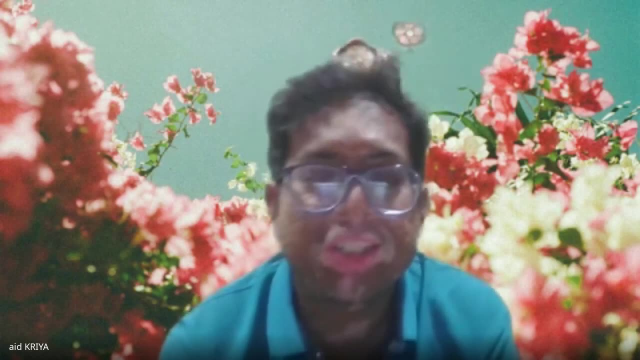 I'm looking forward- especially for, you know, a couple of students under your guidance from IIT Guwahati- to also participate and do some work for our foundation. So definitely. I know we talked about it on the summer time, So I think we are almost there.